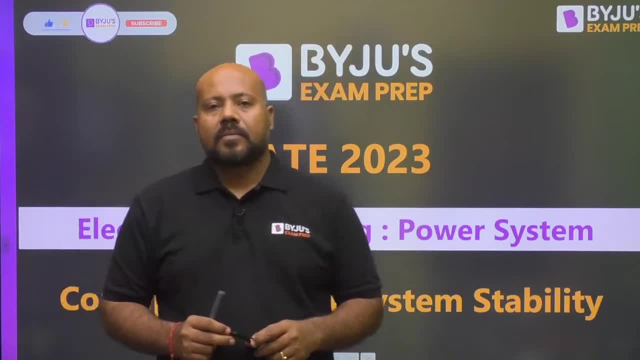 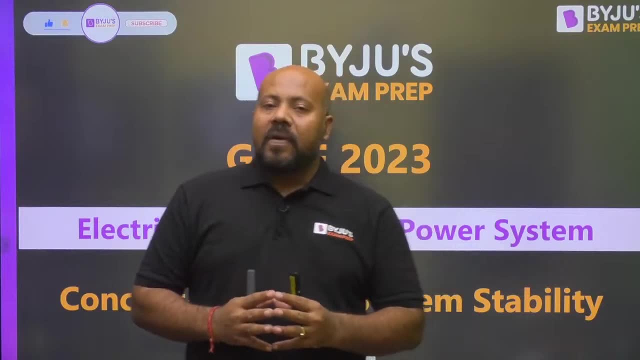 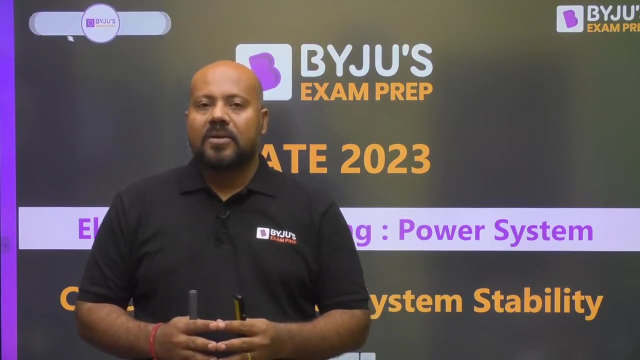 Hello friends, I welcome you on Baiju's exam prep, India's most comprehensive preparation platform for all the engineers, All the candidates who are joining me live. just quickly confirm your presence in the comment section and tell me whether my audio visual quality everything. 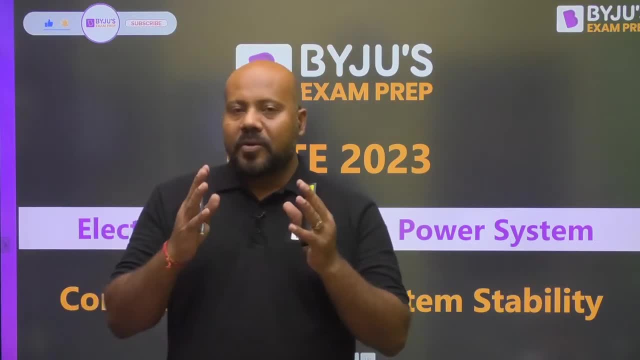 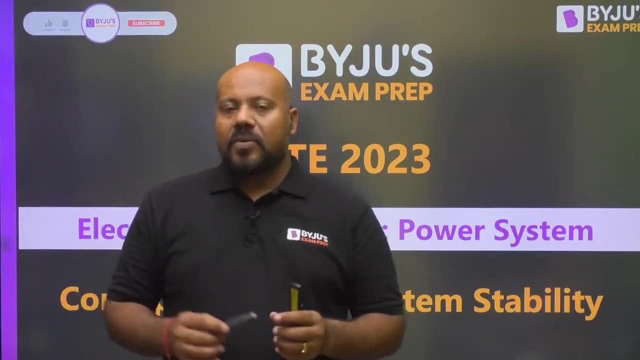 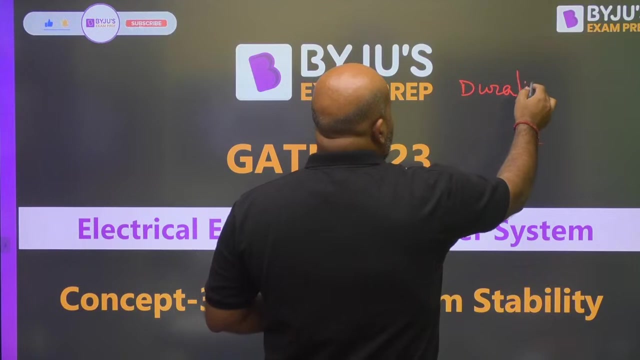 is clear so that we can start with the session. Till you are going to report me this, let me just brief you. what is the ideal duration and what is the agenda for today's session? Friends, the ideal duration for the session is going to be approximately 45 minutes, and 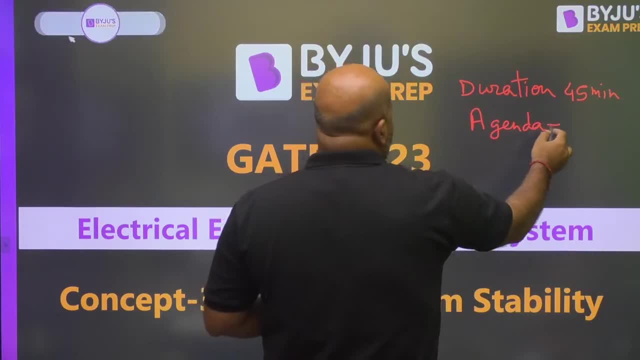 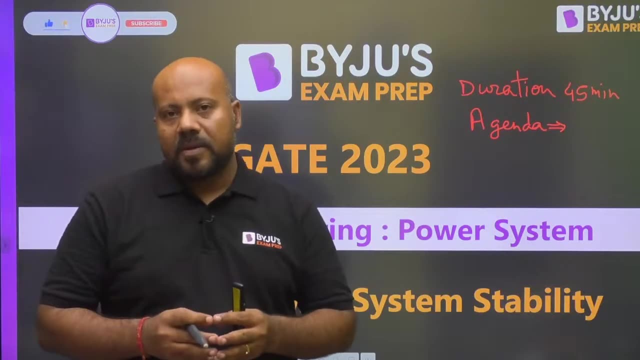 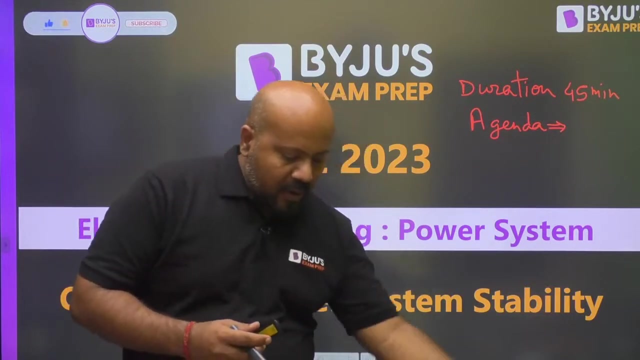 the agenda or the outcome of the session is that today we are going to talk about the third important concept for your subject: power system for your GATE 2023 examination. Today we are going to talk about power system stability. This is again one of the important. 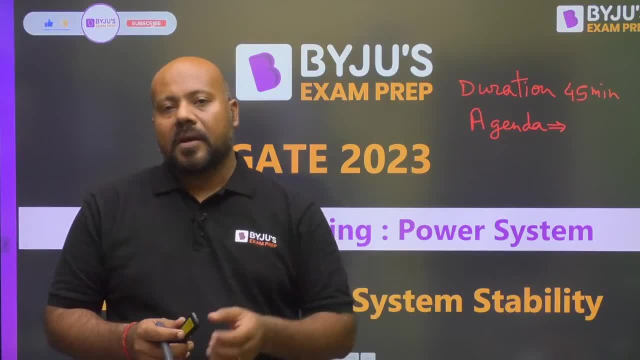 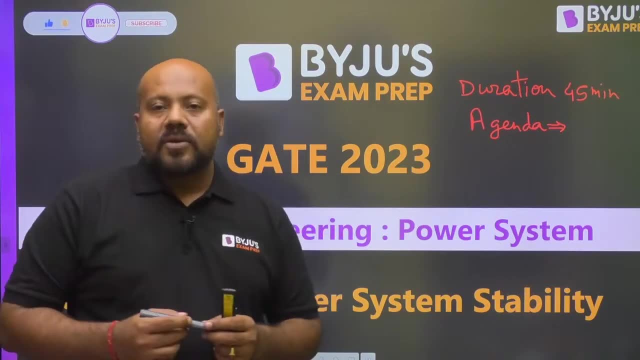 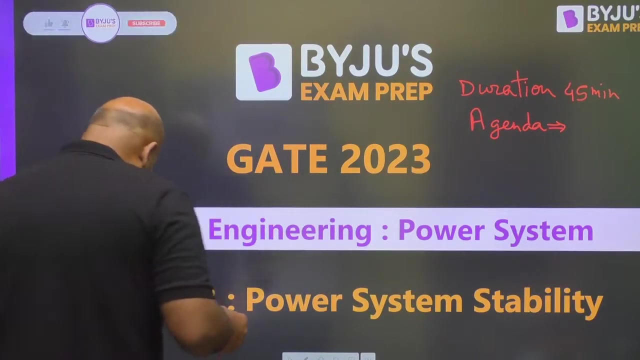 area from where you can see almost every year or alternate year questions are being asked. So everybody who is joining me live just quickly confirm your presence in the comment section so that we can proceed. Before we proceed, all the candidates, do not forget to like, share and subscribe the session so that more and more people are going to be. 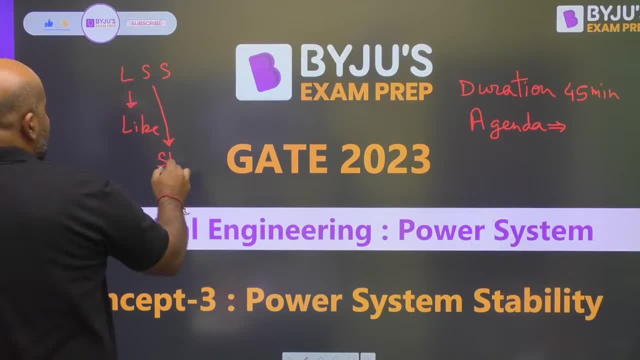 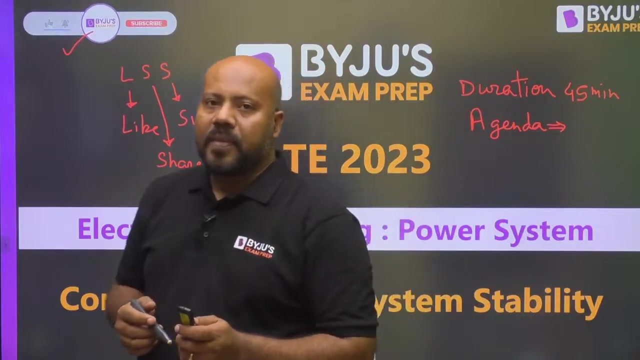 joining with us. Do not forget to subscribe Byju's Exam Prep so that you get all the important class notifications in time And hit the bell icon. this will keep you updated with the important sessions and its schedule. So let us start with the session. Some of you may be joining me for the first time. 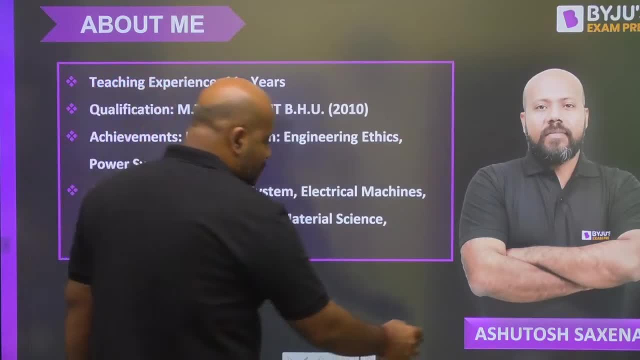 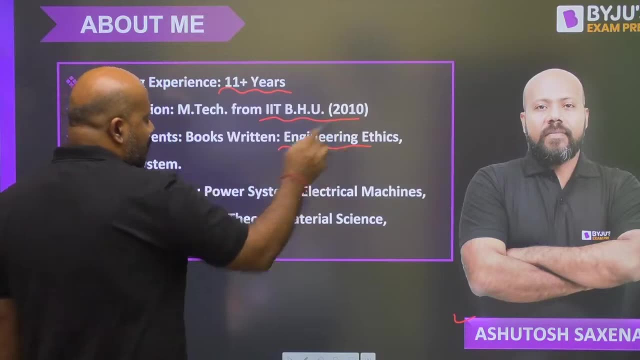 So there is a brief introduction about myself. My name is Ashutosh. as you can see on the screen, I have 11 plus years of teaching experience, completed MTech from ITBHO in 2010.. I have written couple of books on engineering ethics and power system, and these are my areas of expertise. 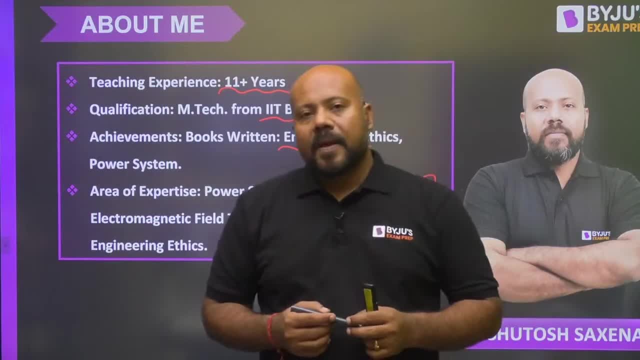 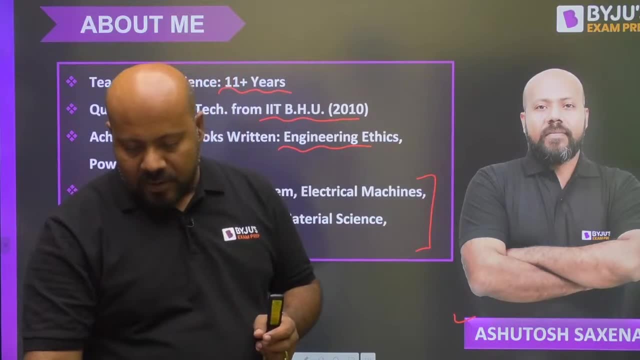 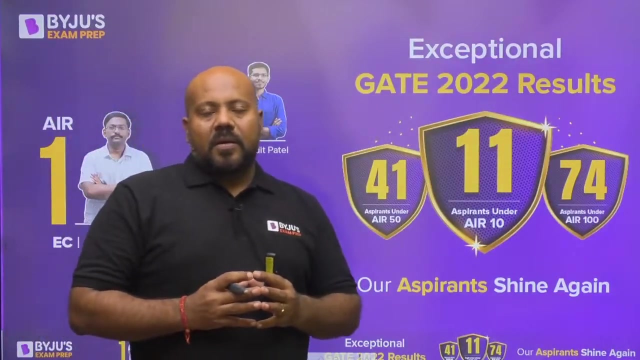 that is, power system, electrical machines, electromagnetic field theory, material science and obviously engineering ethics. so everybody who is joining me live, just quickly confirm your presence in the comment section. i'm not getting any response. just confirm, everything is okay. shall we proceed? before we start? a very proud statement. once again, byju's exam prep has 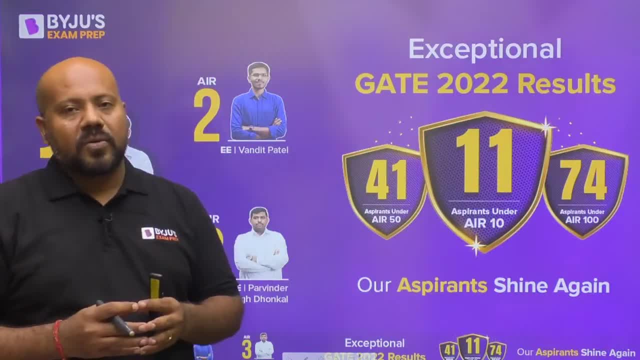 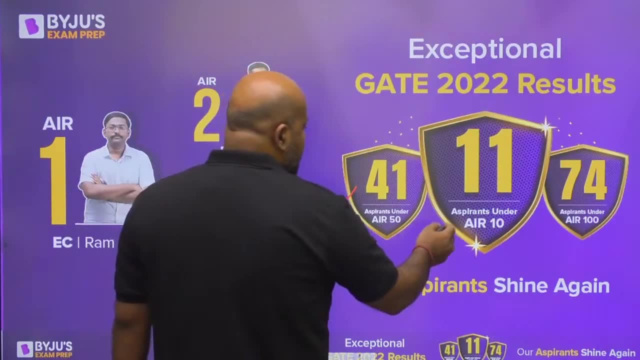 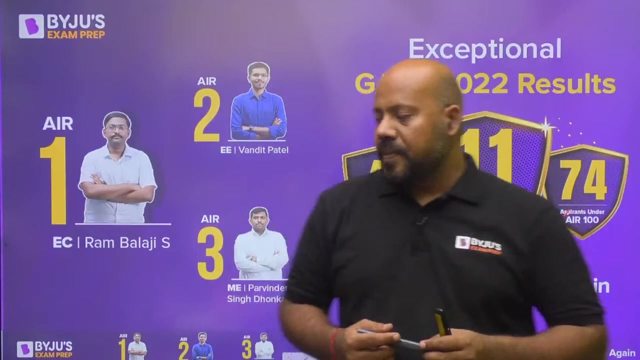 students has got exemplary result in gate 2022 examination. our students have got 41 students under rank 50, 11 students under rank 10 and 74 students under rank 100. some of the top rankers are rambalaji from electronics air 1. 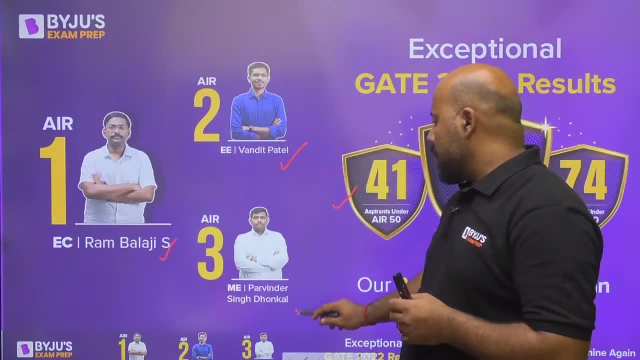 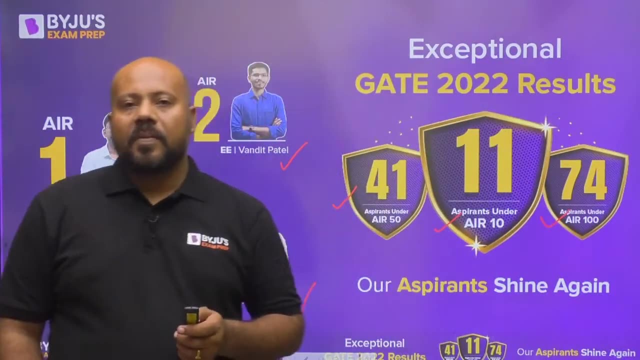 11 dh encontra. 1. bundit patel electrical ai r2 and. parvinder sink mechanical air 3. you can be the next one in this frame if- %HESITATION- you stay connected to byju's exam prep and you really work hard for your goals. 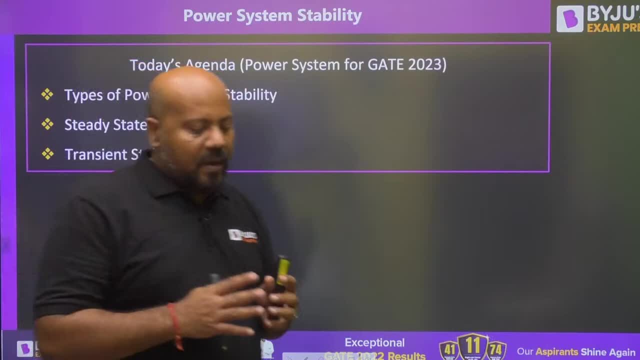 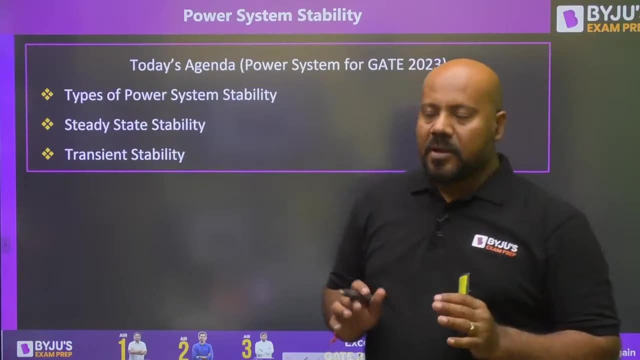 now let us try to understand what we are going to achieve in this particular session. what are the various concept or areas we are going to touch upon in today's session? the first thing we are going to talk about is the type of power system: stability. first, we'll understand. 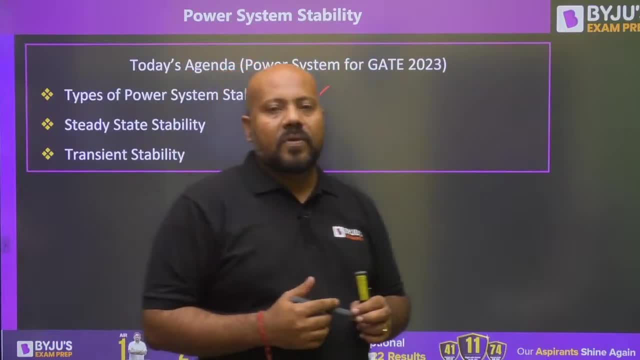 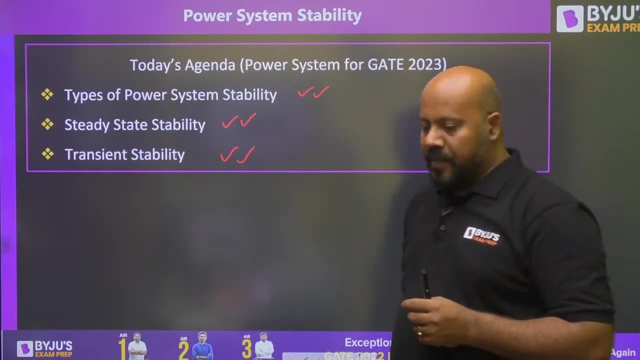 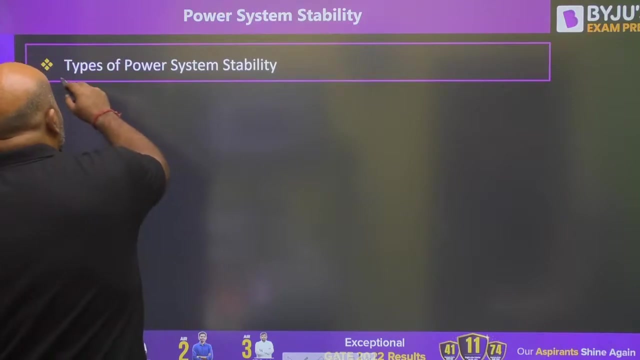 the various types of of power system stability, and then we are going to focus majorly on two types of stability, that is, steady state stability and transient stability. is it clear? everybody? shall we proceed now? let us start with the types of power system stability, but before that I want 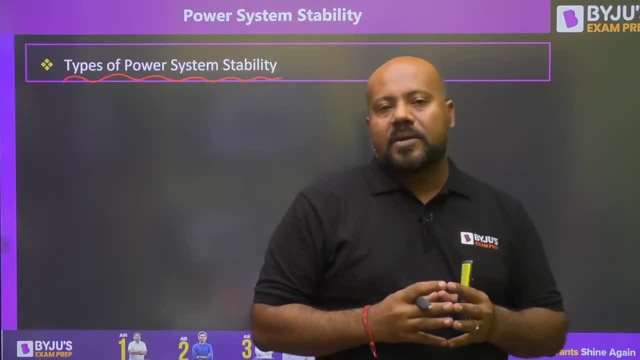 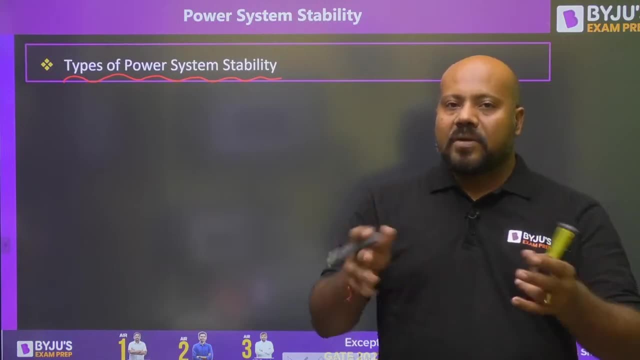 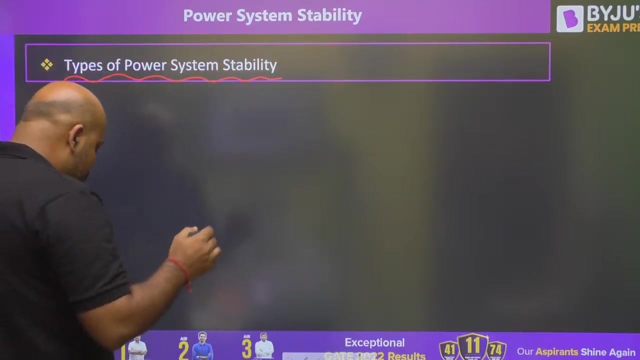 to give you a simple, practical understanding of what is stability is because if you understand stability well, then you will be able to understand power system stability also. tell me yes or no in the comment section. yes, everyone. so let us first understand what is stability. what is stability? let me just give you a very practical 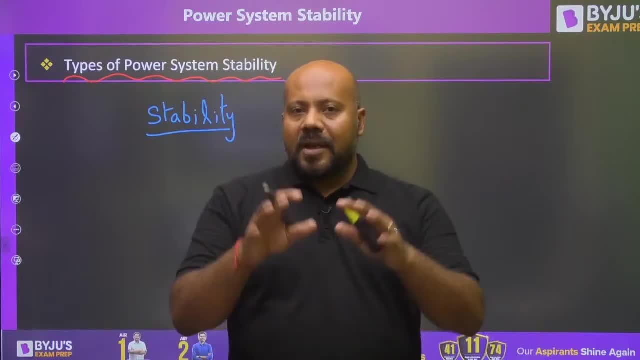 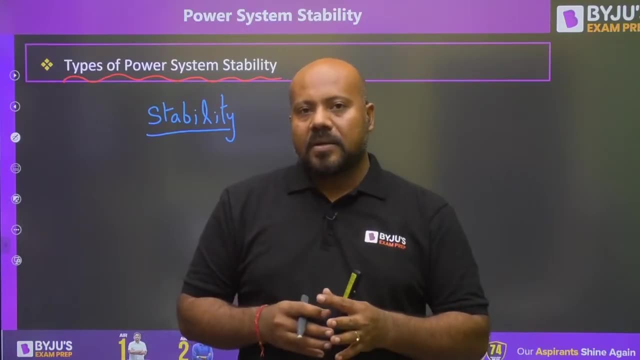 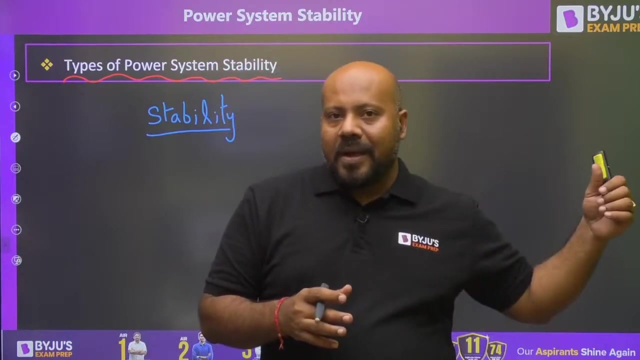 example, suppose there are some students in my class and I am standing here and I am leaning like this and there is a notorious student in the class and he is coming from this side and he is going to push me. now, if the moment he gives me a push, suppose I am leaning like this and I am able to. 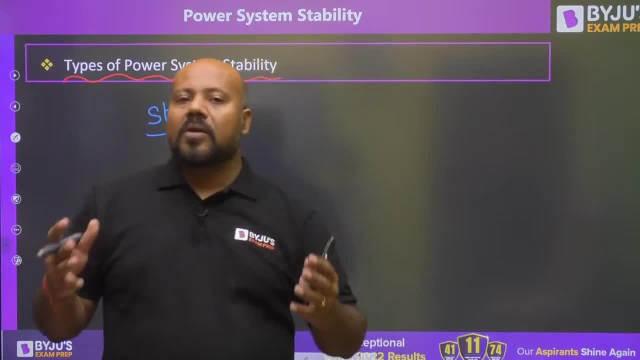 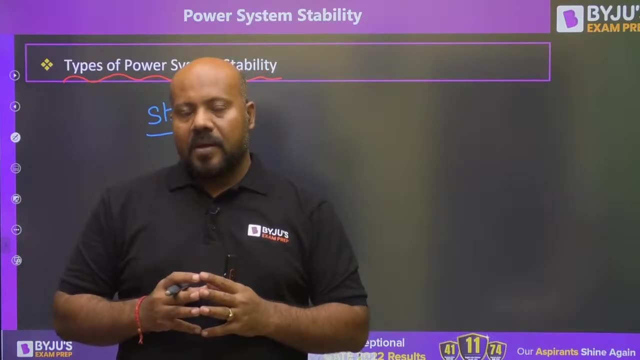 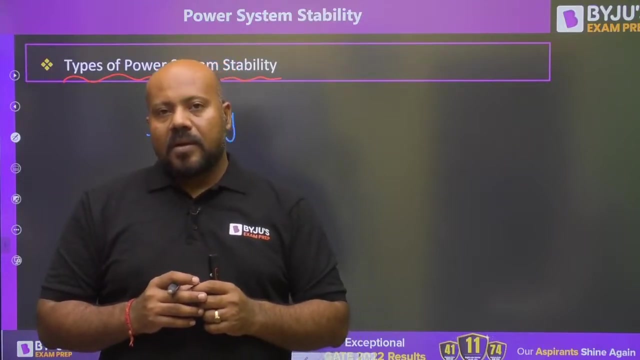 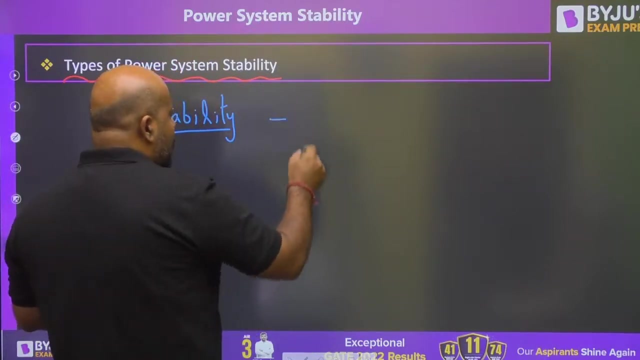 manage myself and I am going to attain in new equilibrium position. then the other candidates are going to say that Ashutosh sir is stable. now what are the two important things you have understood from this example? The first thing is, when you talk about stability, you have to talk. 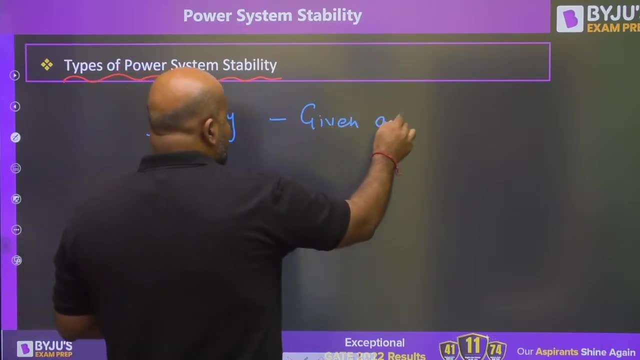 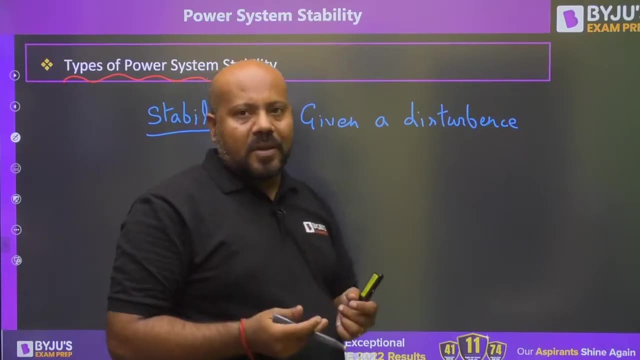 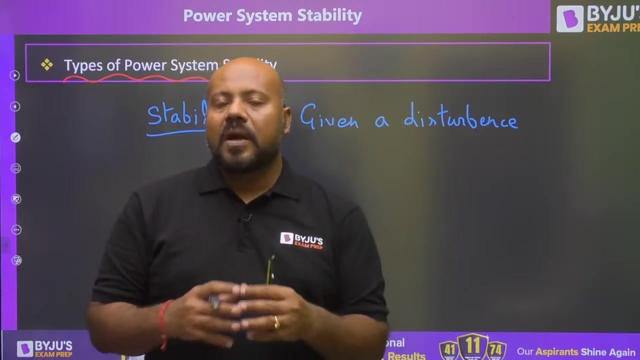 about a disturbance, given a disturbance. If you don't talk about the disturbance, if you don't talk about the change, then there is no meaning of stability, Yes or no. Without disturbance you cannot talk about stability. So the first thing is disturbance. What is? 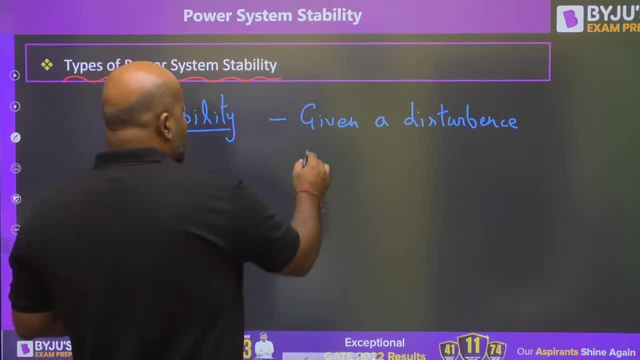 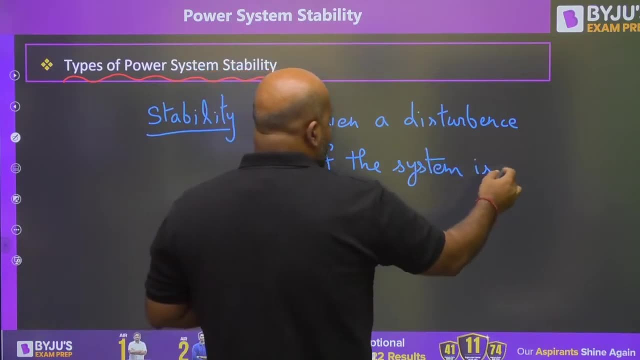 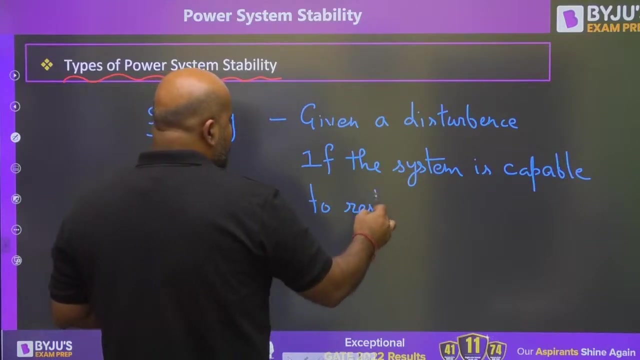 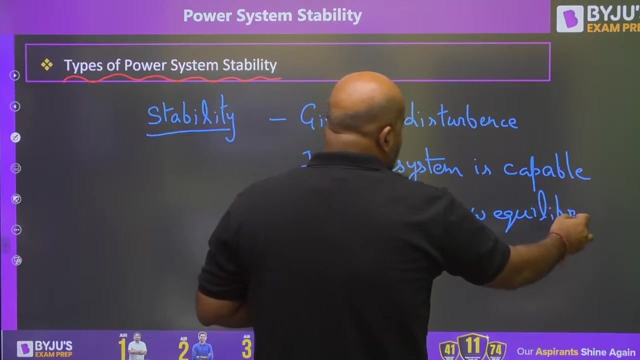 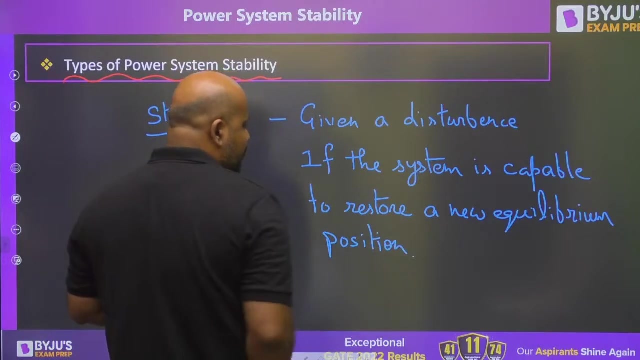 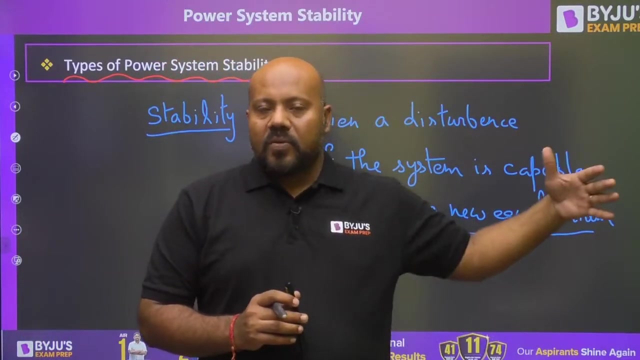 the second thing: Given a disturbance, if the system is capable to restore a new equilibrium position. Now why I am saying new equilibrium position? Let us try to understand. Why am I saying new equilibrium position? Suppose I am standing like this and the student who was the notorious 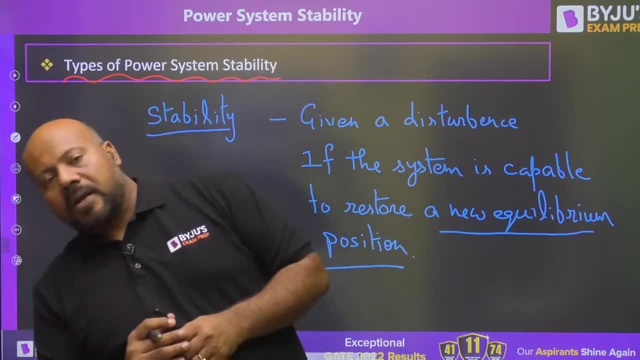 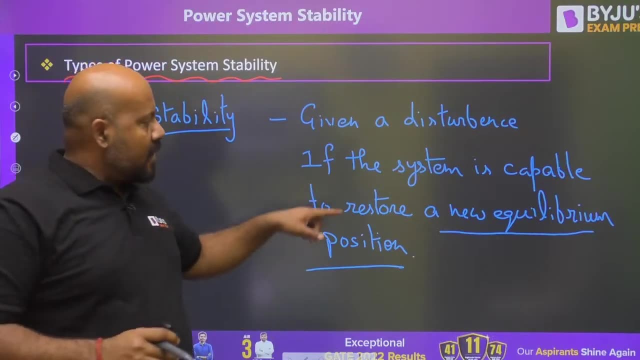 student. he gives me a push and suppose I lean like this and I manage myself. and now I am standing here, Now I am at the new equilibrium position. So now I am at the new equilibrium position, but again I have attained the equilibrium. 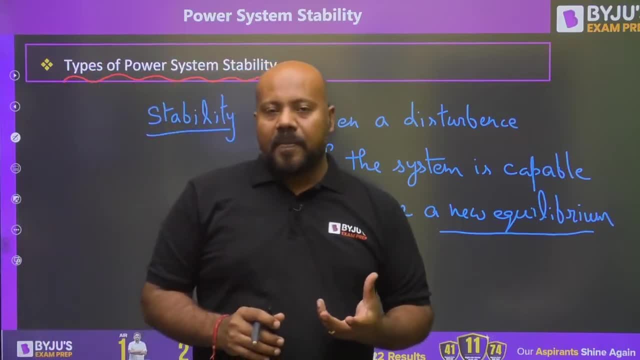 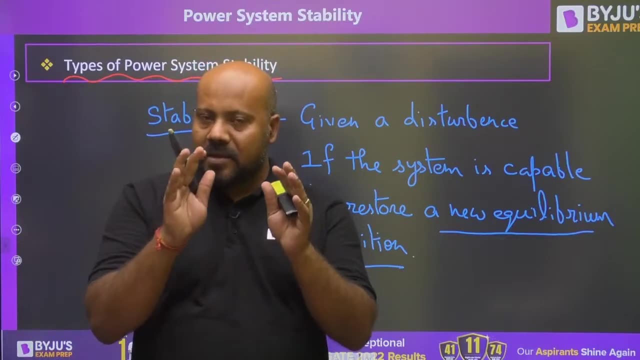 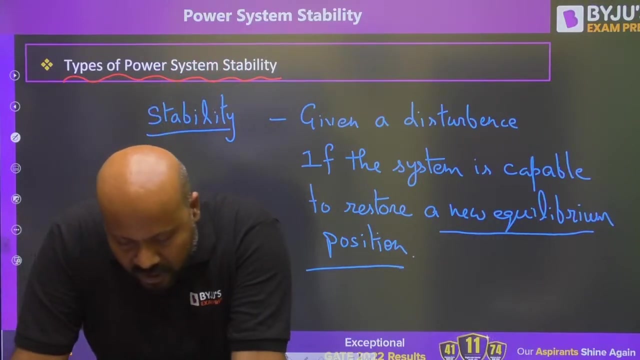 So if the system, any system, has this capability, that, given a disturbance, if that system is able to restore to a new equilibrium position, we are saying the system is a stable everybody. just tell me in the comment section: are you able to follow this, Manish Kumar Yadav, good. 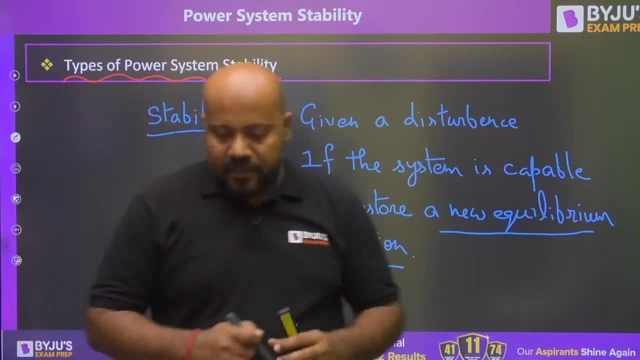 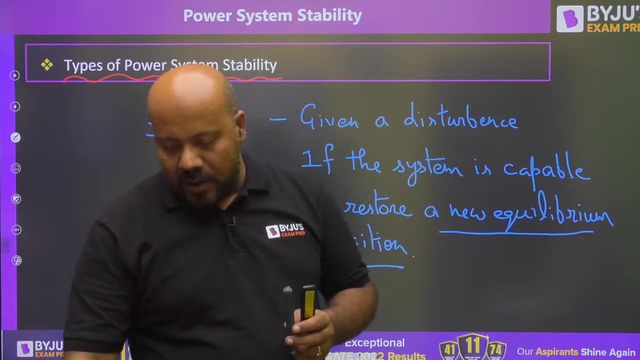 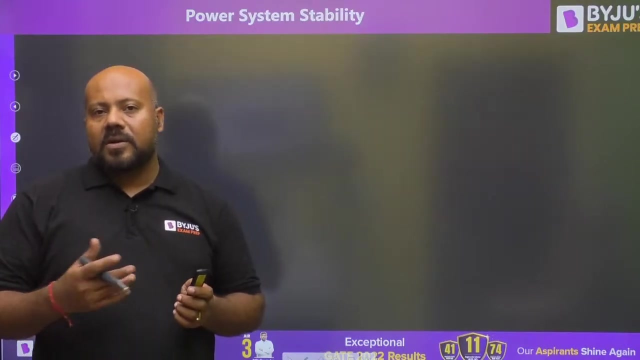 evening. how are you welcome to the session? so the first candidate who is commenting, everybody just tell me in the comment section: are you able to follow this? so if now you are comfortable with the concept of stability, let us try to understand various types of power system stability, if you 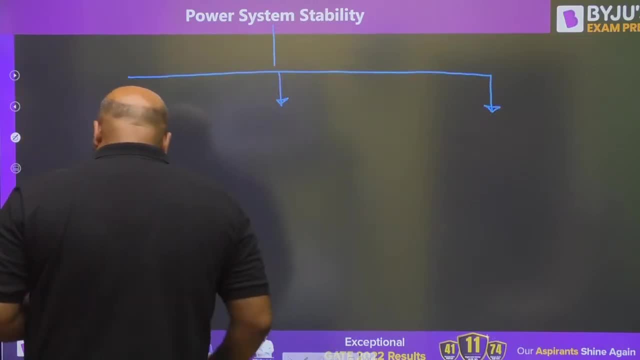 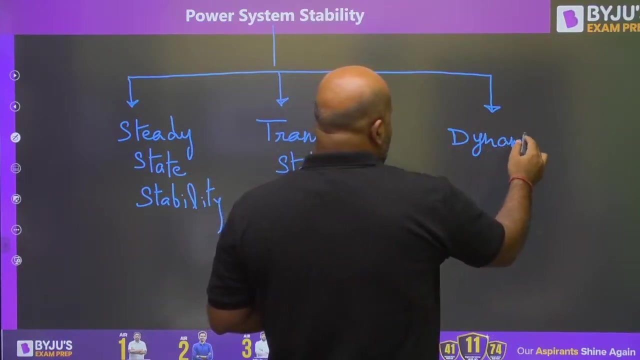 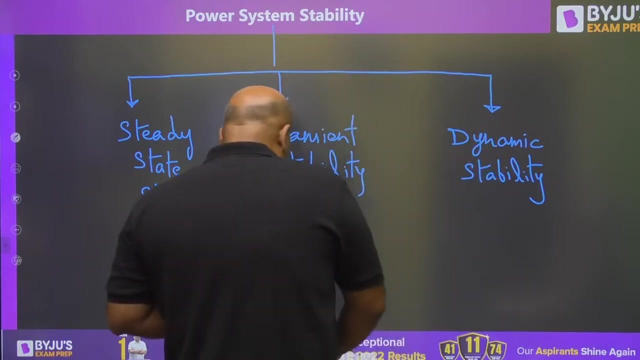 classify the power system stability. you can classify it under three heads. the first one is a steady state stability. you GD state is stability. the second one is transient stability. the second one is transient stability and the third one is dynamic stability. third one is dynamic stability. now let us first try to understand what is a steady state. stability will discuss. 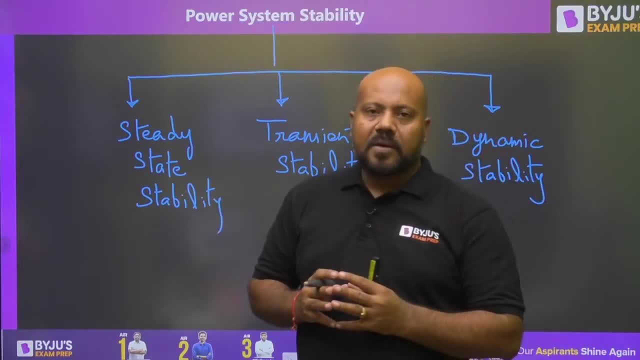 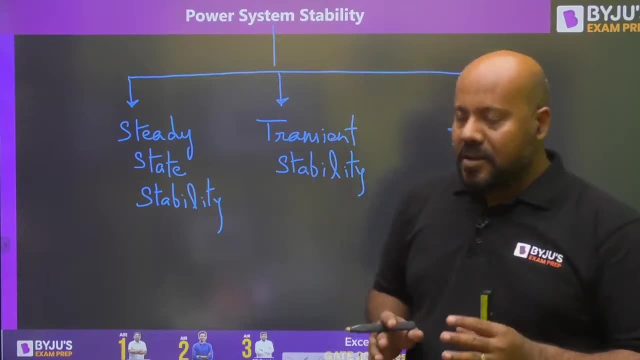 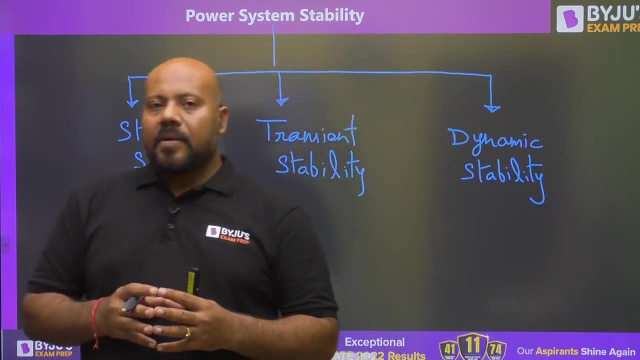 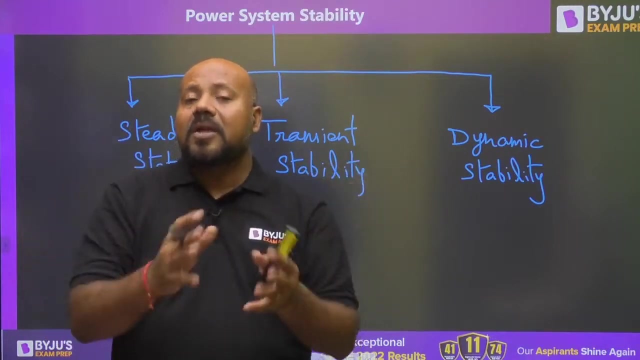 in some more detail, but let us have some brief introductory idea about these three different types of stability in one go. when you say steady state is stability, or transient stability or dynamic stability, we have three different types of the stability. stability is on the basis of three different types of 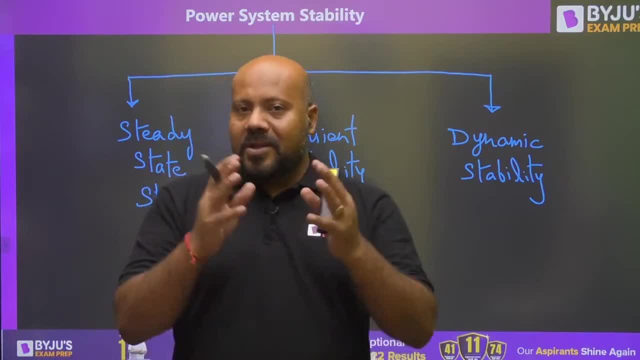 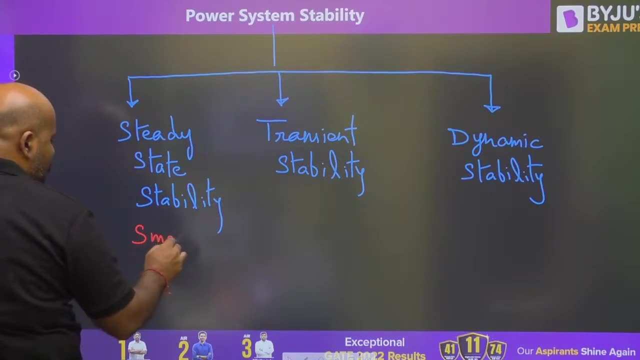 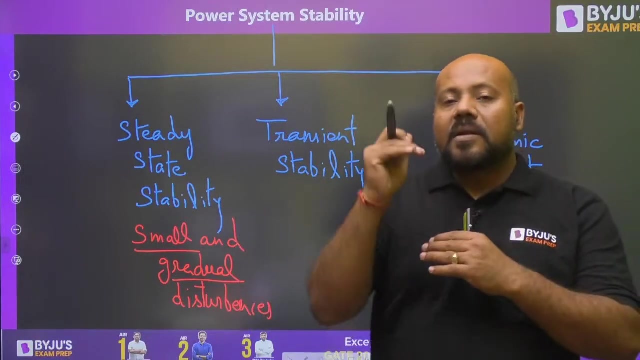 disturbances we can have in our solve for a steady-state stability. we are talking about a small and gradual changes or disturbances. changed means disturbances, you, you, us, all you. small and gradual. a small means the magnitude of change is small, and gradual means the rate of change is also very less. is it clear? everybody? just tell me in the comment section. 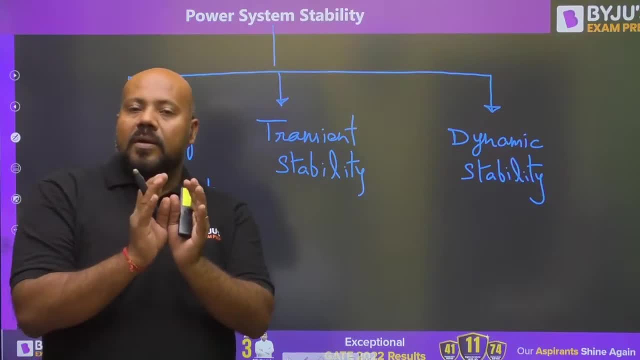 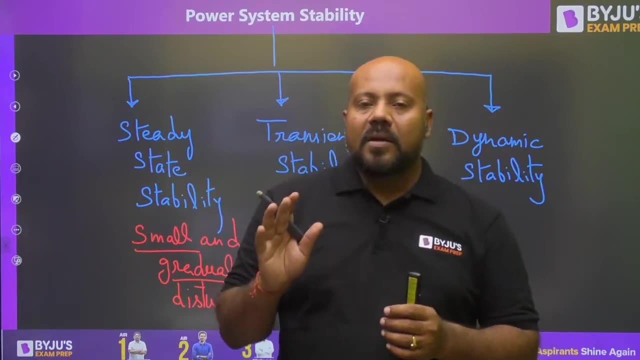 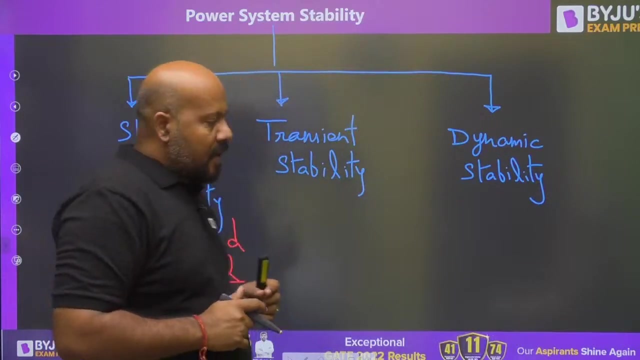 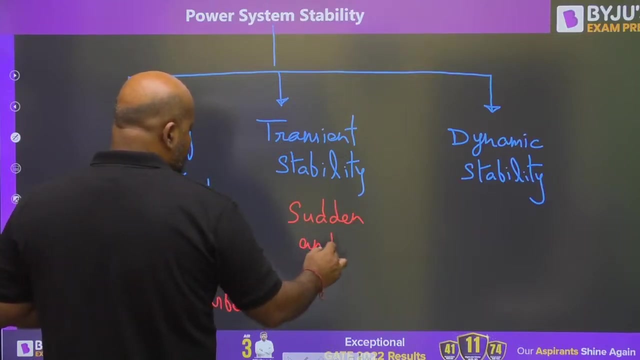 so when the given disturbance is small in magnitude and its rate of change, its variation with respect to time, is also small. it means we are talking about steady state stability. for the transient stability, we are talking about sudden and large disturbances. sudden and large disturbances: sudden means within no time. 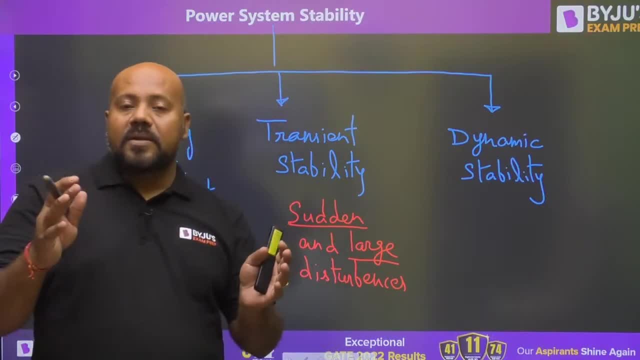 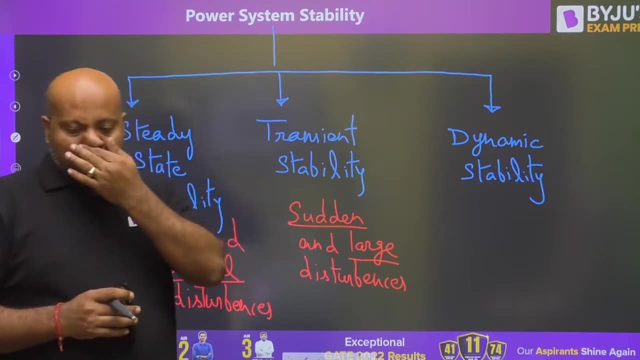 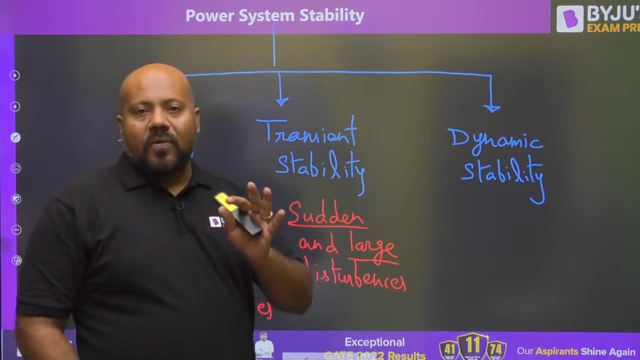 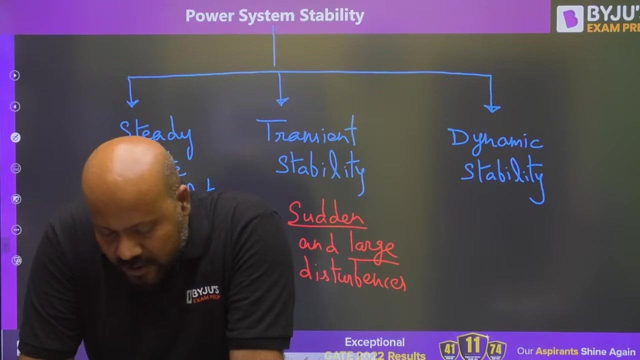 sudden means within no time, and large means the magnitude of change is significantly large. then we talk about the transient stability. is it clear now what is dynamic stability? first i will tell you what is dynamic stability, then i will tell you prachi kumari is saying stability. 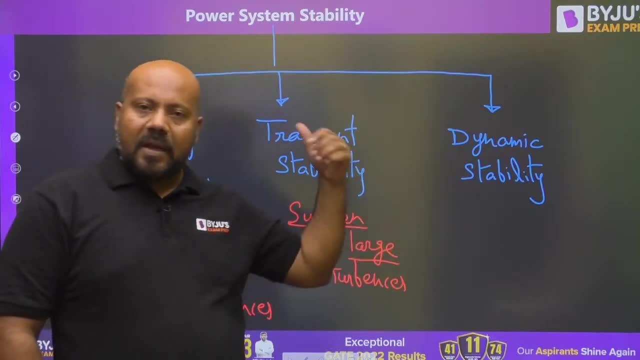 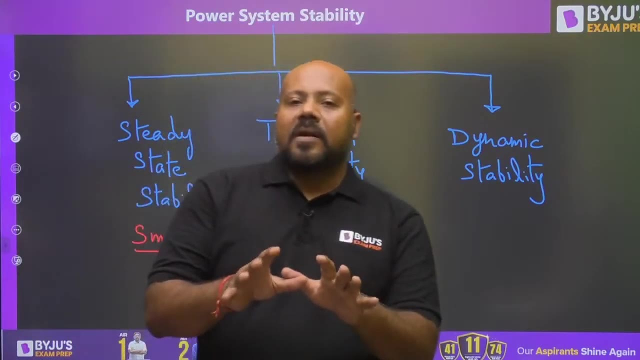 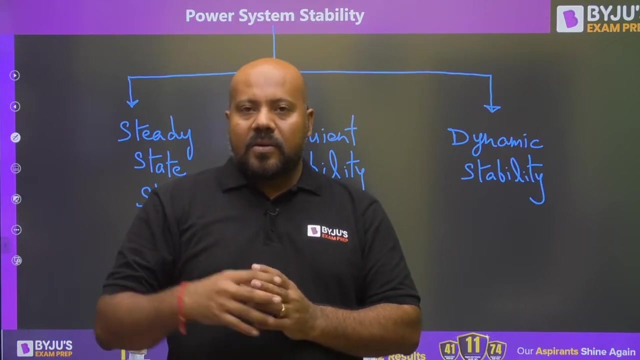 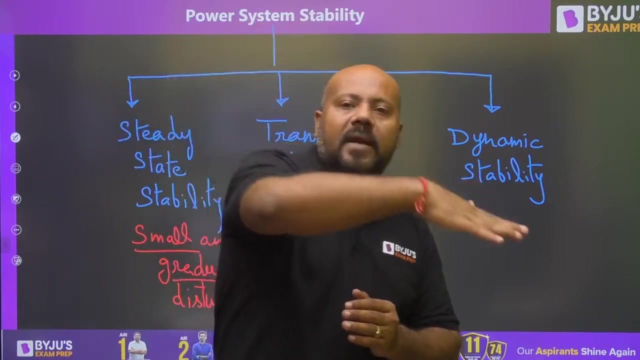 definitely, i will repeat, but let me just first complete this, then i will come back to the previous slide and i will tell you what is the stability, what is in this relativization, western stop. i will come back to it. so, in parts 10 to 17, adaptedCause: 61.8: water vapor with featuresesp. 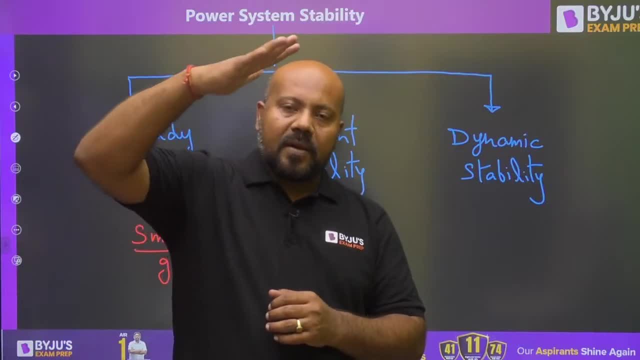 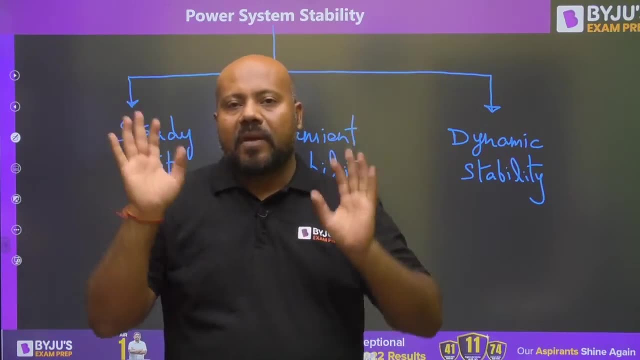 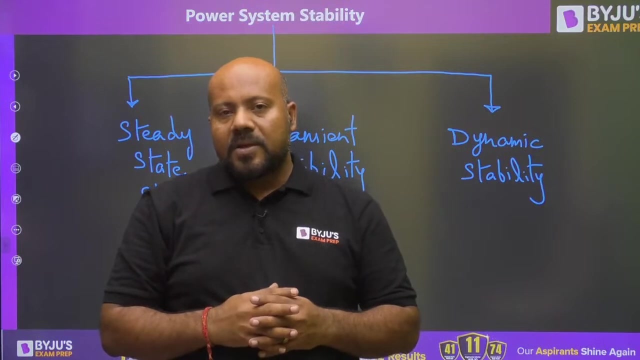 42' evaporated air and always fairly low oxygenступ 2 constant disturbance disturbance. It hardly matters what type of category you are going to travel. Still there will be at least some constant disturbances. Same example you can take in a car If you. 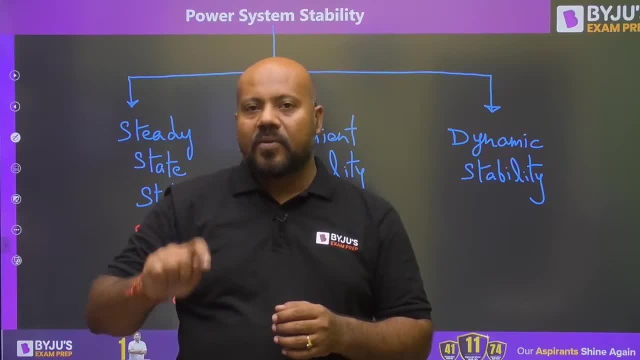 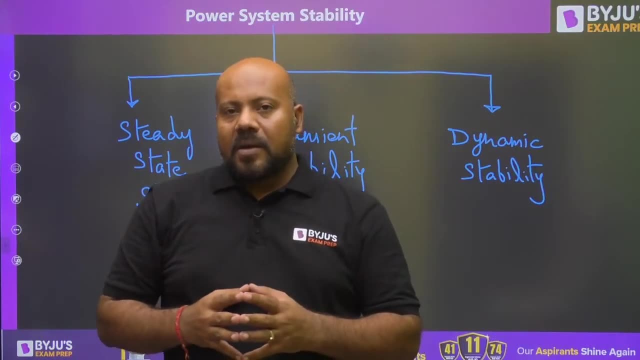 are traveling in your car. the moment you start your car and the moment you reach your destination and stop the car, there is a constant disturbance, constant disturbance. Even if you are sitting in a luxury car, still there will be some disturbances, but that may be. 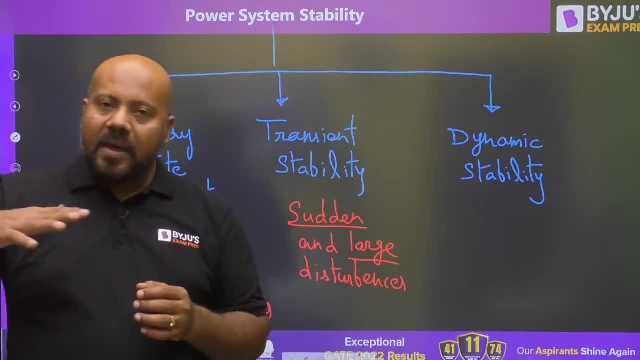 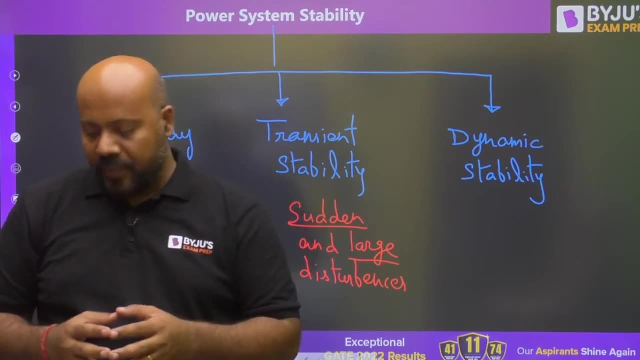 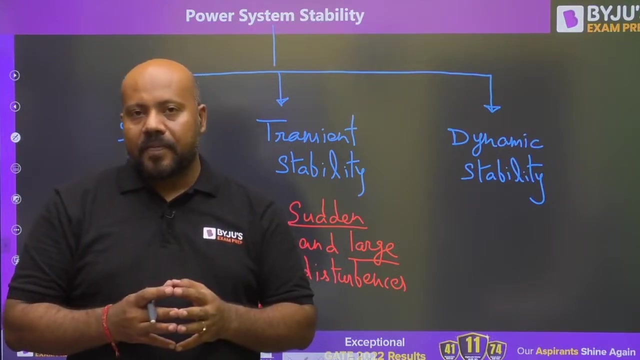 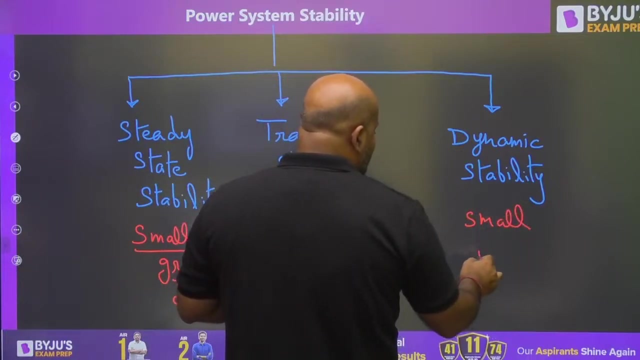 less because you have paid a lot of money, But there will be some disturbance throughout the operating of the system. This type of disturbance we are calling as categorizing as dynamic stability. So we are defining dynamic stability with the small but continuous disturbance. Small but continuous disturbance, Everybody just tell me in the 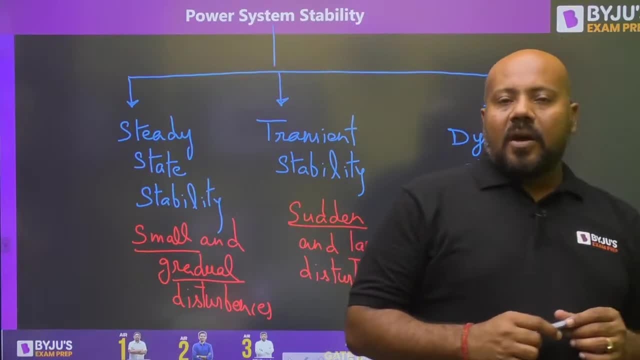 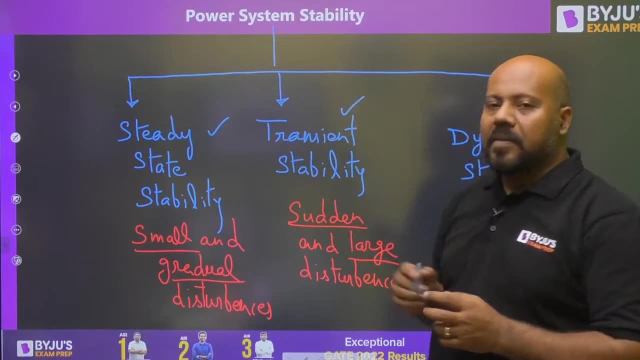 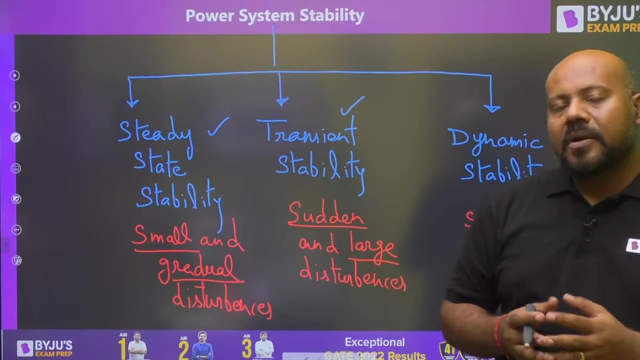 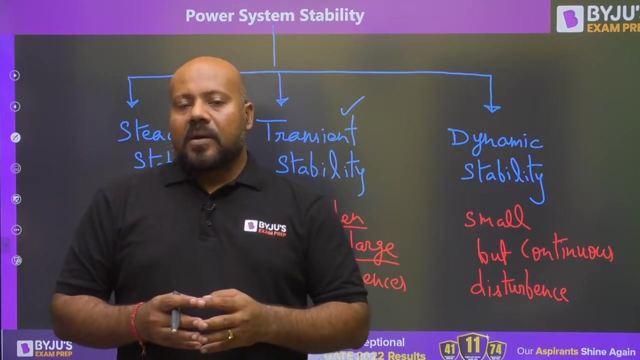 comment section. are you able to follow this? Now you have only steady state stability and transient stability in your slabs as far as gate or engineering services and other examples- arms- are concerned, but you may get a direct theoretical question on dynamic stability also. that is why you have to understand, you have to talk about dynamic stability also. 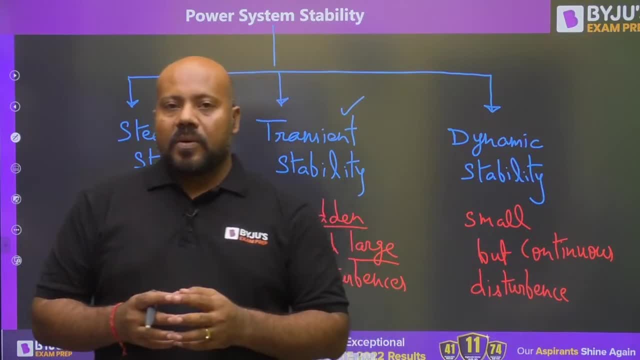 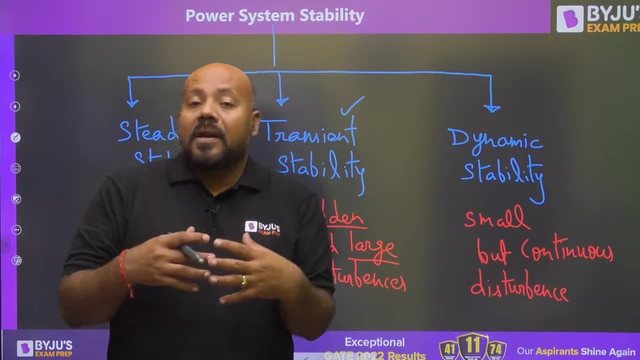 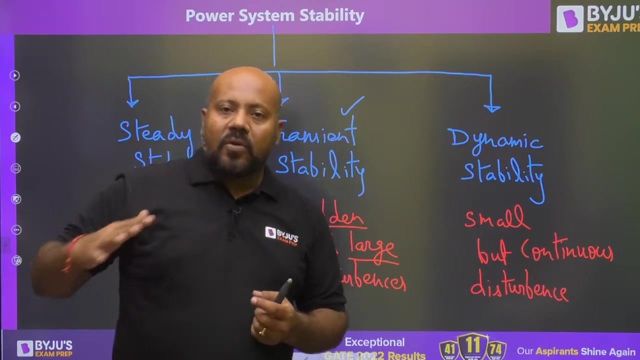 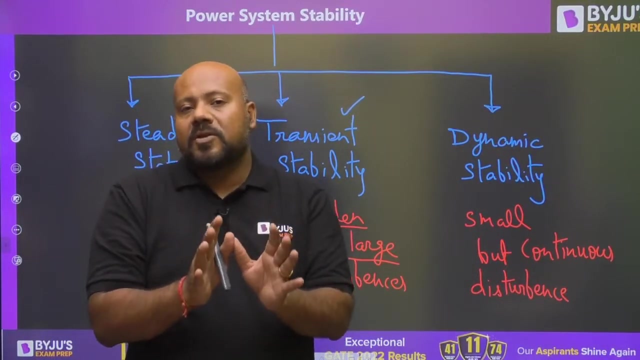 It is very difficult to remove these type of disturbances because the disturbances within the dynamic stability they are because of the very nature of existence of the system. If you don't want any disturbance, you don't fly. if you don't want any disturbance, you don't travel. but if the system is going to run, it is the inherent disturbance which is. 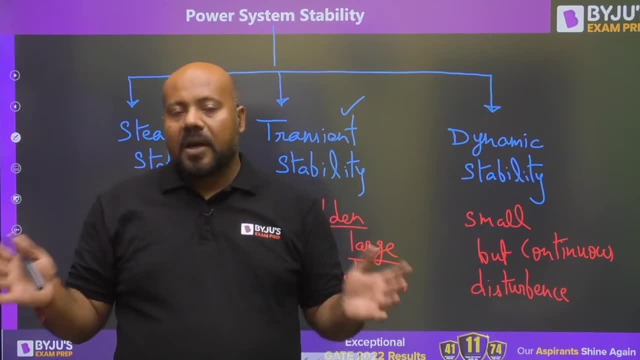 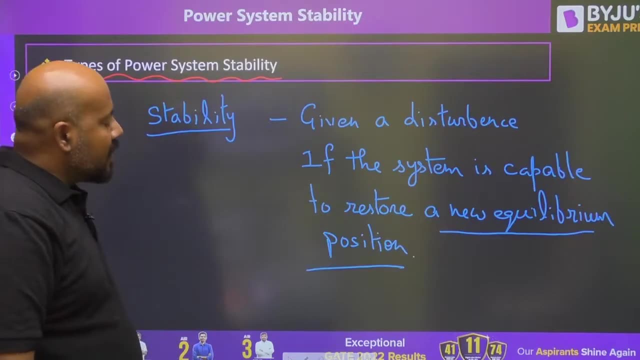 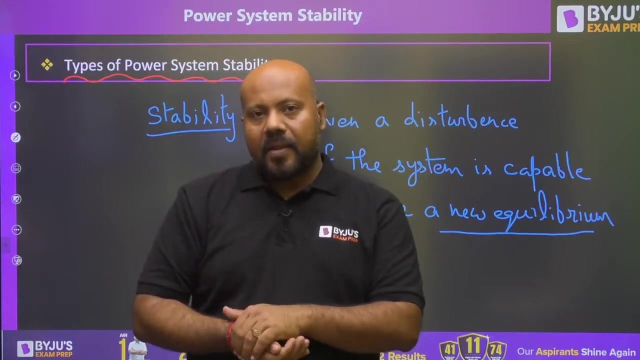 present and you cannot remove it hundred percent. are you getting this everybody? just tell me in the comment section. are you going to follow this? Now? Prachi is asking about defining the stability again, so let me just give you the same example once again in a different way. 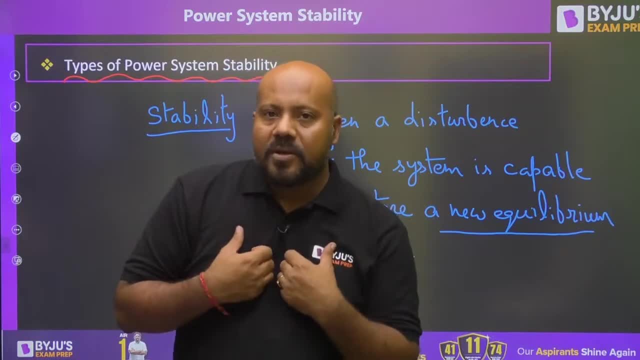 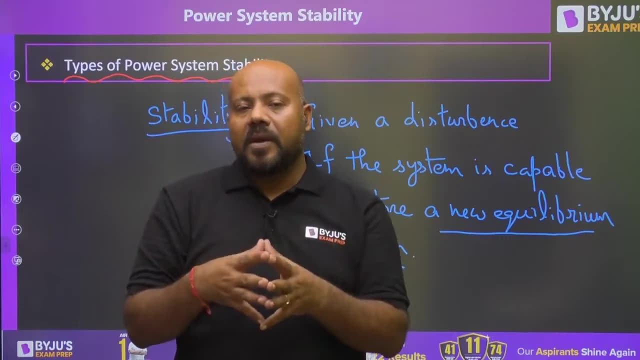 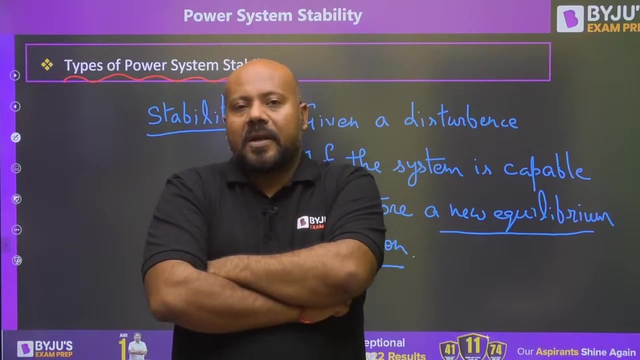 Now, first you have to, You have to tell me. I will show you my two positions, two circumstances, two situations. I will tell you, show you and you have to tell me in which situation I am more stable. First situation is this: suppose I am standing like this. 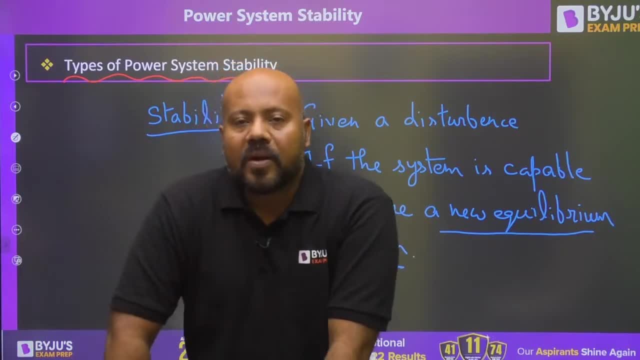 This is more stable? or suppose I am holding the table or some support I am taking and now I am standing like this. in which situation, first or second, I am more stable? Just by using your common sense you can say: yes, sir, when you are having some support, then 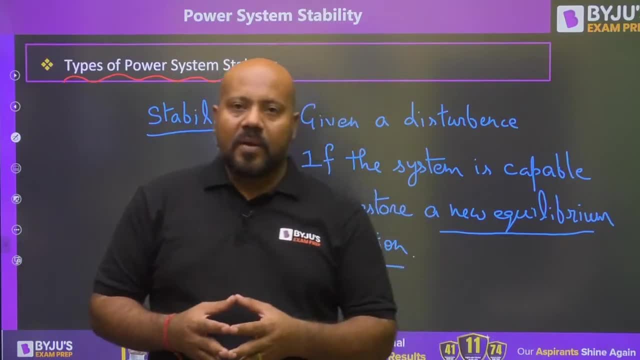 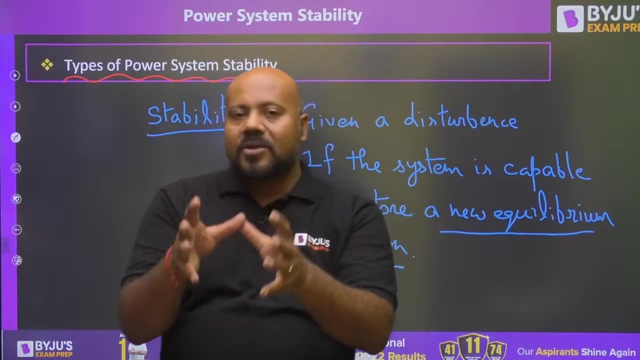 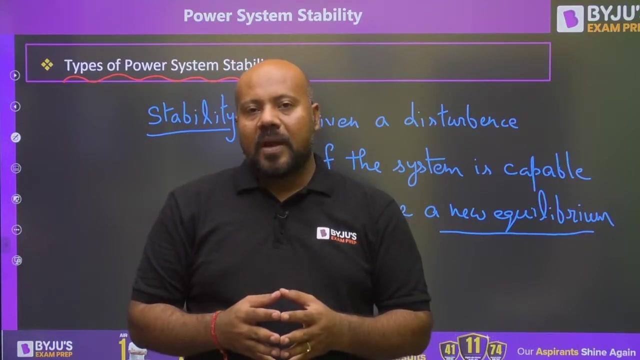 you are more stable. why you are saying so? Now understand the practical example. suppose I am standing like this and there is a notorious student in the class and he is coming from this side and he is going to give me a push, sudden push. I was unaware what will happen. the moment he pushes me, I will lean like this. 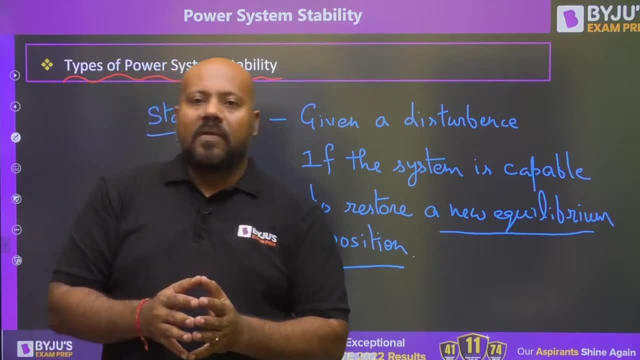 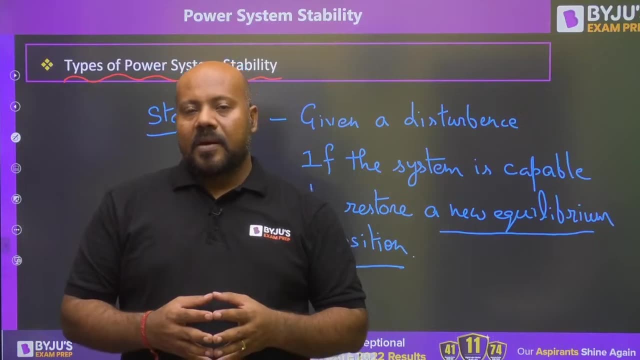 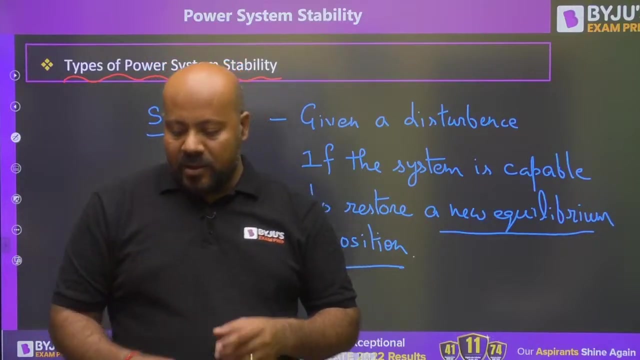 but if I am capable to manage myself, I will manage myself and I will come back or restore to a new equilibrium position. This is what we call stability. With this example you can understand that stability you cannot discuss without a disturbance. So the first thing you have to understand is: given a disturbance only if the disturbance 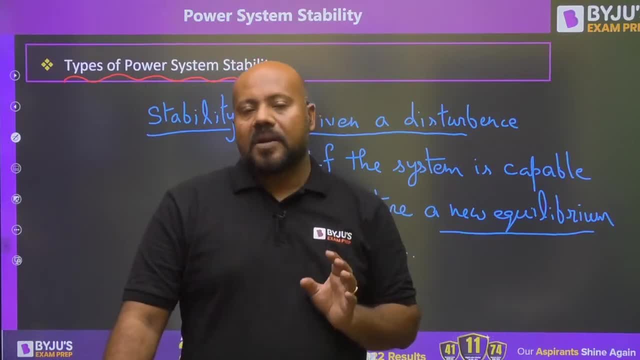 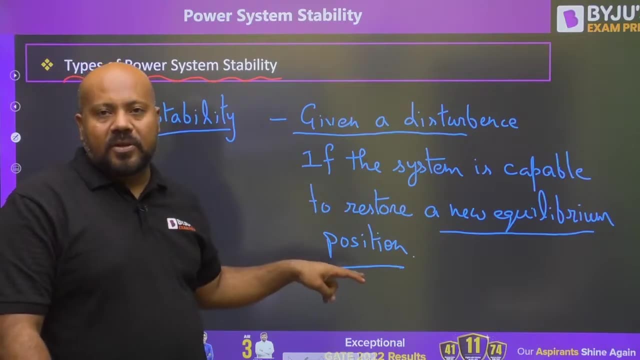 is present, then only you can talk about the stability second thing. if the system is capable to restore In New equilibrium position, then you are saying system is stable. I hope you are getting this. Is it clear everybody? just tell me in the comment section. 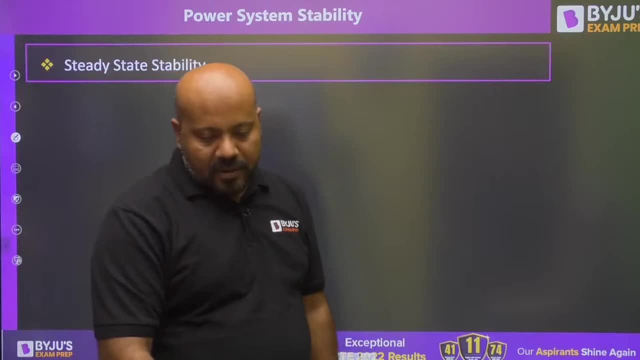 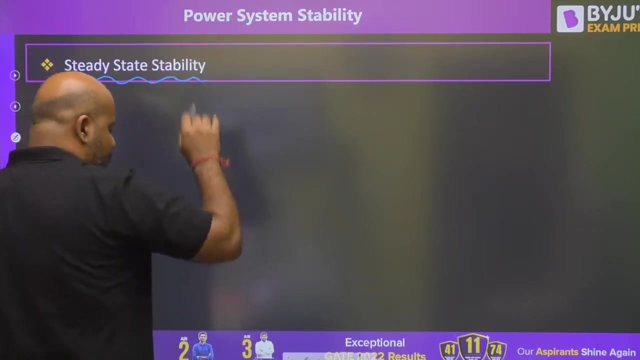 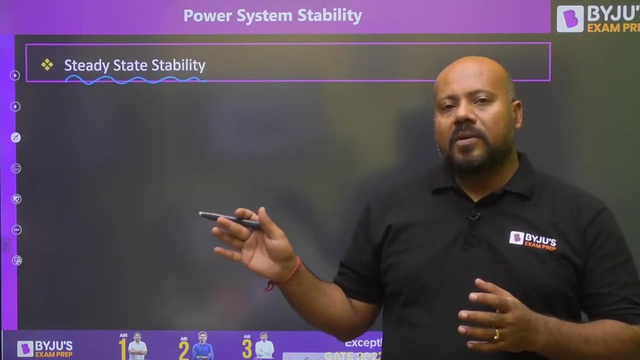 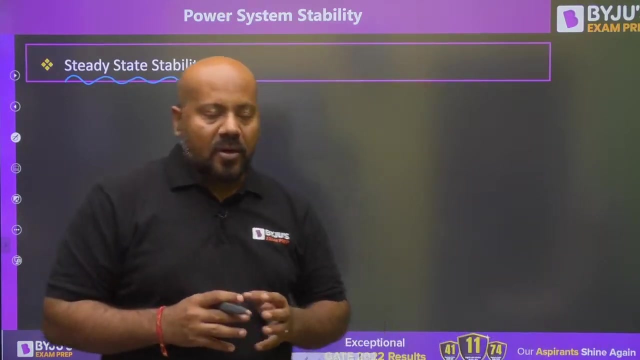 Now let us talk about the steady state stability. Is it clear- Now let us talk about the steady state stability- how you are going to understand that, whether in the question or the interview, somebody is talking about steady state stability, only one difference. you have to understand that difference is small and gradual changes, or? 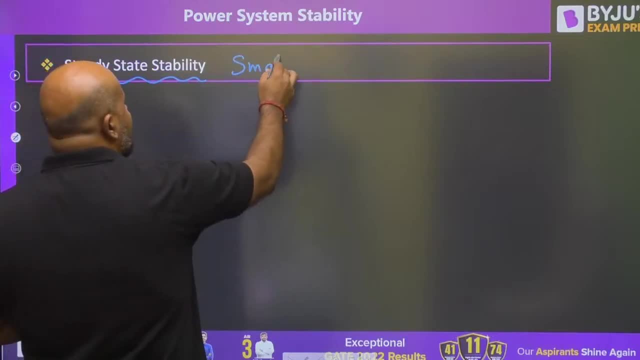 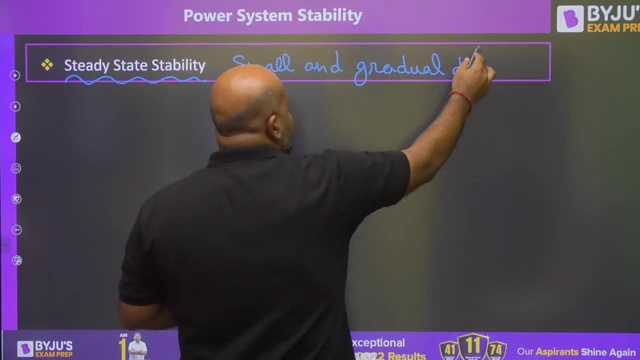 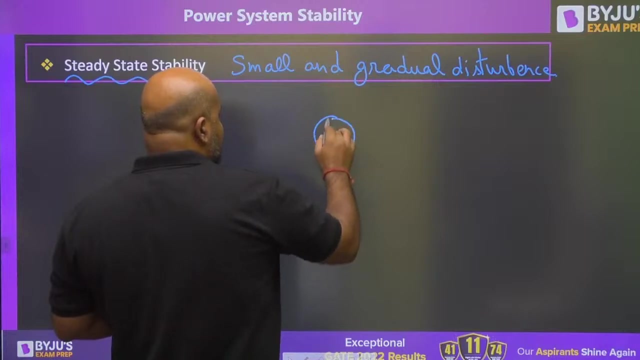 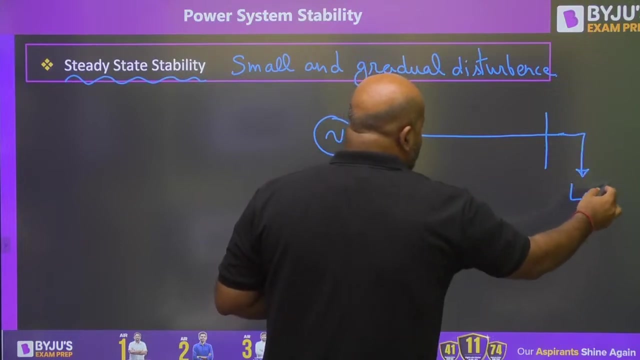 disturbance. So you are going to write here small and gradual changes or disturbance. now let me take a simple power system. Suppose this is the generator, This is the transmission line, and suppose this is a load. This load is having this much real power requirement and this much reactive power requirement. 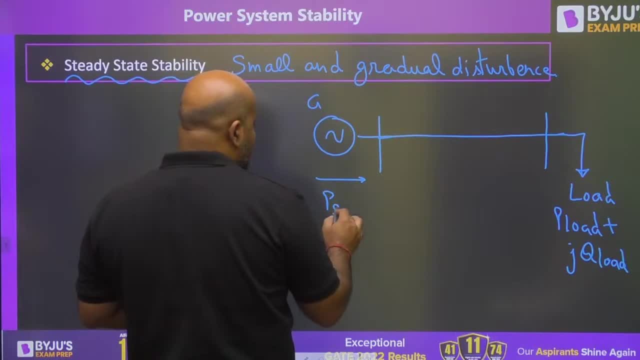 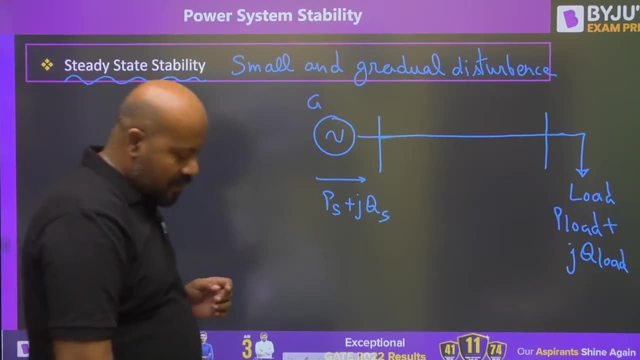 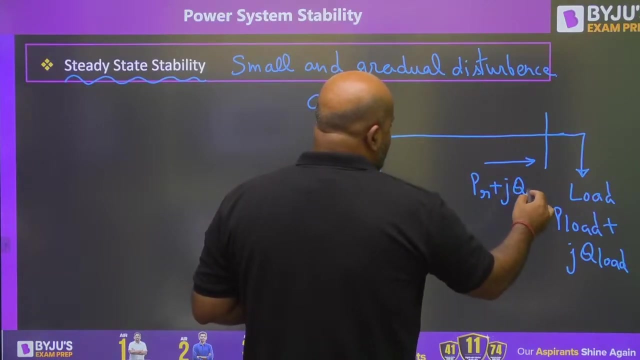 This is the generator and this generator is suppose sending PSJQS. This is the real and reactive power sent by the generator. and suppose at the receiving end the power which is received is PR plus JQR. that is real and reactive power received at the receiving end. 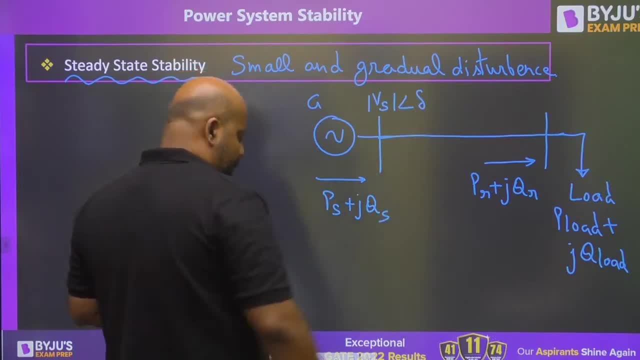 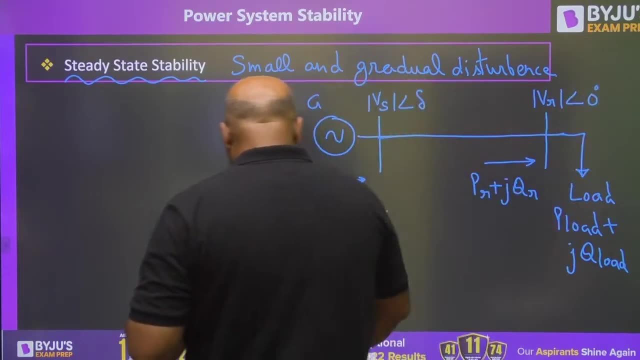 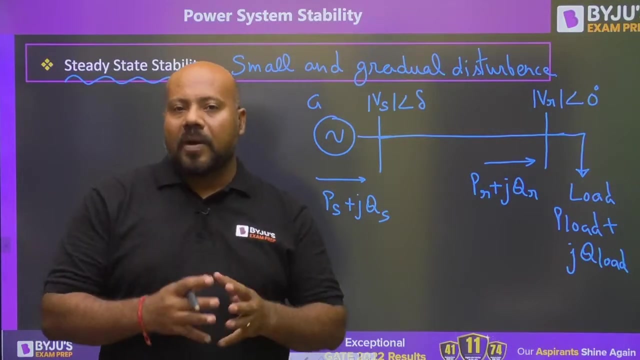 Suppose the voltage at the sending edge is mod Vs angle del and voltage at the receiving end is mod VR angle, 0 degree. Now please try to understand one thing: when you talk about efficiency, you always talk in terms of real power, Yes or no? 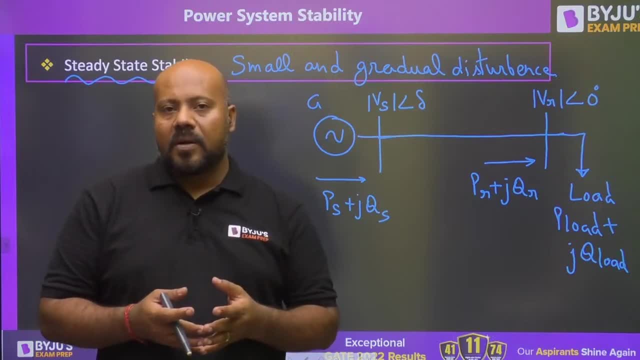 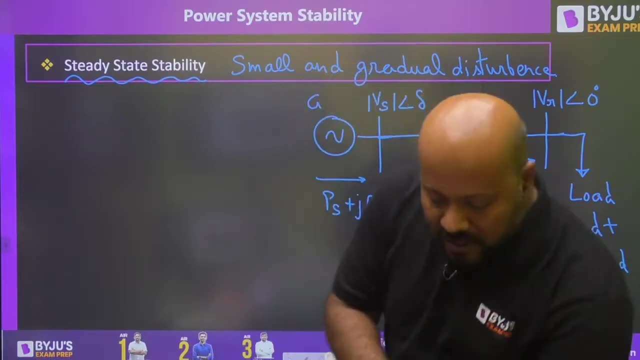 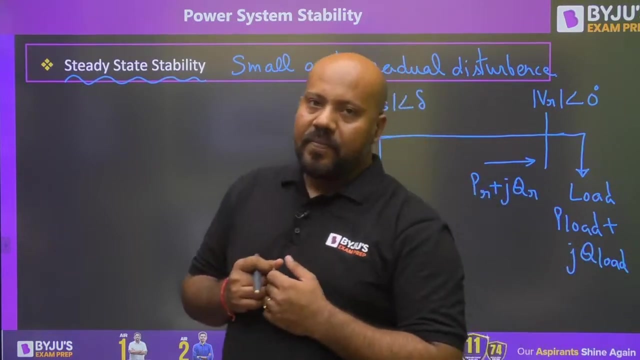 When you write the efficiency formula P output upon P input. what is that P? that P is real power. So you are talking in terms of real power when you talk about the efficiency. similarly, when you talk about the stability, again you talk in terms of the real power. 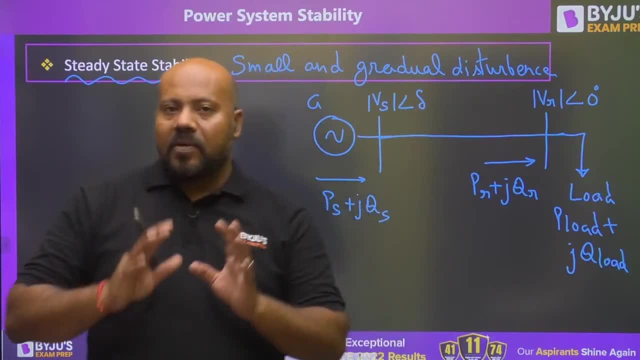 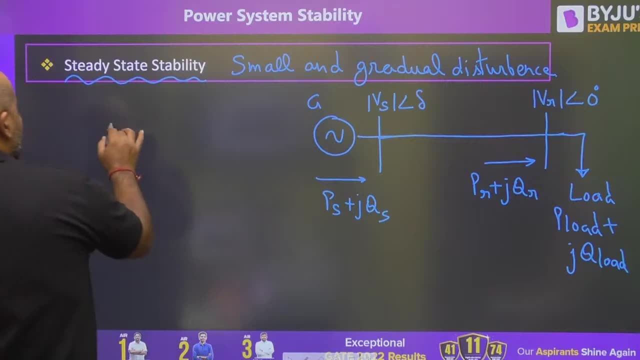 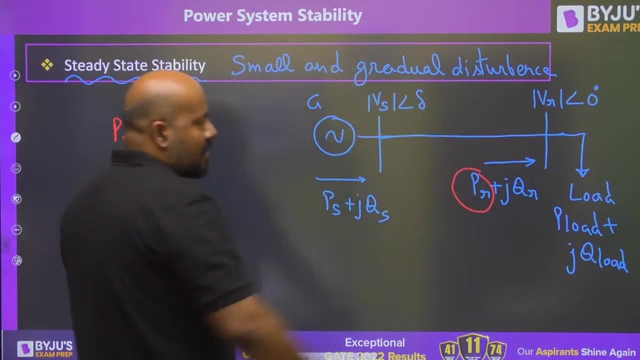 So when we talk about the stability, we are interested in the real power, not the reactive power. So can anyone tell me what is the expression I can write for the efficiency formula: Real power received at the receiving end. I am interested in this parameter: real power received at the receiving end. 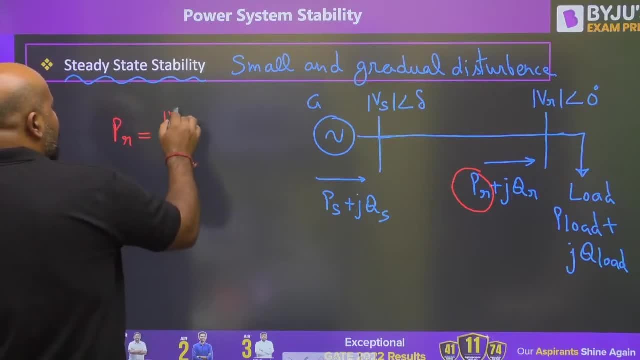 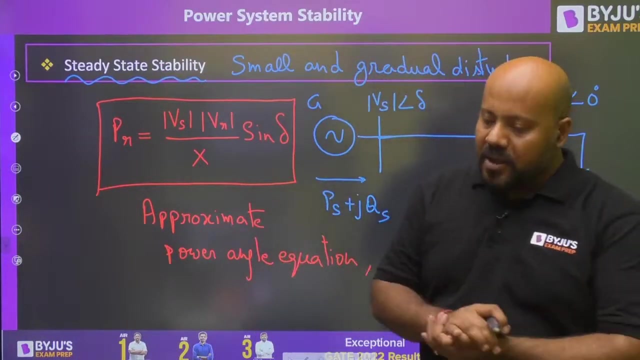 Can anybody guess? It is going to be mod Vs, mod VR upon X and this is going to be sin del, yes or no? What is this? This is the approximate, Approximate power angle equation, yes or no? Now, this equation is going to give us some idea about the stability. 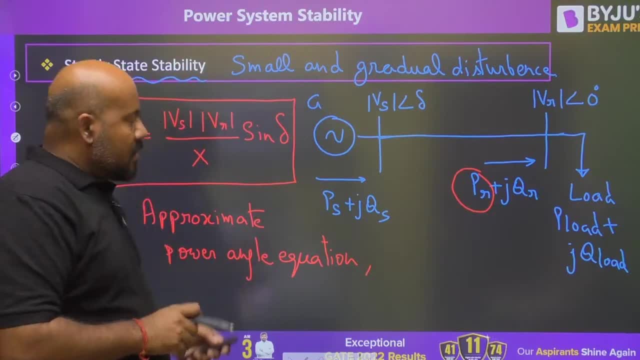 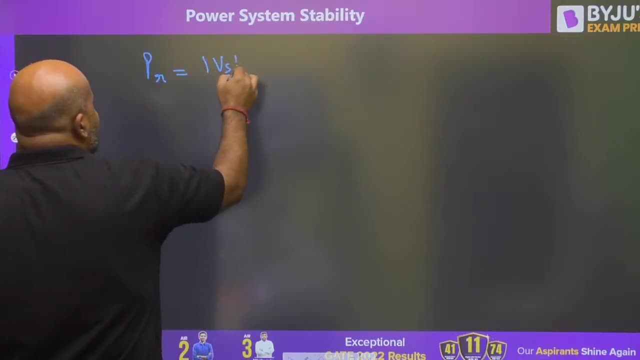 Let us try to analyze this equation. So if you are saying your equation is mod Vs, mod VR upon X, Yes or no, Yes or no, Yes or no. Now, if you are saying mod VR upon X, sin del, you can understand that this equation del 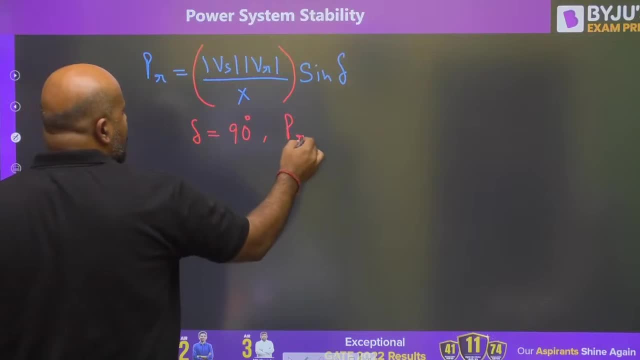 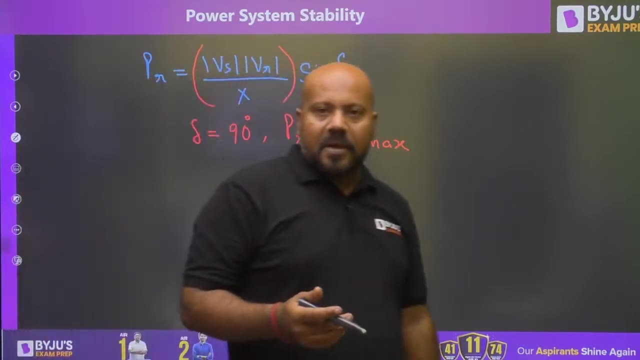 is equal to 90 degree is going to give you the maximum value of the real power received at the receiving end, Yes or no? When del is going to be 90 degrees, sin del is going to be 1 and for this sinusoidal equation, 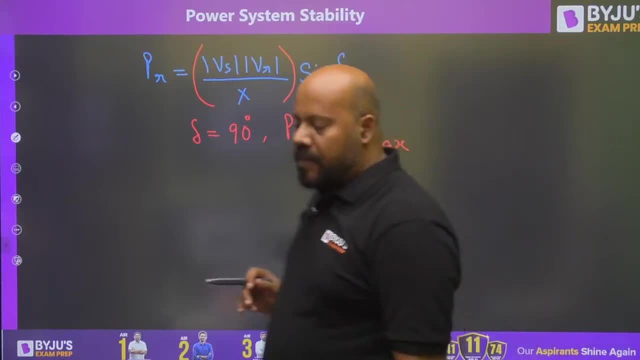 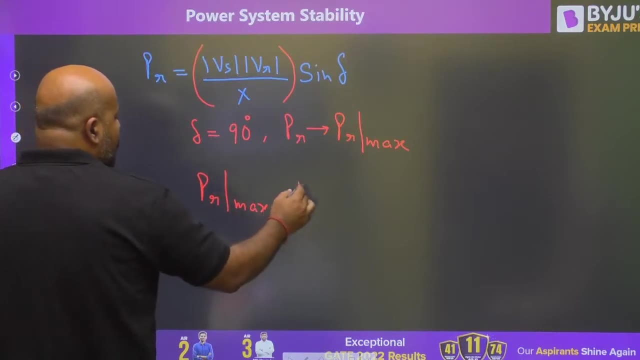 you will be getting the maximum real power received at the receiving end. What is the value of this maximum real power? The value of this maximum real power is going to be mod Vs, mod Vr upon x. So now I can rewrite this equation and I can write: Pr is equal to Pr max and sin del. 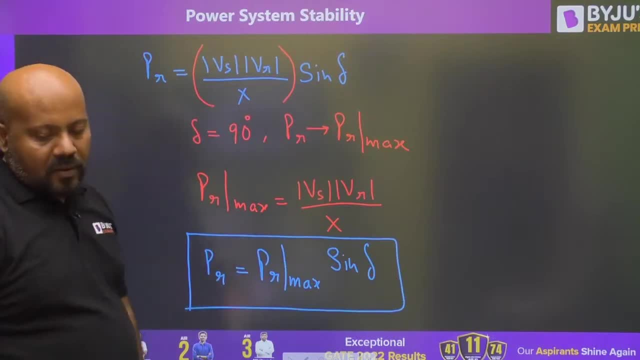 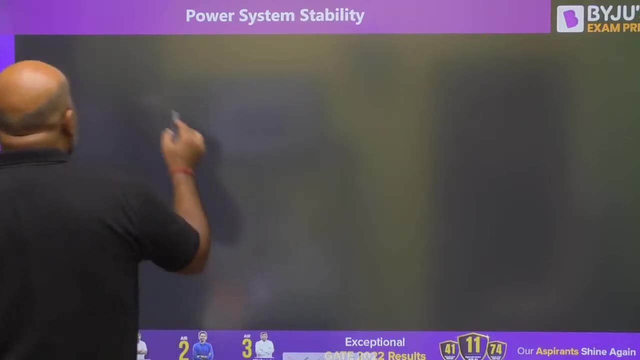 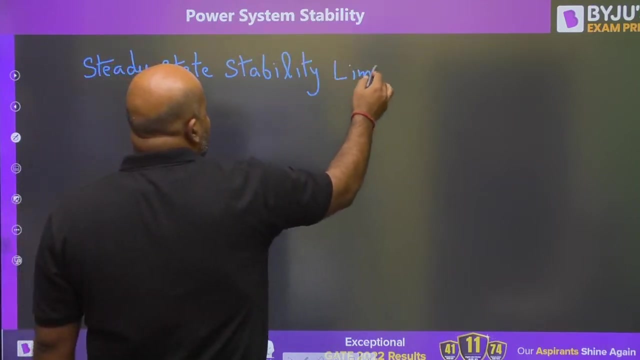 This is going to be my final expression, which I am going to use for the stability analysis, This Pr max. we are using another term for this, that is steady state stability limit. Why we are saying so we will discuss, don't worry, This is steady state stability limit is nothing but. 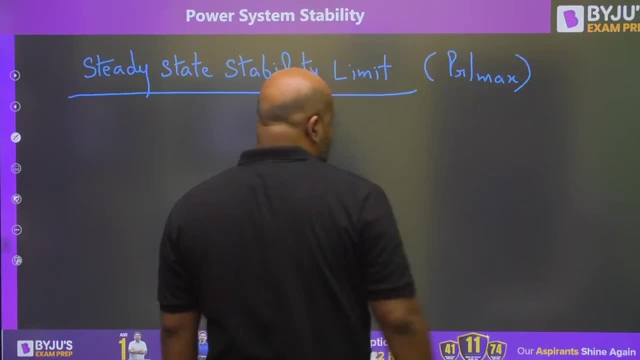 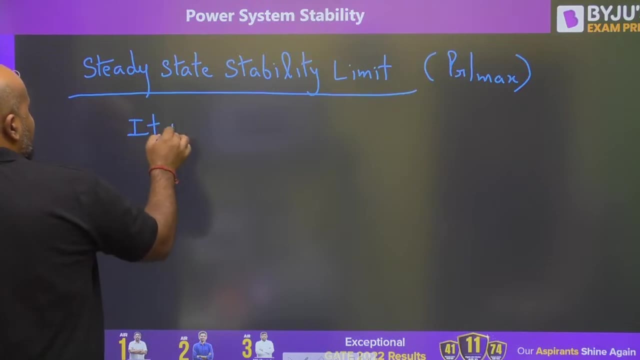 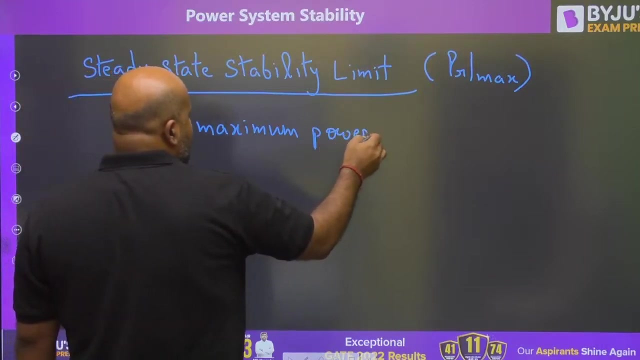 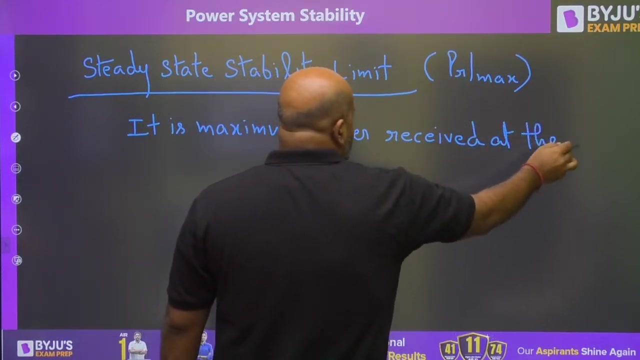 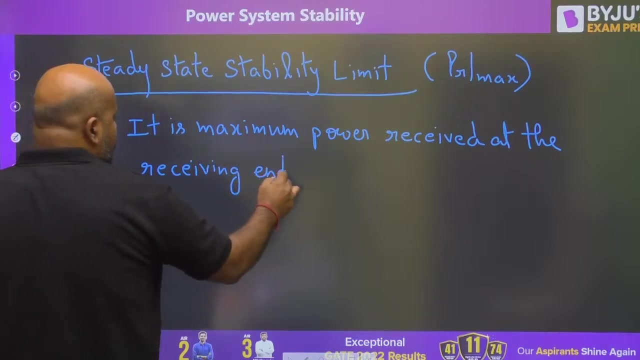 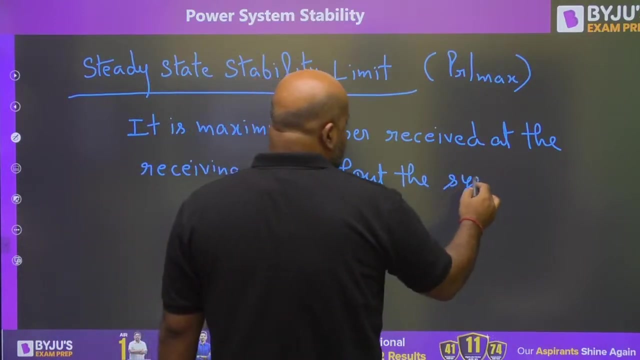 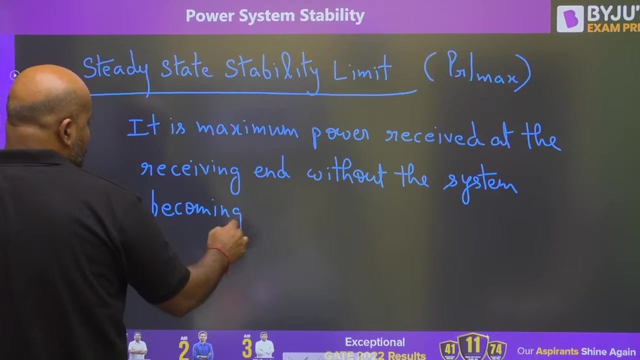 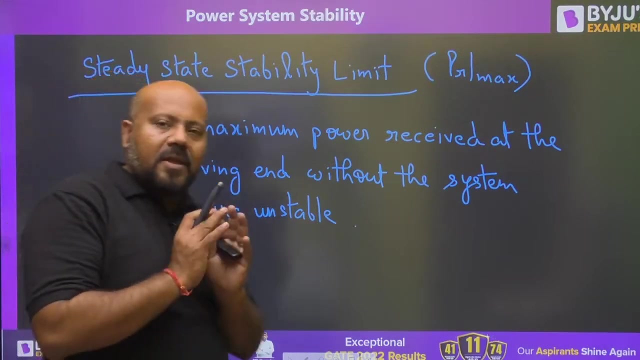 The maximum real power received at the receiving end. How we are defining it. Let us try to understand. It is the maximum power received at the receiving end Without the system becoming unstable. What is the idea here? You are saying this is the maximum power which can be sent or, sorry, which can be received. 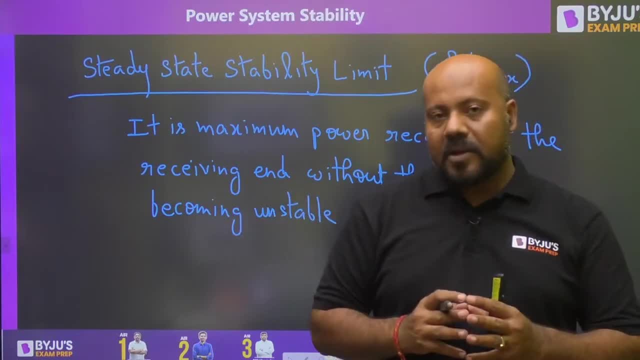 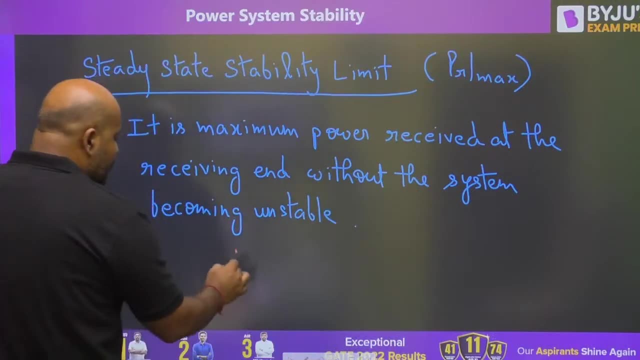 at the receiving end Without the system Having its stability. It means if more power is transferred, the system is going to become unstable for sure. So can I say: if the real power received at the receiving end is more than Pr max, then the system is going to become unstable. 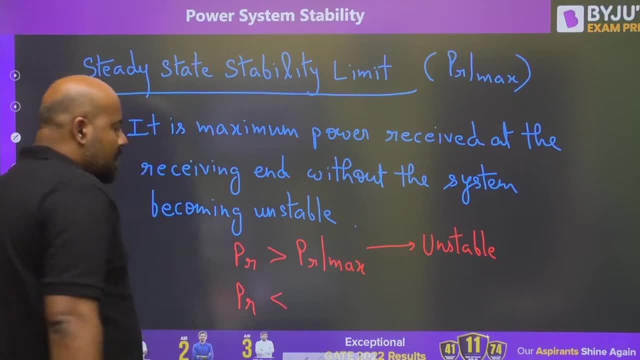 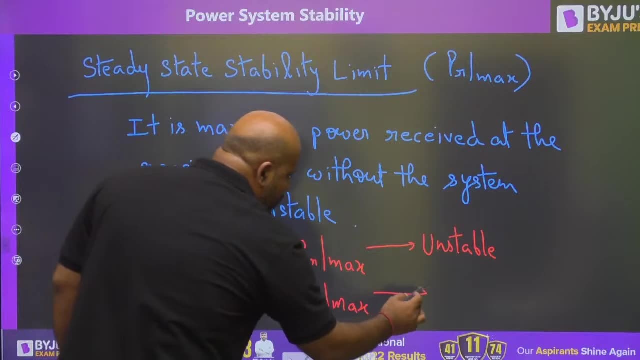 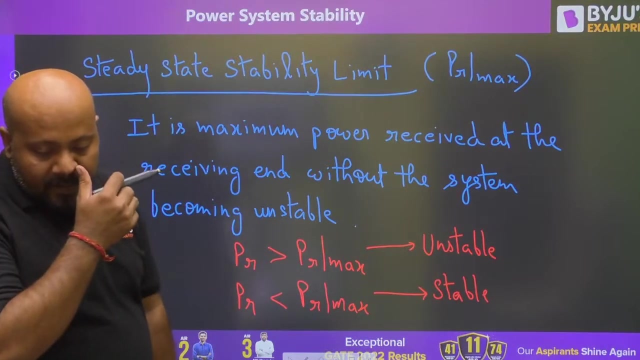 In other words, I can say: if the real power received at the receiving end is less than this value, That is Pr max. That is Pr max, Then the system is going to be stable. But the story is not over. Let us try to understand with the help of the power angle curve. 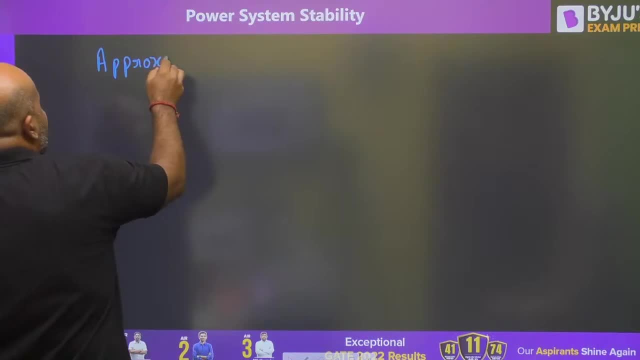 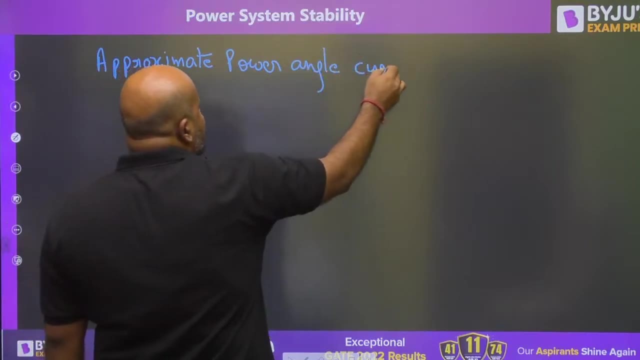 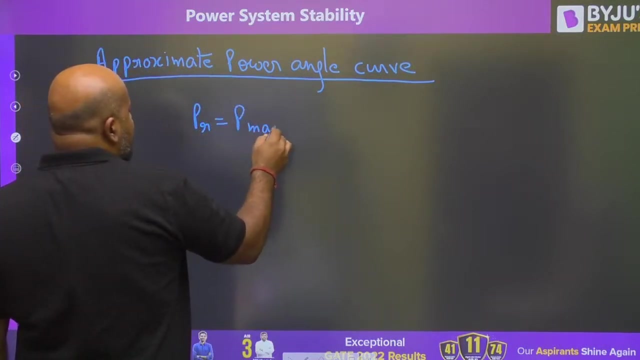 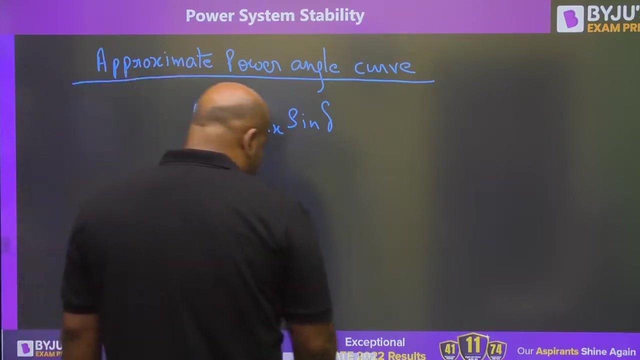 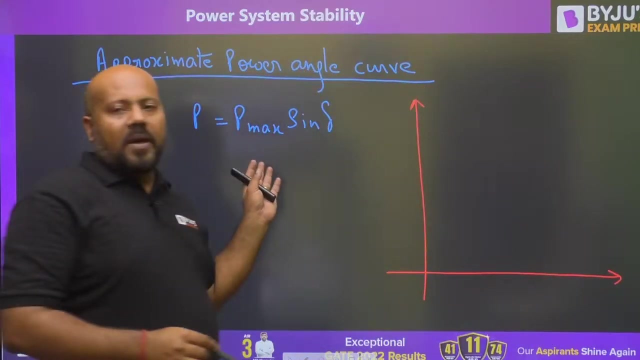 What is this? approximate power angle curve? Approximate power angle curve. You have the equation: Pr is equal to Pr max sin del. or just forget this Pr and write it simply P, to make it simple. Now, very easily, you can understand. it is going to be a sinusoidal variation. 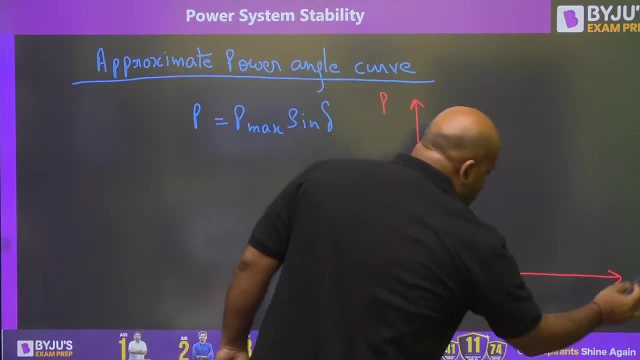 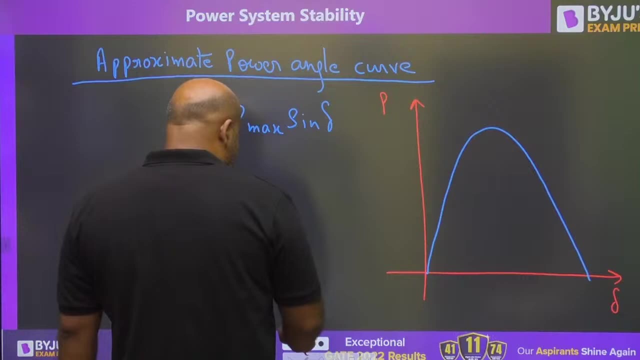 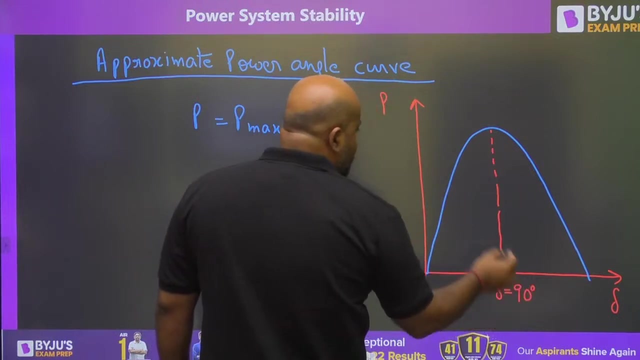 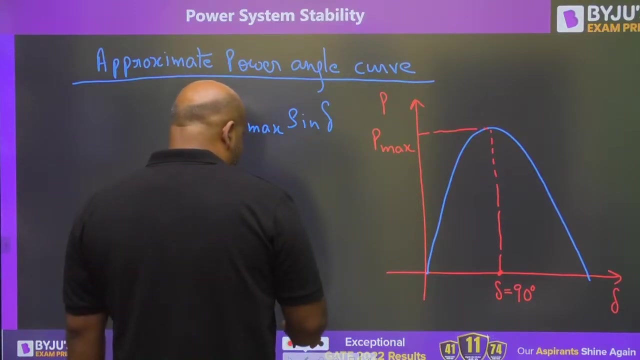 So this is your real power and this is your power angle, and the variation is going to be sinusoidal, something like this. Now you are saying: At del is equal to 90 degree, del is equal to 90 degree, You are getting the Pr max situation. 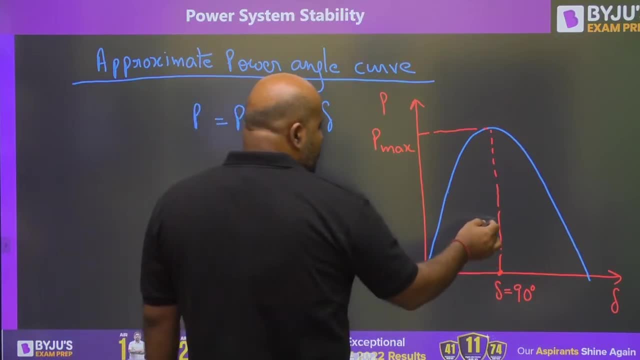 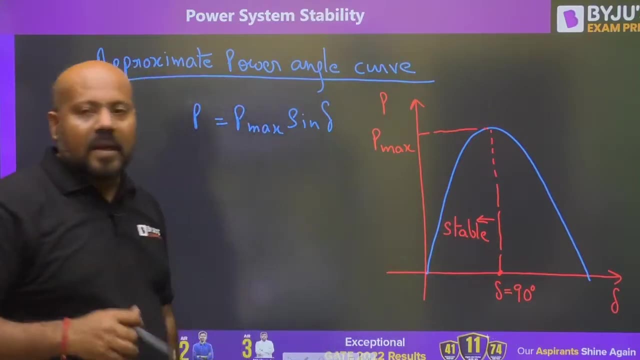 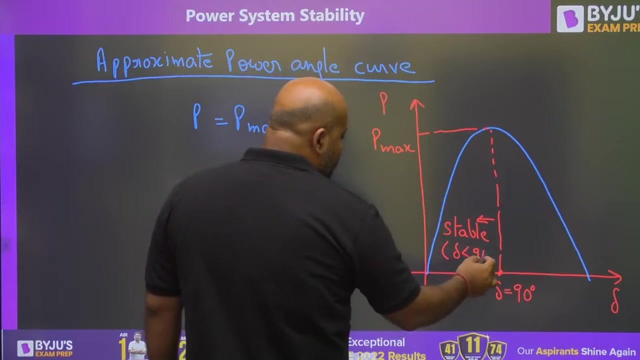 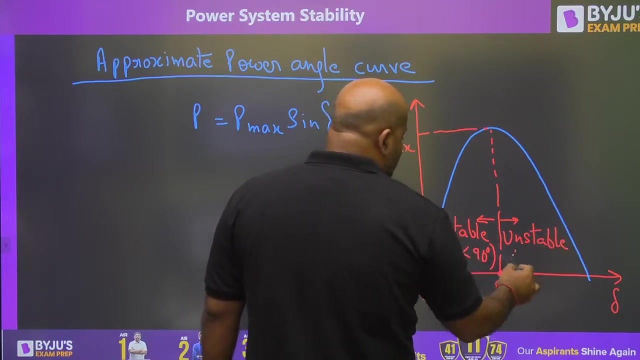 Also, you are saying that in this region, the system is stable when the power transferred is less than del is equal to 90 degree. You are saying the system is stable, Ok, And system is unstable in this region when del angle is more than 90 degree. 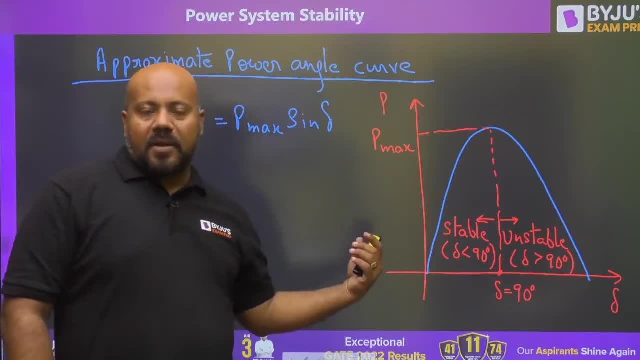 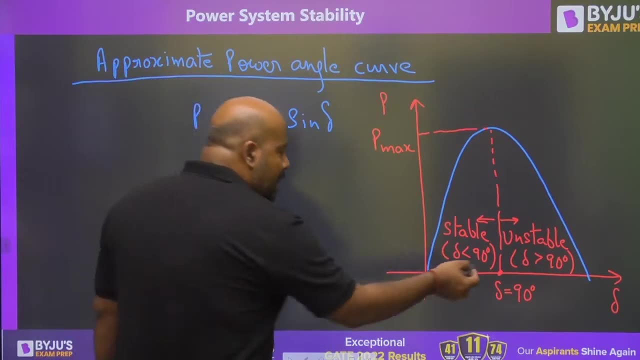 Now why we are saying that del less than 90 degree the system is stable and del more than 90 degree the system is unstable. Let us try to understand Exactly. at del is equal to 90 degree, we are having the marginally stable system. 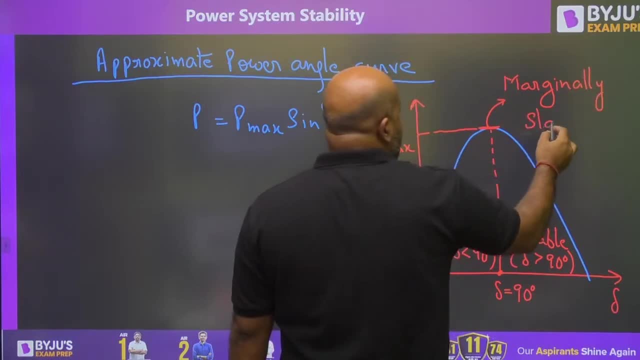 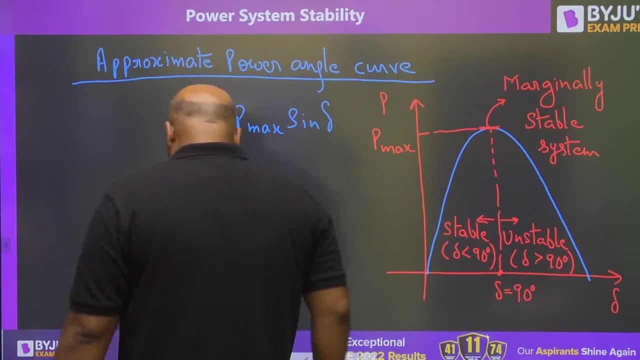 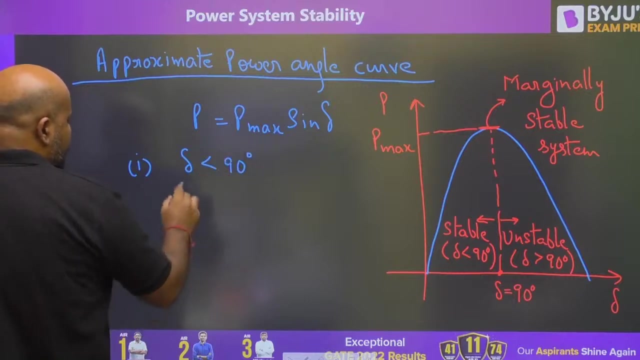 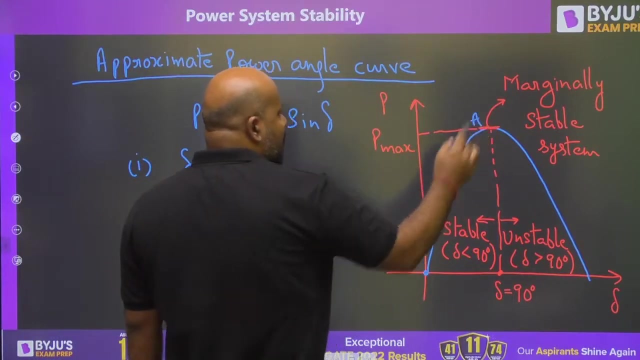 So let us consider the first condition. What is the first condition? The first condition is: del is less than 90 degree. When del is less than 90 degree, it means you are talking about 0 to A. Suppose this point is A From 0 to A, what is the slope of the curve? 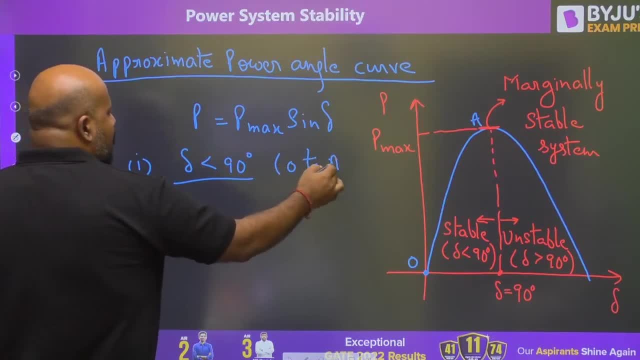 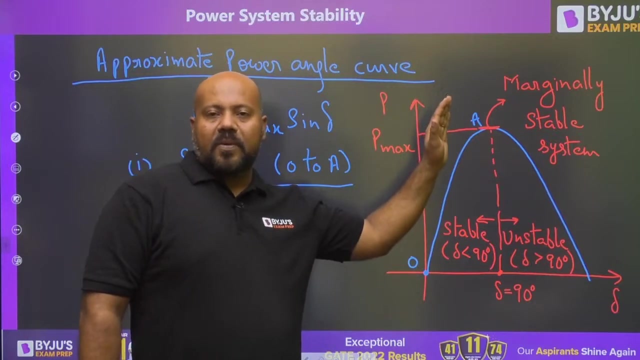 The slope of the curve is dp upon d del and this is positive. You can see the slope of the curve, Can you see? my hand Gives you the slope of the curve. It is positive. dp by d del is positive. What is the meaning of dp by d del- positive? 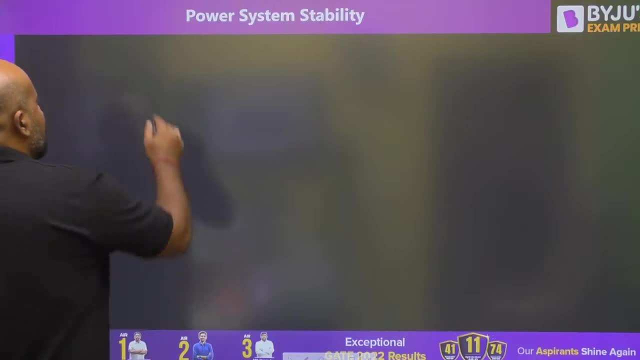 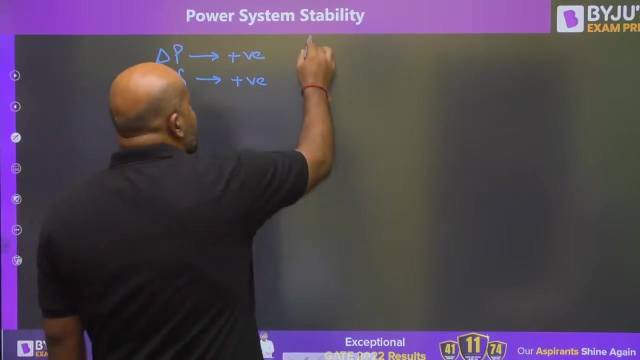 Let us try to understand. Ok, If you are saying Change in P, Ok is delta p, and this is positive, And change in del is delta del, and this is also positive. Similarly, change in p that is delta p is suppose negative and change in del, that is delta del is. 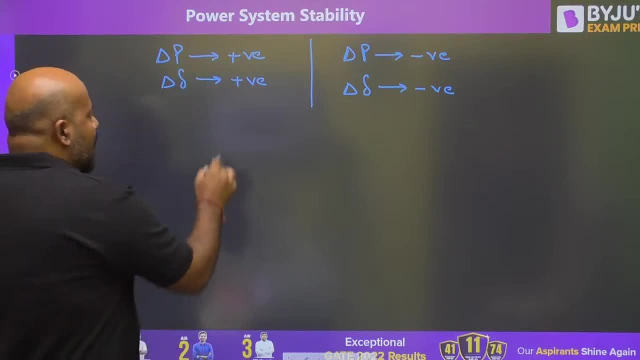 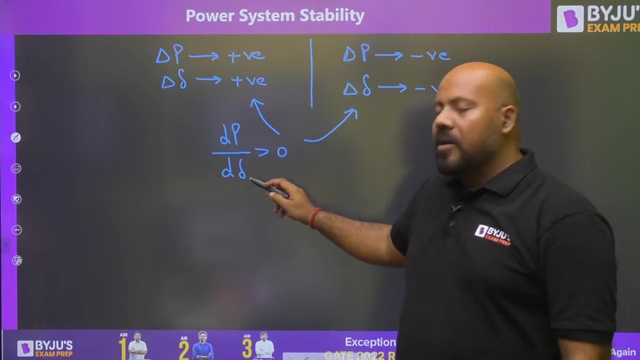 also negative If you are having the slope dp by d, del positive, so you can have only two conditions. You can have only two conditions. Are you getting this or not? If the change in p and the change in del- both are positive, then this slope is going to be positive. If the change in p and the change 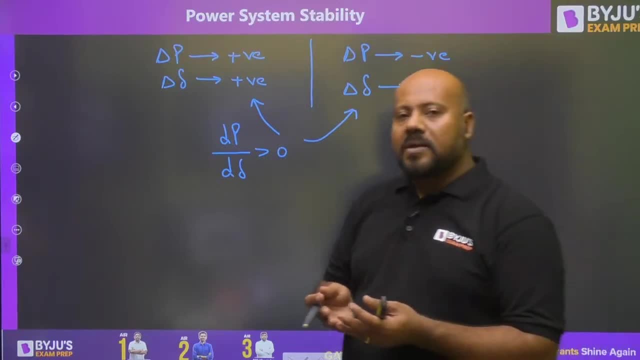 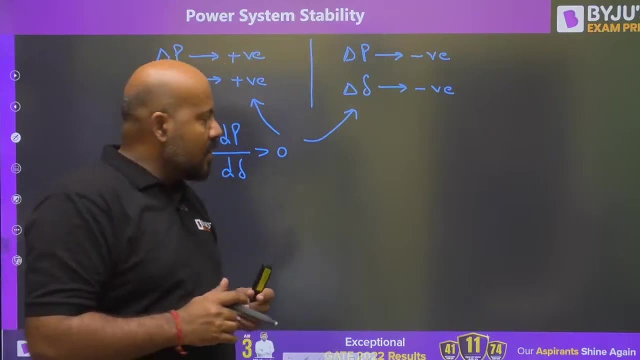 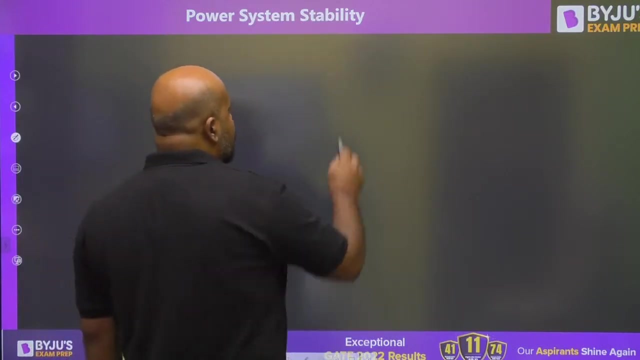 in del, both are going to be negative. so again, you are getting the slope as positive or more than 0.. What is the practical understanding of this? Let us try to understand. Suppose, at any particular point of time, suppose this is the situation. 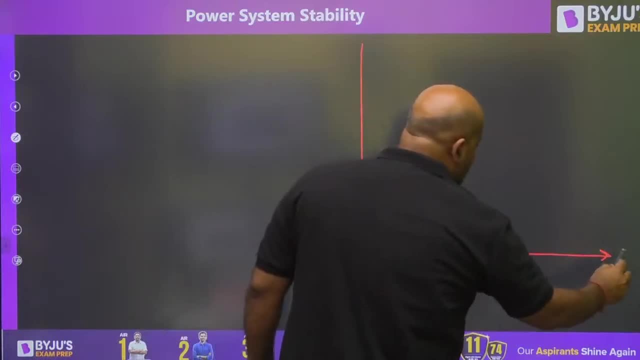 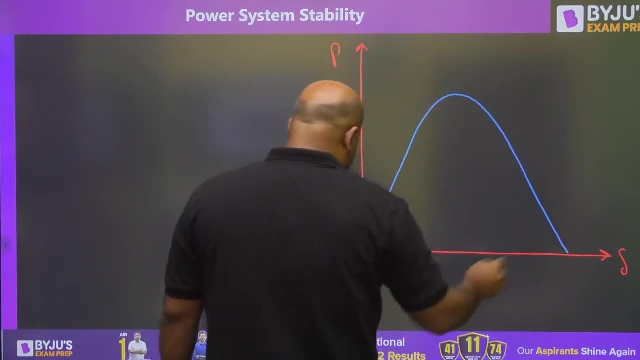 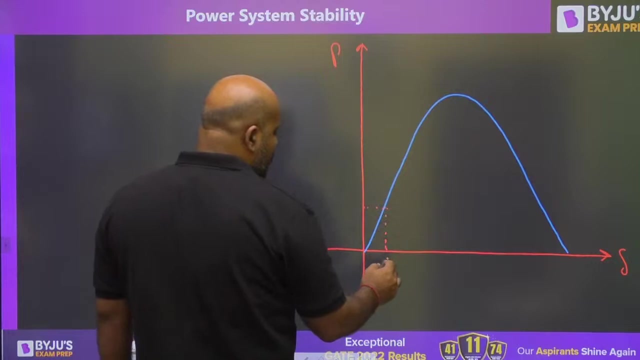 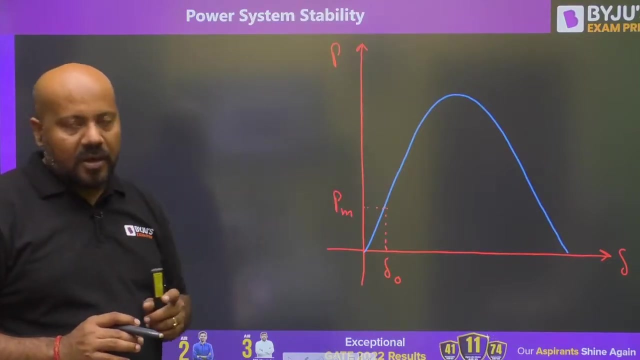 del and this is p. and suppose this is your power angle curve. Now suppose, at any particular point of time you are at del 0 and this is the real power that is supplied by the generator or received at the load end. Now suddenly, 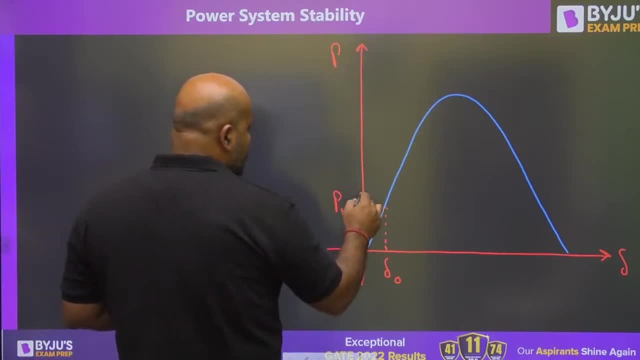 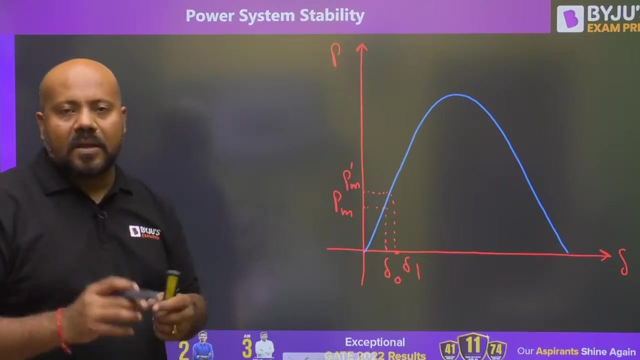 suppose this is the situation: del 0 and this is the real power that is supplied by the generator. Suppose you have increased the load and you want to transmit or send p m dash power. So what is happening Now? you are operating at some other power angle, that is, del 1.. 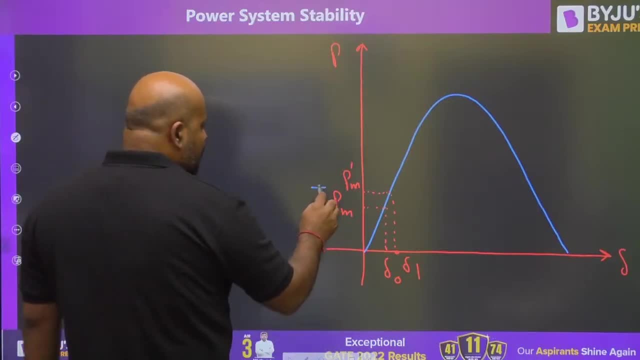 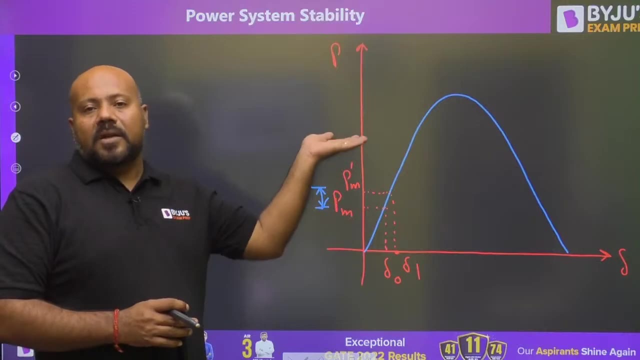 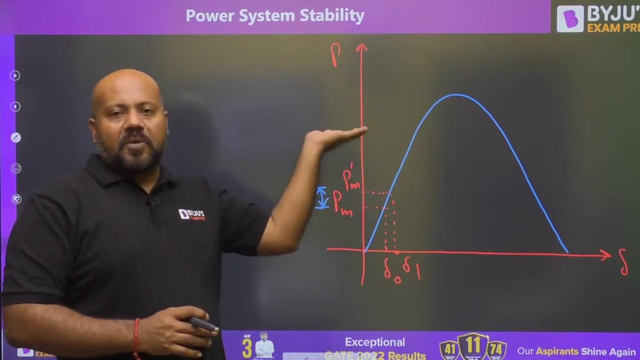 Now, if you see, because of this disturbance- what is this disturbance? The p, m or the power received by the load is increased, Then del also increase. Are you getting this or not? When the change in P is positive, the change in del is also positive. Both are positive means positive slope, So system. 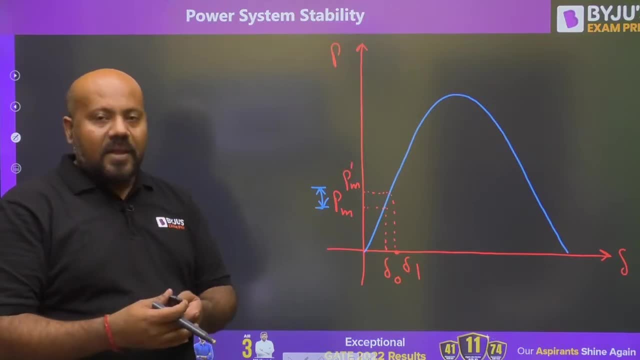 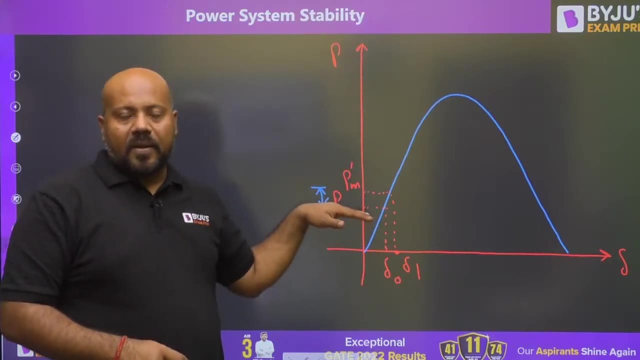 is stable, Yes or no? In the other case, suppose initially you are operating at Pm' and del 1 and you want to reduce the power sent or power given to the load to Pm. It means the change in P is negative, So the change in del should also be negative If your system 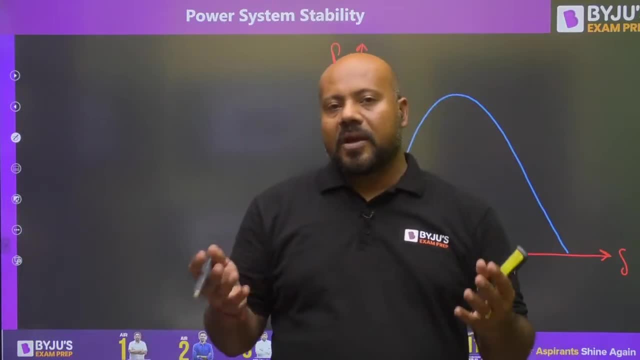 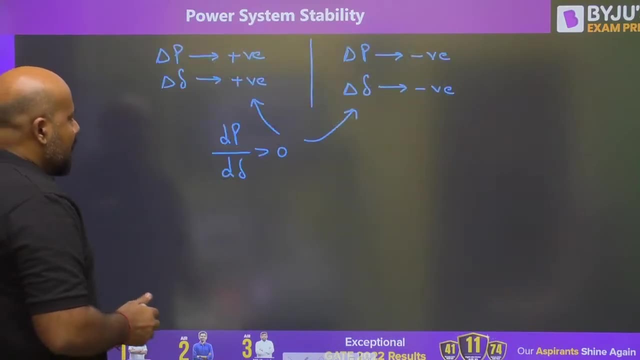 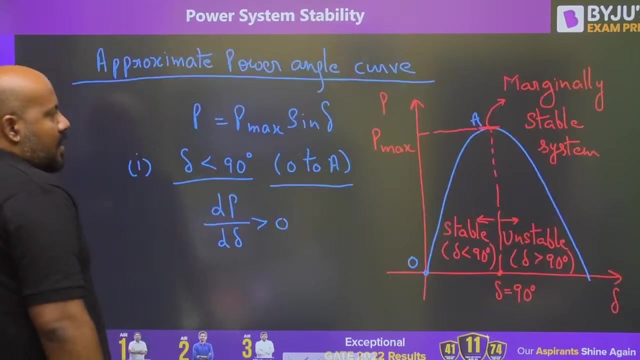 is able to match with the demand on the system, then you are saying your system is stable. I hope it is clear for everyone. Just tell me in the comment section. The second case, when del is equal to 90 degree. That is point A. In this case, if you see the slope of the curve is zero Dp by D del. 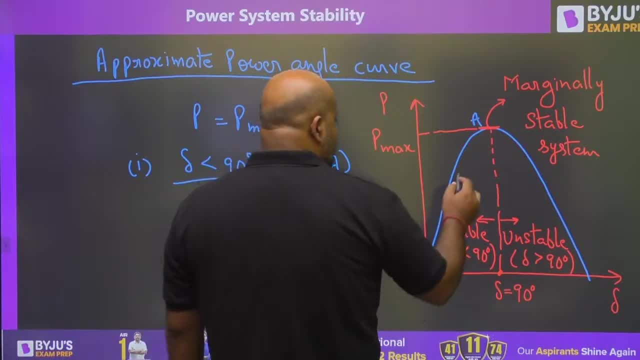 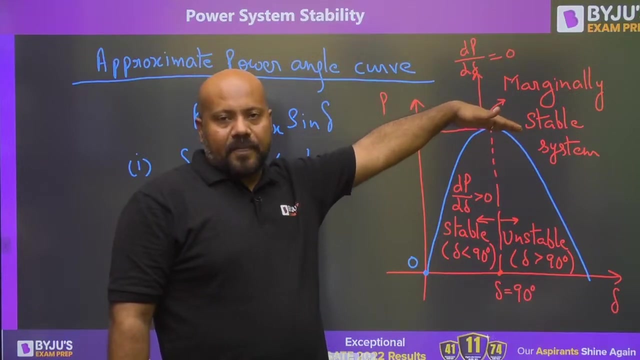 is zero. In the stable part. Dp by D del is greater than zero At point A. Dp by D del is zero When the slope is zero because it is the peak point. Are you getting this? So the system is marginally stable. 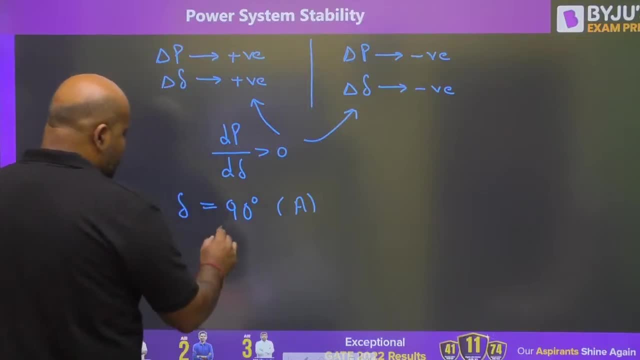 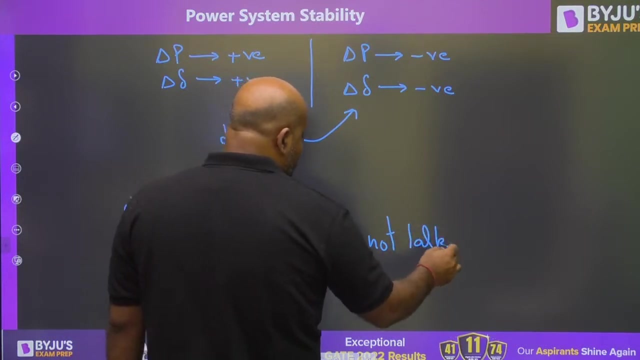 Now, when the slope is zero, When the system is marginally stable, what is the conclusion statement you can give? Cannot talk about stability. What is the meaning of this? Because if you are operating your system at del is equal to 90 degree. 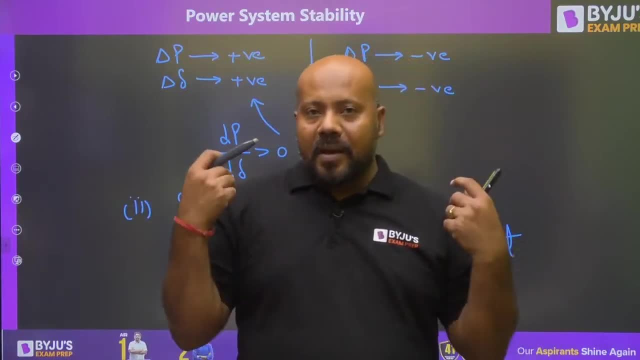 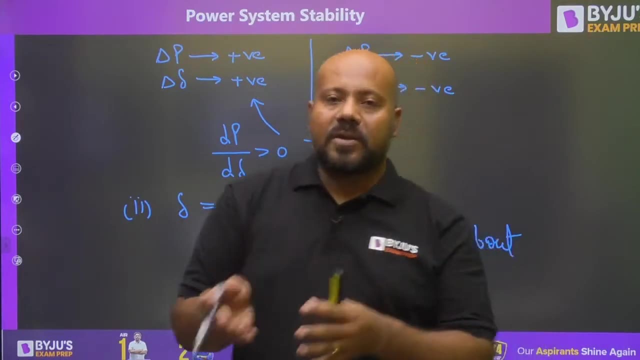 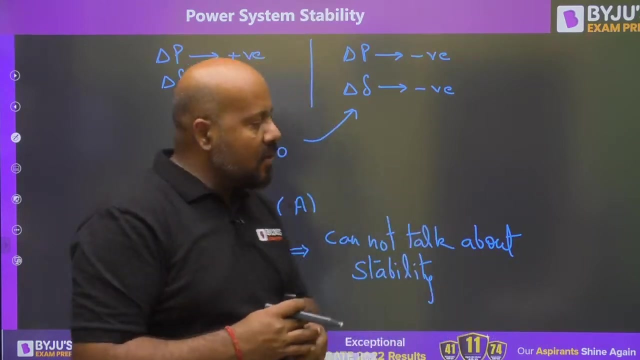 That is at the marginally stable point, then you can never know whether the system the next time, the next moment the system is going to be stable or unstable. You cannot predict anything, You cannot say anything, You are not sure about it. So we are saying: 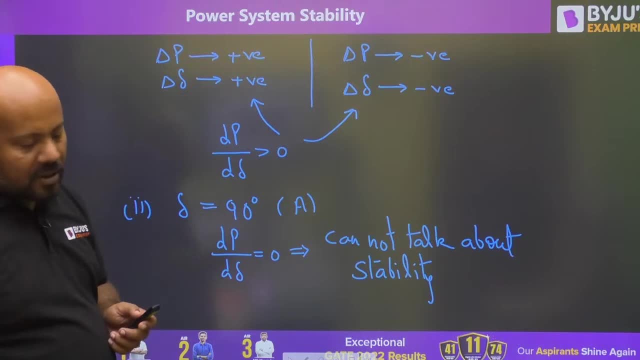 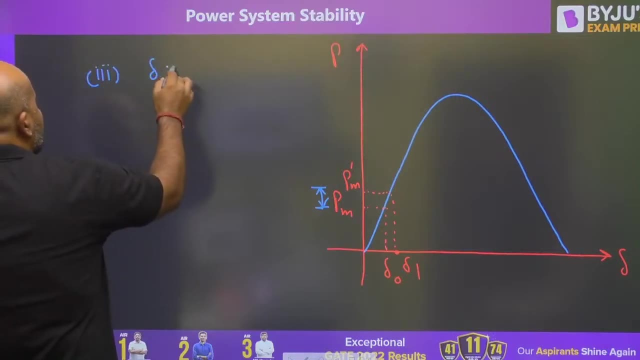 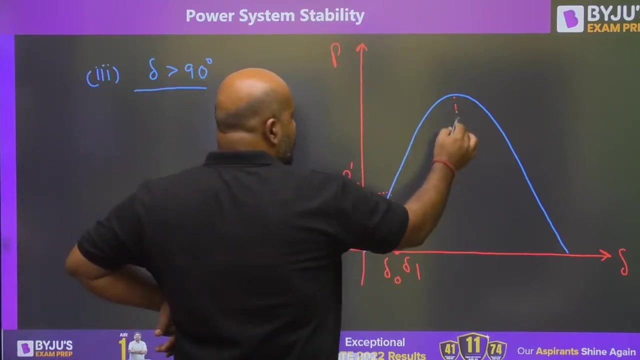 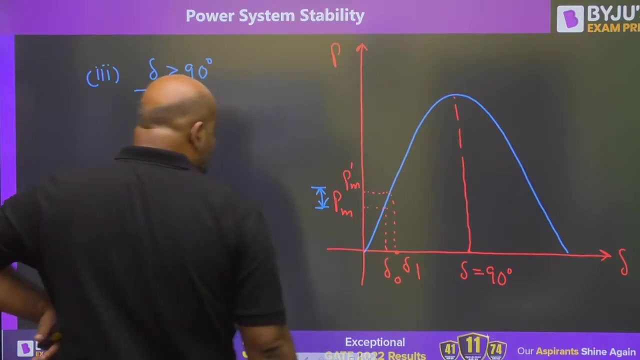 cannot talk about stability. Is it clear? Everybody, just tell me in the comment section. The third part is when del is more than 90 degree, When del is more than 90 degree, When del is more than 90 degree- See in this diagram: Del more than 90 degree. What does it mean? 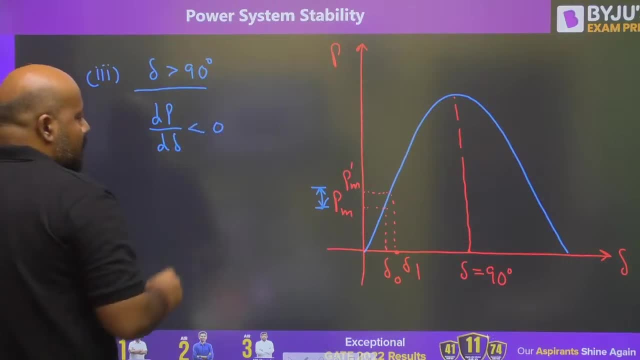 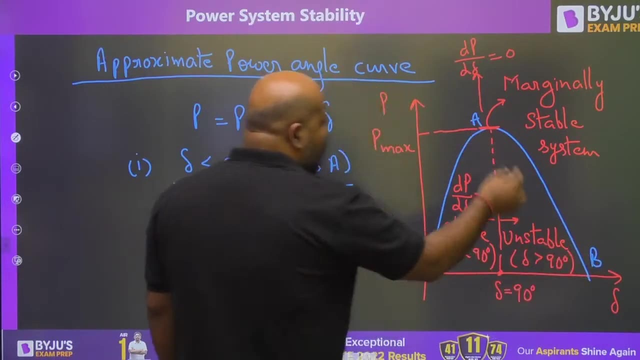 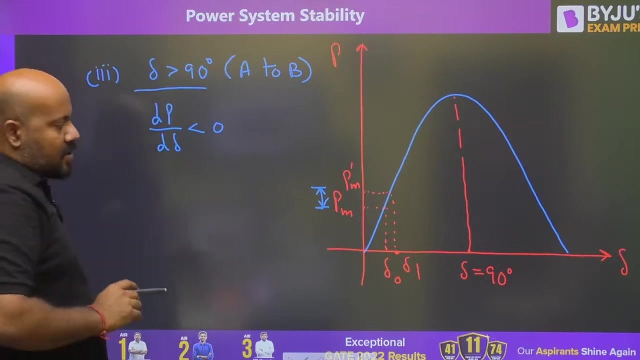 The slope of the curve is going to be less than zero, It is going to have the negative slope. from where to where, If this point is A and this point is B? So from A to B, we are saying the slope is negative, So it is going to be unstable. Now let us try to. 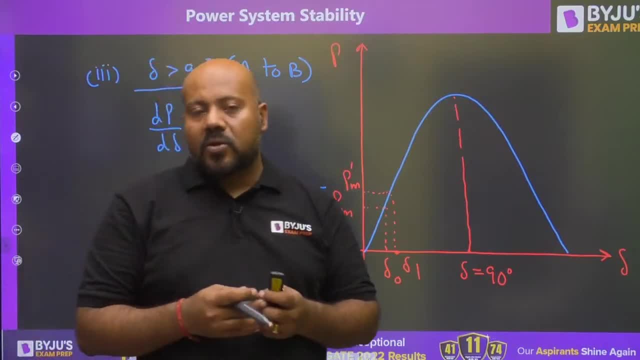 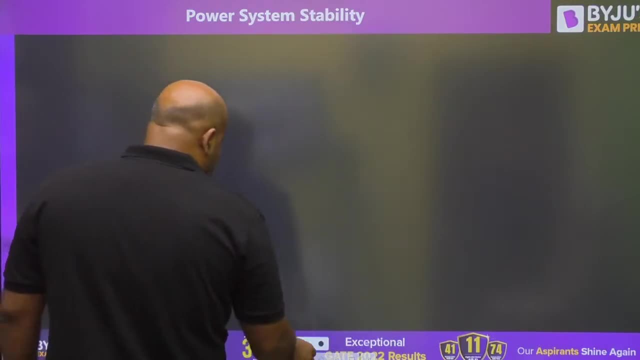 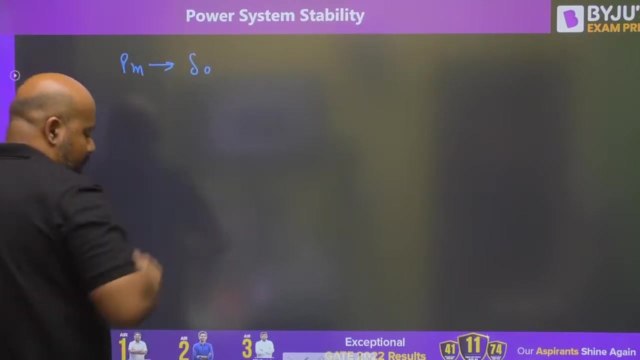 understand how we are able to relate this slope, How we are able to relate this slope with the stability. Now please try to understand. Suppose you are generating Pm power at del. not. You are generating Pm power. real power at del is equal to del not. 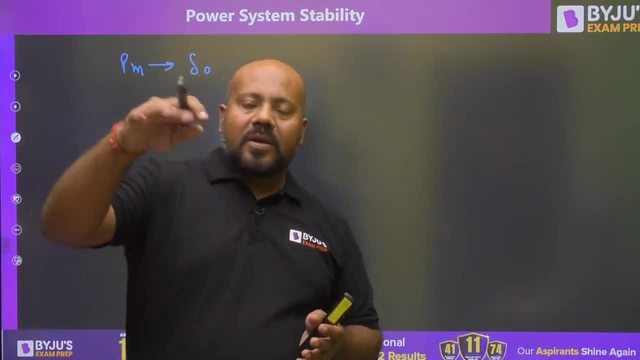 Now because of any particular disturbance in the system, Suppose new load is connected. Now you have to generate more, Yes or no? This is what we call as disturbance. Any change is disturbance for the system, Suppose a new load is connected. So if new load is, 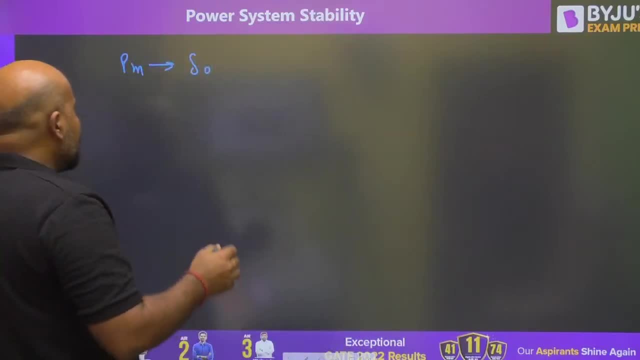 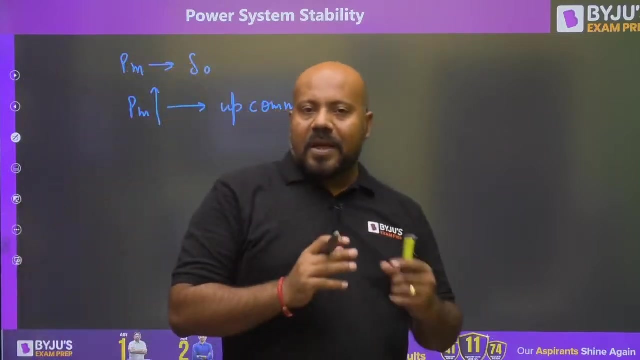 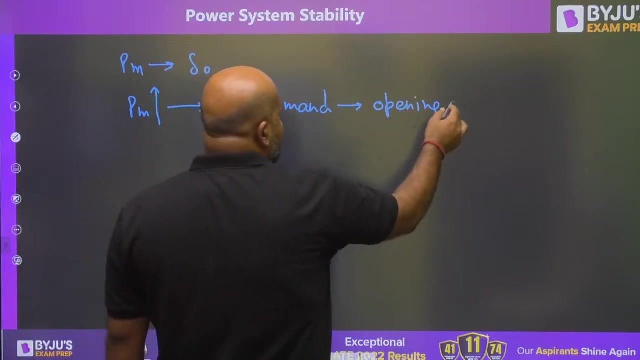 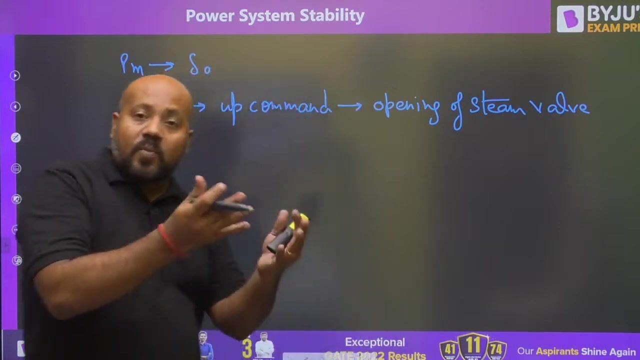 connected. it means you have to generate more. The moment Pm is increased, the load is increased. So an up command will be given. If you understand what is this up command, this up command simply means that opening of a steam valve. Opening of steam valve, means more steam is going to come. How power is? 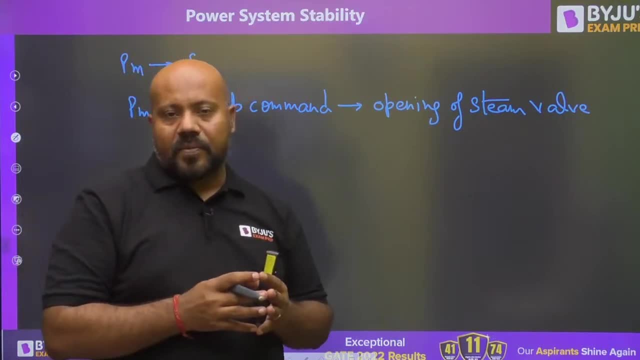 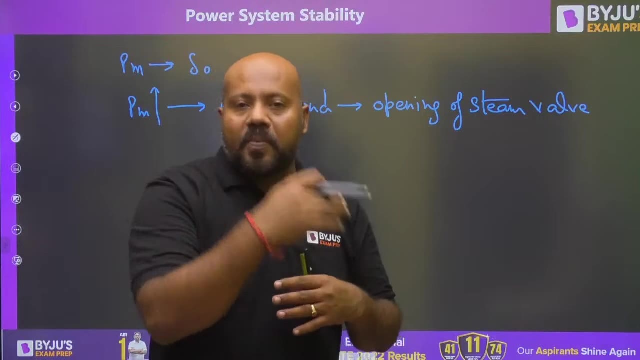 generated. High pressure, high temperature, steam is focused on the blades of the turbine. Turbine rotates, Electricity is generated. If you want more power in the system or you to be generated, then you have to increase the steam so that the turbine blades rotate at a 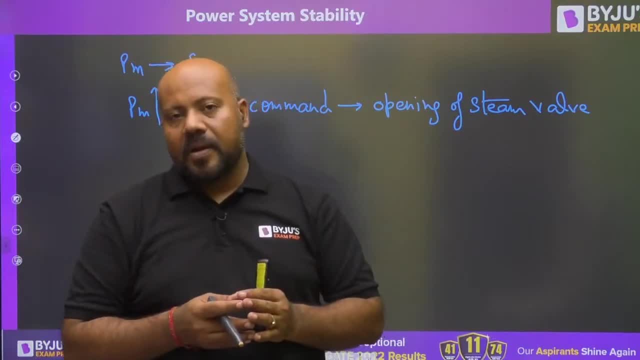 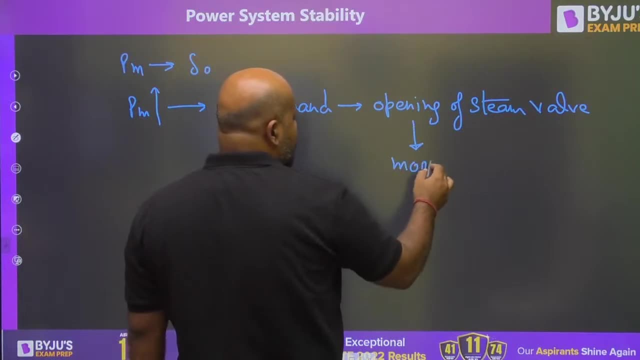 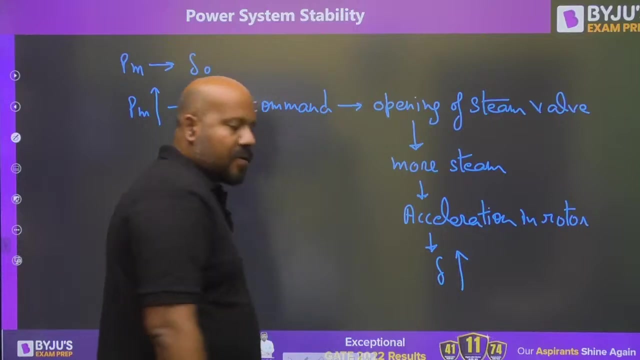 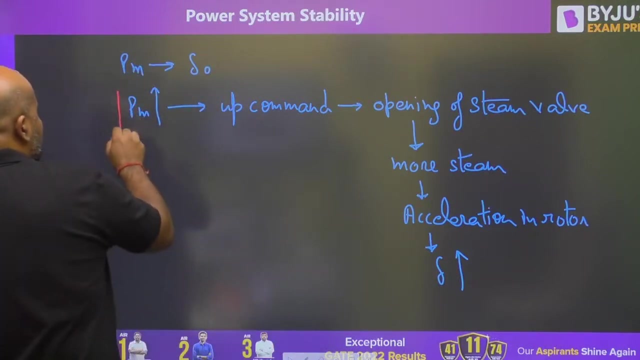 faster speed, more electrical power is generated. so when more opening of the steam wall happens, more steam comes, more steam comes. so there is acceleration in the rotor. acceleration in the rotor means what del angle is increased and it is vice versa. it is vice versa if this power is. 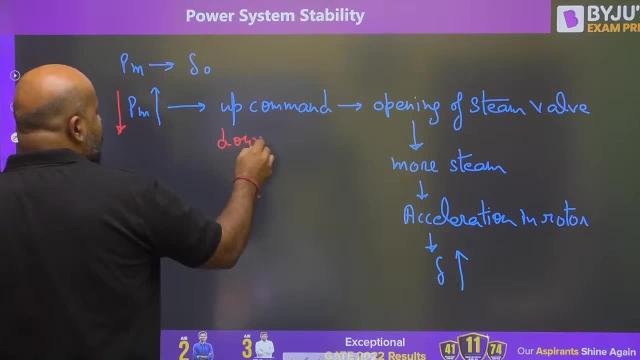 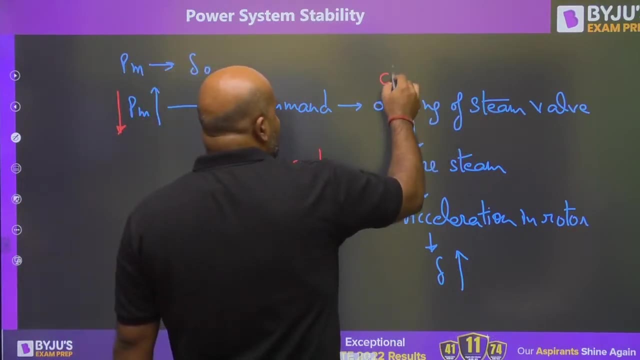 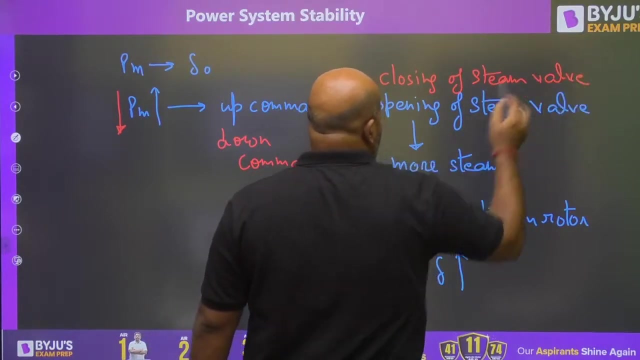 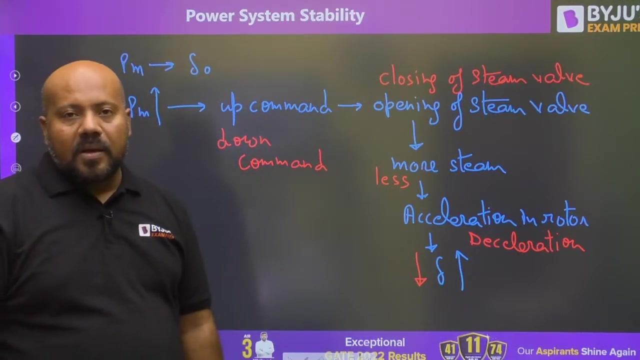 reduced. instead of up command, down command is given. instead of opening of a steam ball, closing of a steam wall, more steam instead of that, less steam. acceleration. it becomes the acceleration and instead of increasing del, the del is reduced, vice versa. now you can observe the very important relation here. 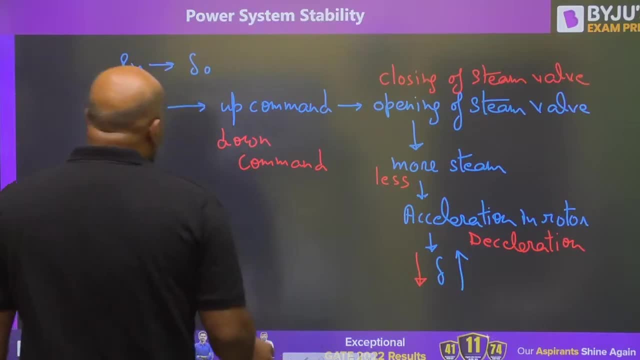 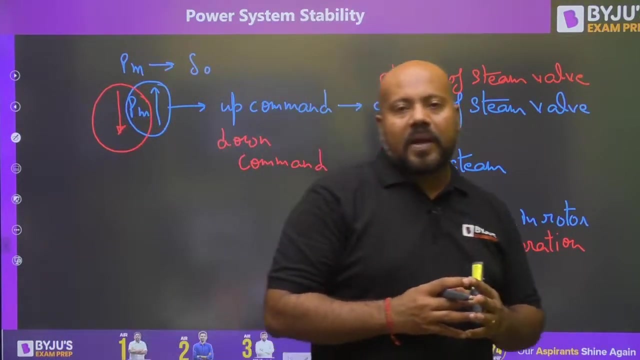 between P and L. when P is increasing, del is also increasing. when P is reducing, del is also reducing. and that is why we are saying: when the slope of the power angle curve is positive, the system is stable. when the slope of the power angle curve is negative, the system 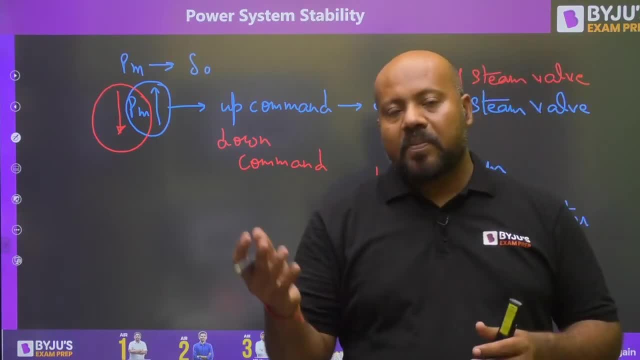 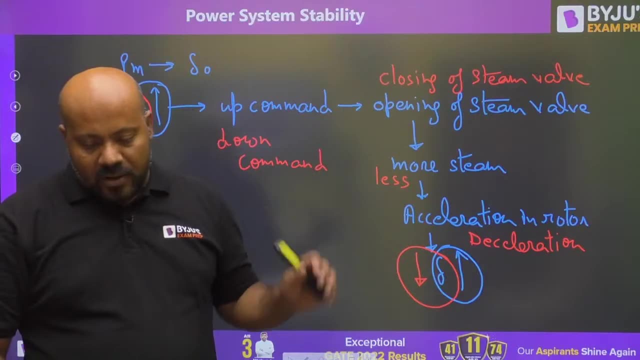 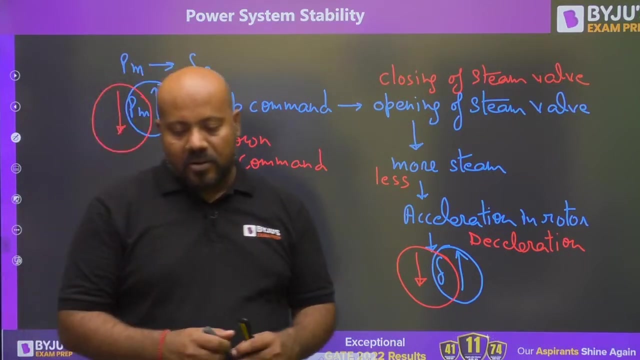 is unstable and when the slope of the power angle curve at the peak P max situation is zero, then the system is marginally stable. so this is what I wanted you to understand. in case of steady state stability, everybody just tell me in the comment section are you able to follow this or not. 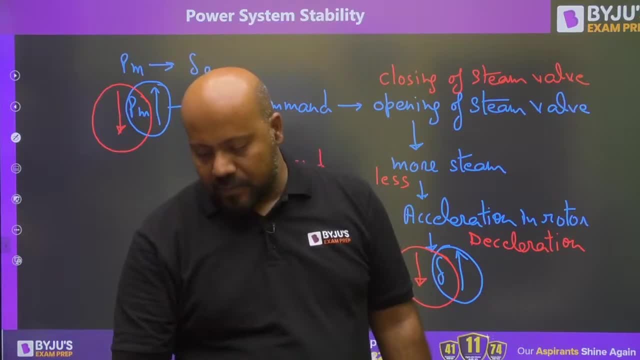 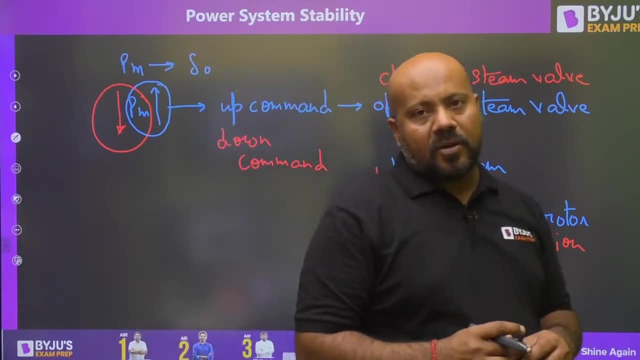 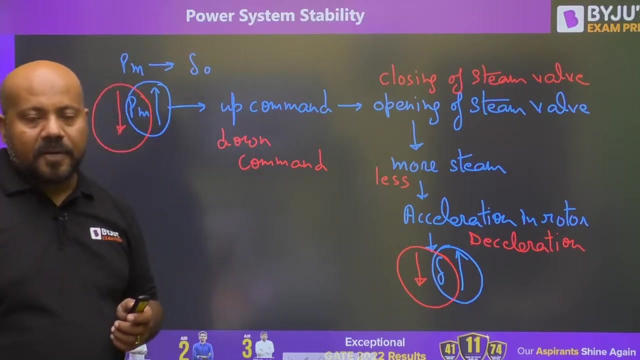 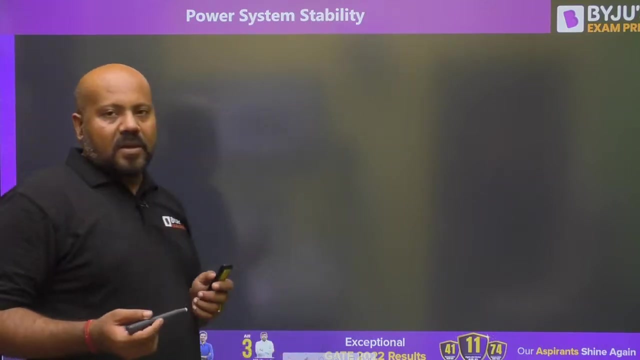 yes, everyone, everybody. just tell me in the comment section: are you able to follow this or not? if you are live with me, do not forget to comment, then only I can understand whether you are able to follow me or not, and if you have any query, you are most welcome now. what we have discussed right now is: 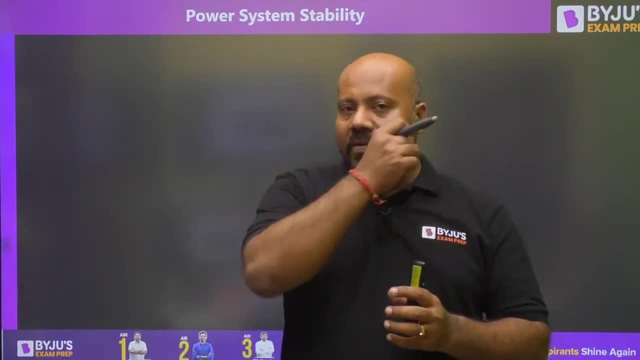 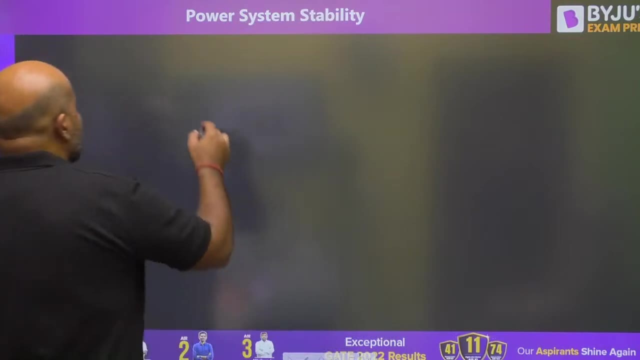 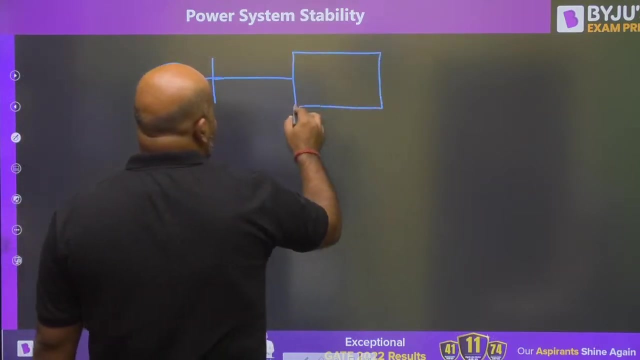 actually the approximate power angle curve. but we want to know the approximate power angle curve to have a general understanding of the stability. so, for that purpose, what we are going to do, we are going to take a more general example. this is a generator. suppose this is a transmission line. 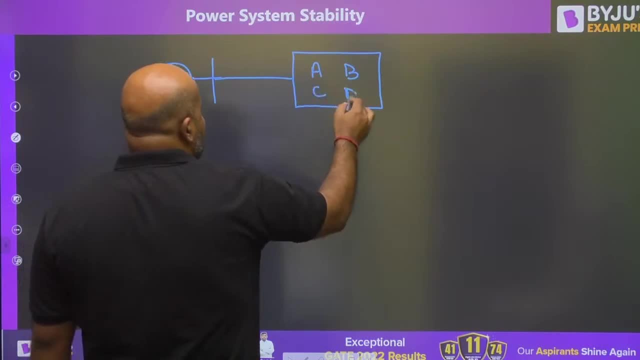 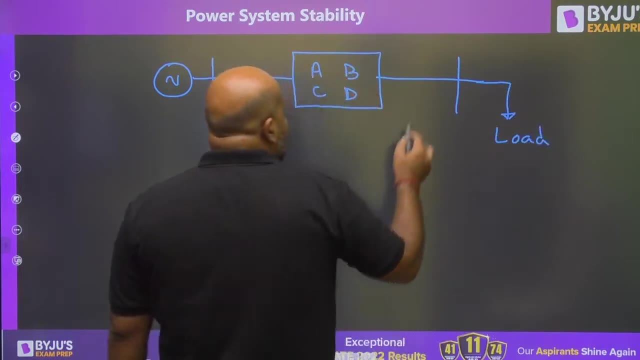 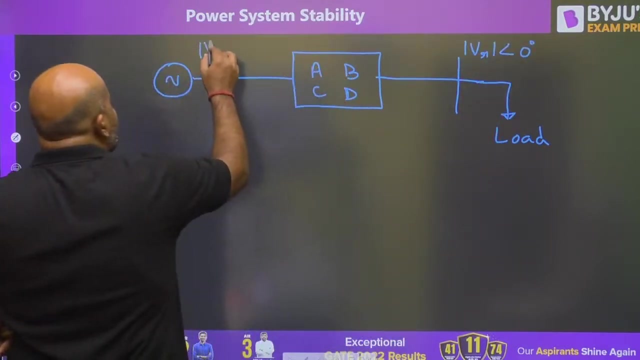 having ABCD parameters like ABCD, and this is the receiving end and this is your load again, the receiving end voltage is: we are angle zero, the sending and voltages vs angle del. the real and reactive power sent from the generator is PS j, QS and the. 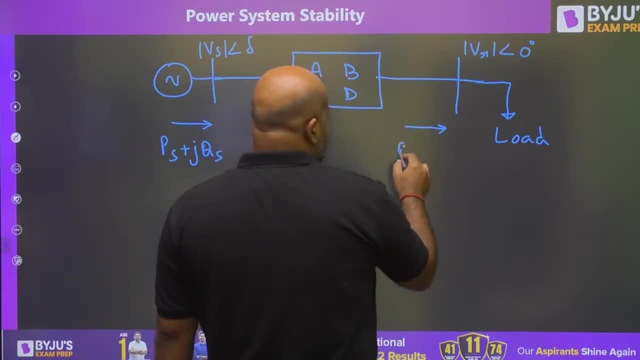 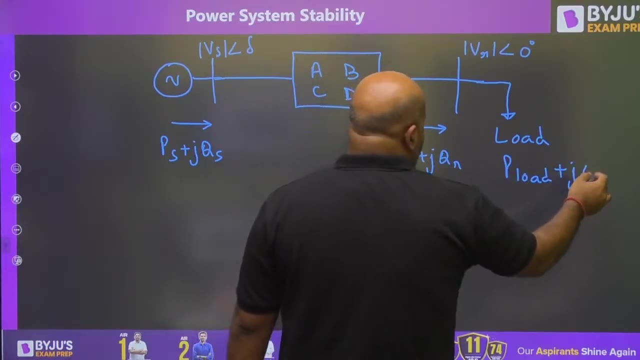 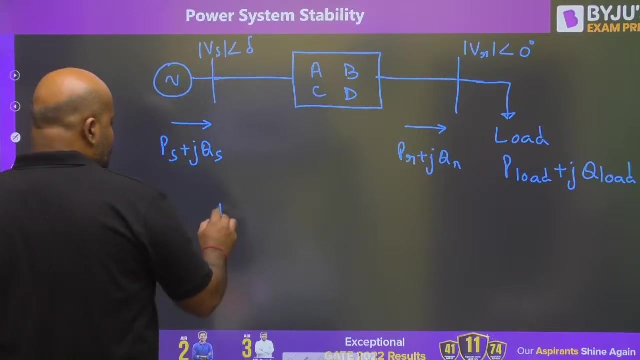 real and reactive power received is PR plus J q are in the load. real and reactive power demand is p load plus jq load. now please try to understand this. a parameter we are defining as mod A angle, alpha B parameter we are defining as mod B angle beta. 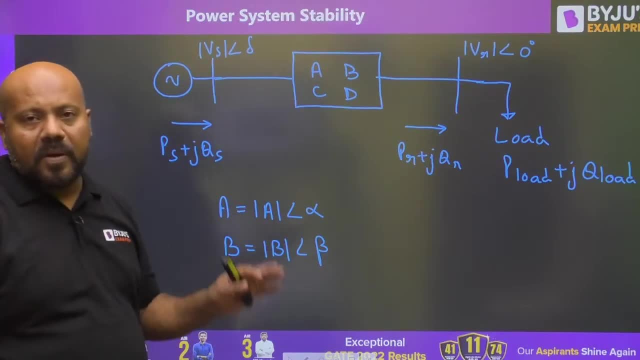 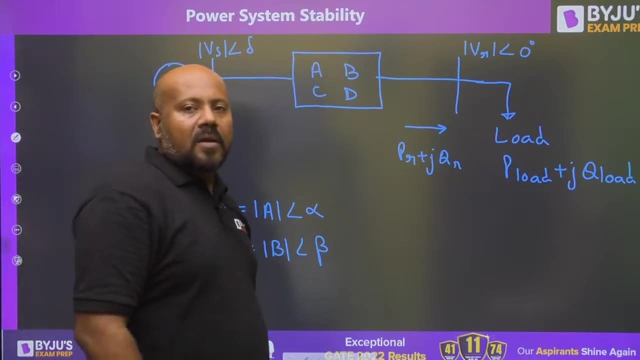 We are interested in A and B. only If you know the derivation part then you will be able to follow it. Otherwise you can see the derivation part. It is given in the book also. That is the steady state power transfer equations for the transmission line. Is it clear? 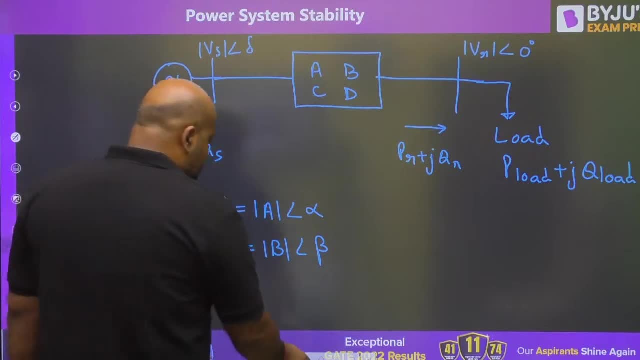 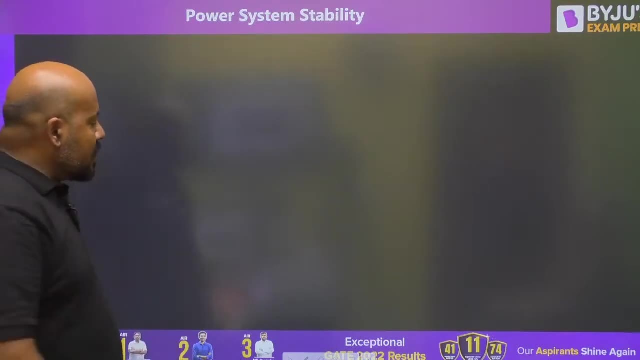 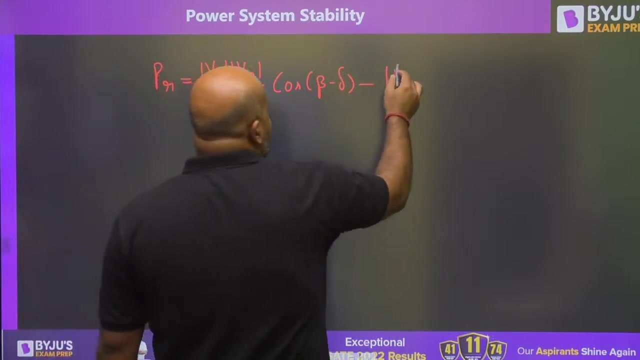 Now, if I want to analyze the stability, I want to focus on which parameter? I want to focus on the real power received. Now, what is the expression for the real power received? It is given as: mod Vs- mod Vr upon mod B. cos, beta minus del. minus mod A upon mod B- mod Vr- square. 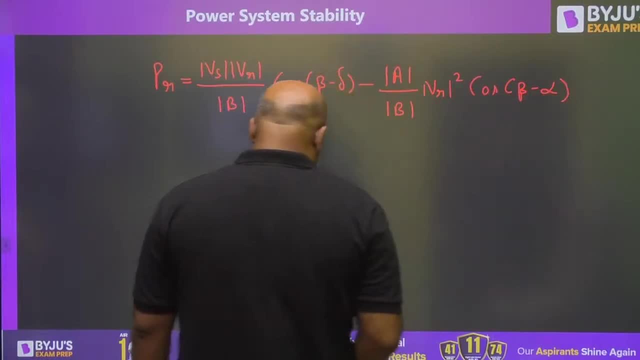 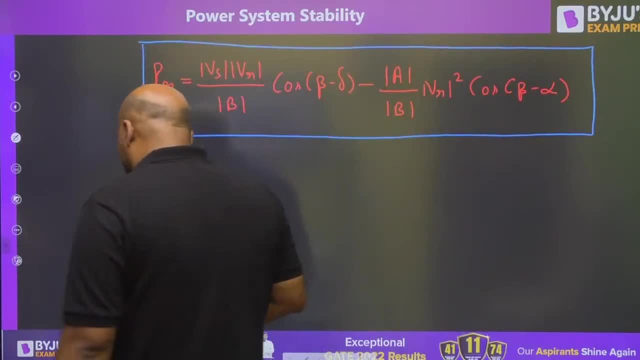 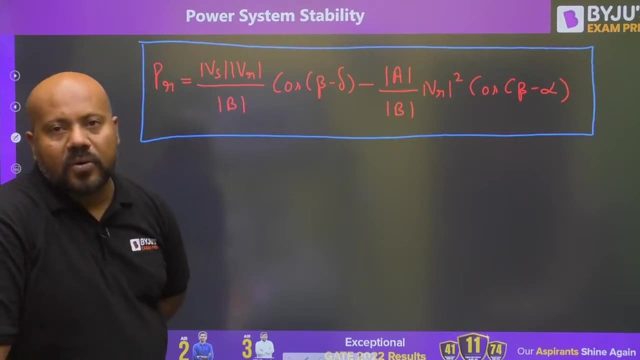 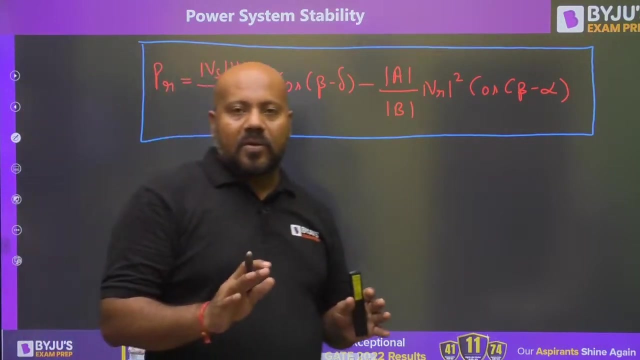 Now this is the equation. if you see the previous year gate questions, almost every alternate year you are going to get a question on this particular equation. So if you do not know about this equation, you please read it from some book and remember it. this is going to give you lot of help. 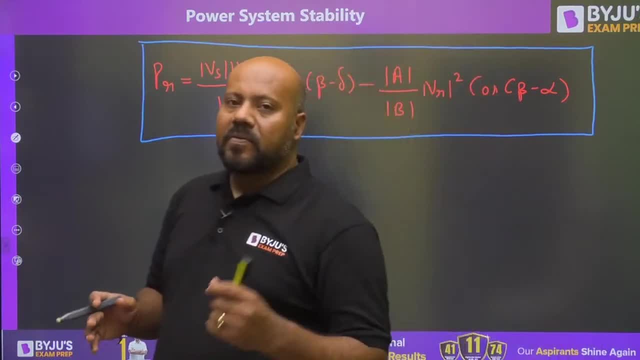 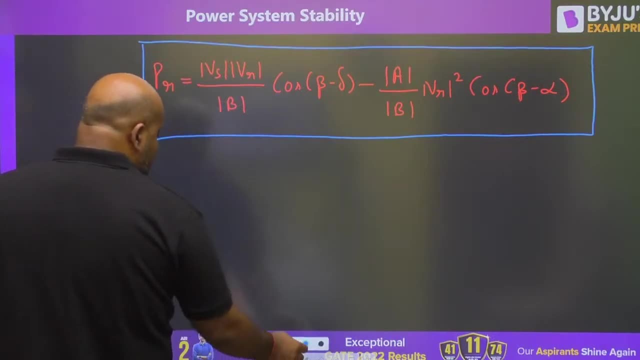 in your examination. In lot many places in power system we used to use this particular equation. Now again, if you want to know what is the condition for PR to be PRmax, which we are calling as steady state stability limit, Is it clear, everybody? 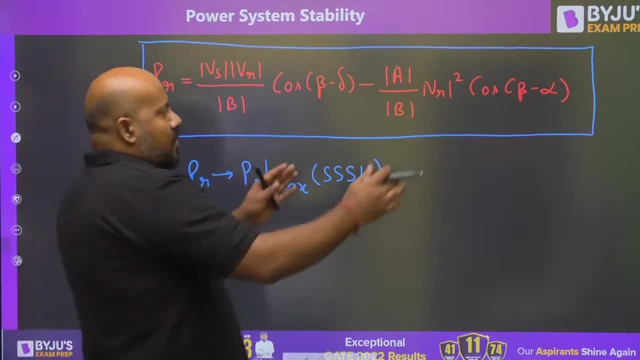 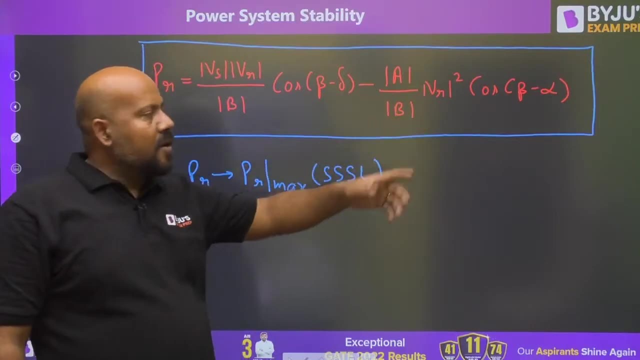 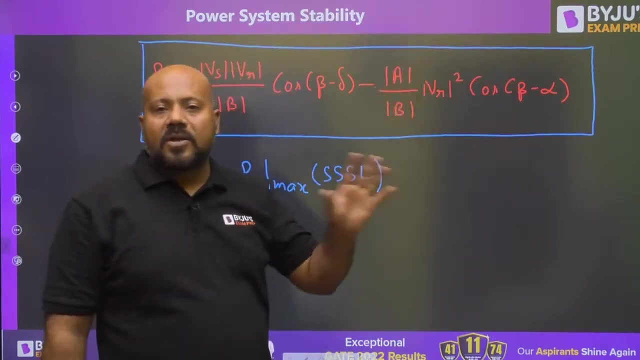 What is that condition? Now, if you see this particular term- mod A, mod B, both are ABCD parameters, mod VR, square- we are not changing beta angle of B, alpha angle of A. it means this particular term is not going to have any variation, it is going to be constant. 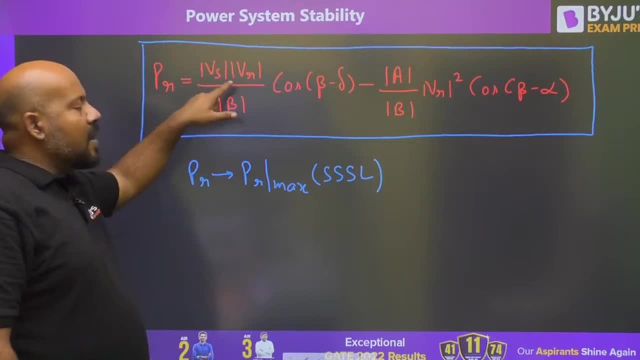 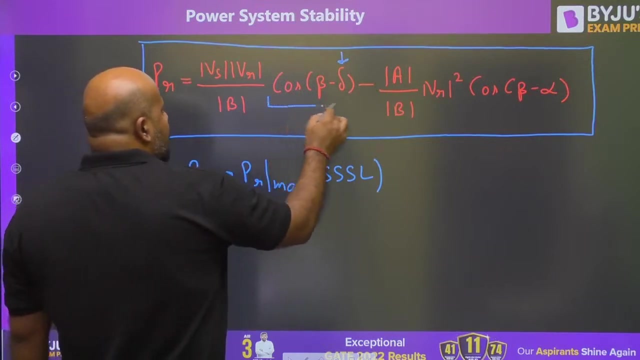 First term can be varied. where it can be varied. VS VR magnitude, we are not changing B is the ABCD parameter constant. we cannot change it. Cos beta minus del beta is also constant, but del can be changed. del is the variable. So the maximum condition will be given when this cos beta minus del is going to be 1, when 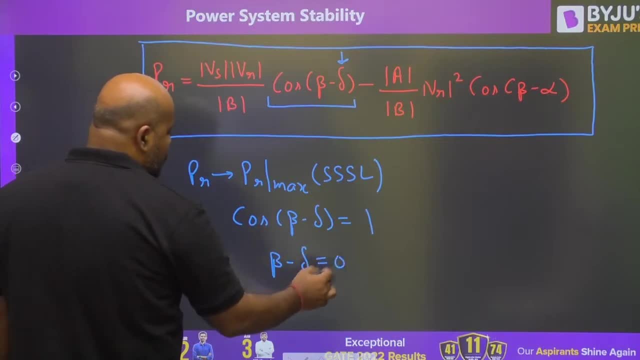 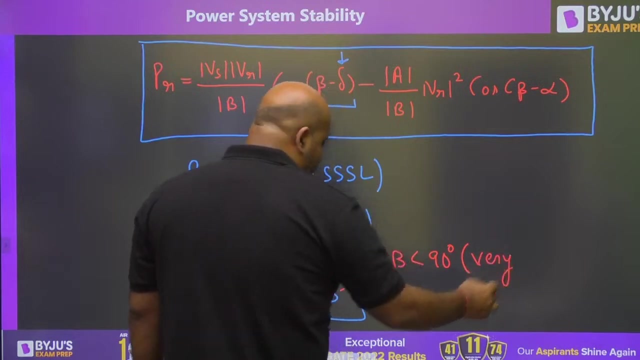 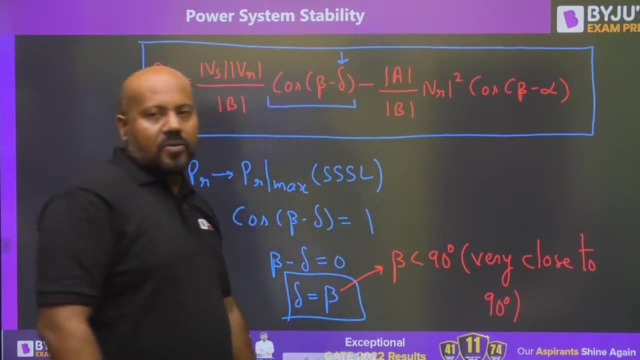 it can be 1 when beta minus del is 0, or you can say del is equal to beta. And let me tell you in general, for most of the practical cases, beta is less than delta, It is less than 90 degree and it is generally very close to 90 degree, very close to 90. 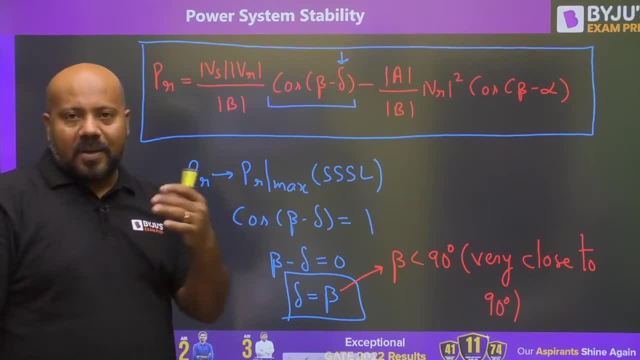 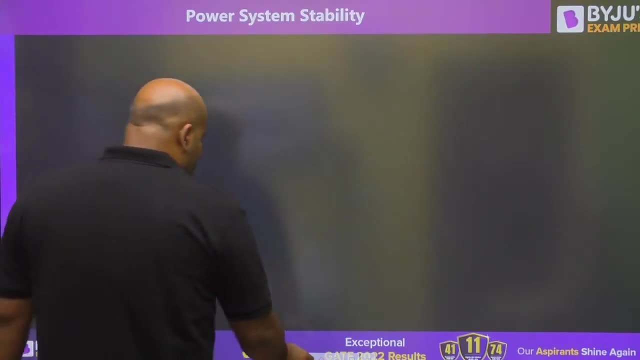 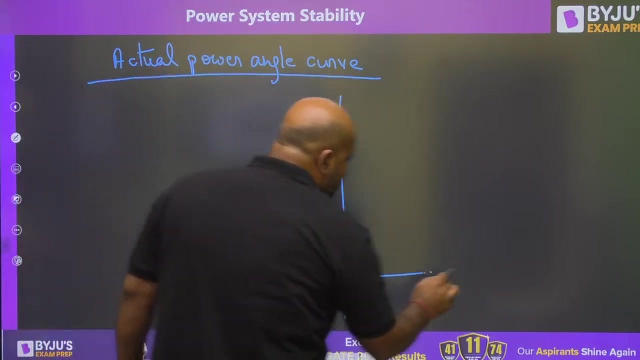 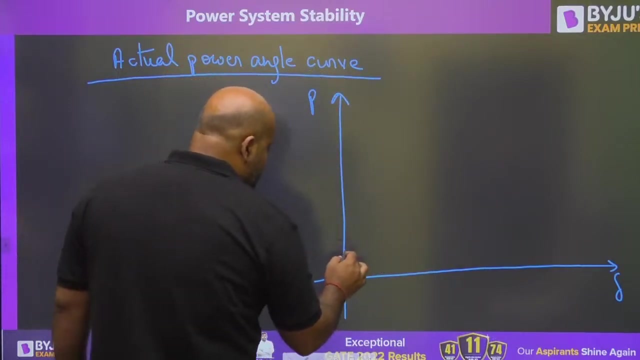 degree. So if you want to know the stability steady state stability analysis accurately, then you have to use this equation. Let us see the actual power angle curve: Actual power angle curve. Actual power angle curve is going to be something like this: It is going to start somewhere here and it is going to be something like this because 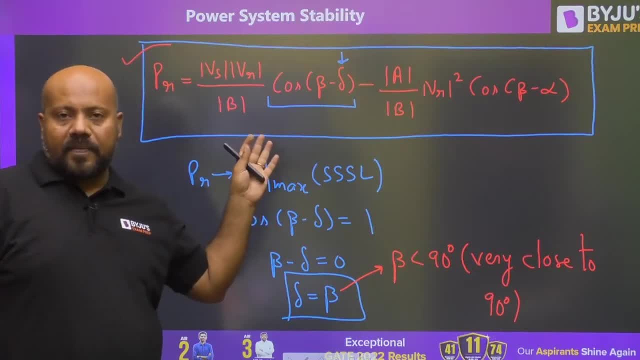 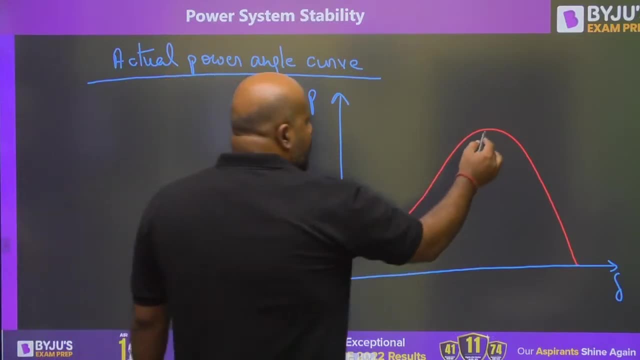 if you see, this equation is not a pure sinusoidal equation. It has little variation. so you are having this type of variation And the maximum power You are getting somewhere here. So You are getting somewhere here. that is, del is equal to beta, which is very near to 90. 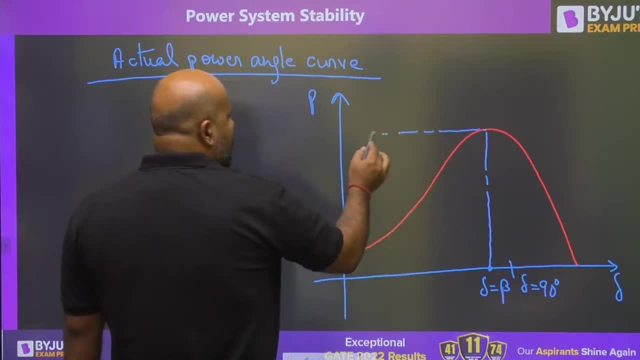 degree. It is less than 90 degree and this is what we are calling as P max situation. or you are saying it is steady state stability limit. Now you can see the regions of stability. You can see the regions of stability. I think people are not interested in stability. 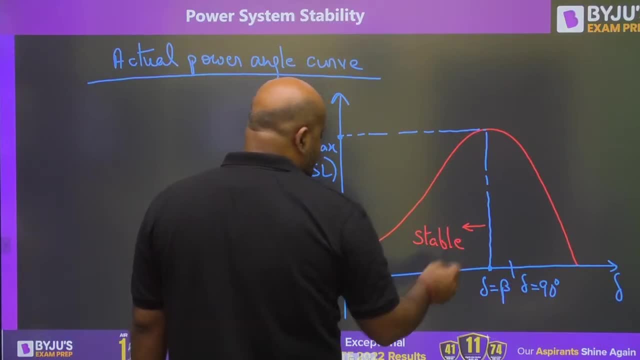 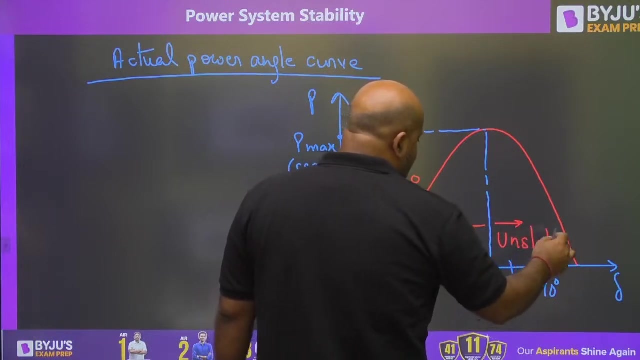 So this is a stable region. Why it is a stable region? Because the slope of the curve, dp by d del, is positive, greater than 0.. This region is unstable region. Why it is unstable region? Because dp by d del is greater than 0.. 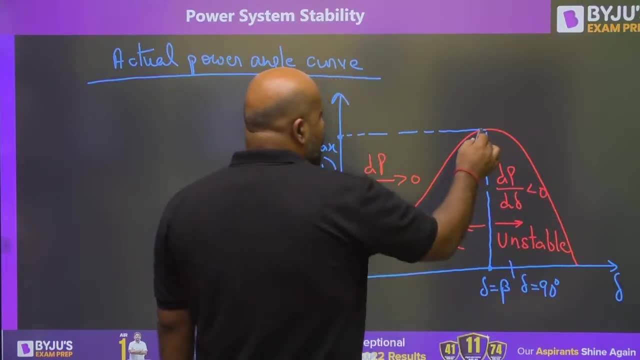 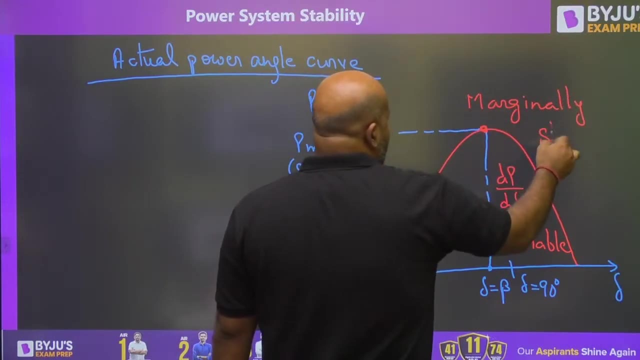 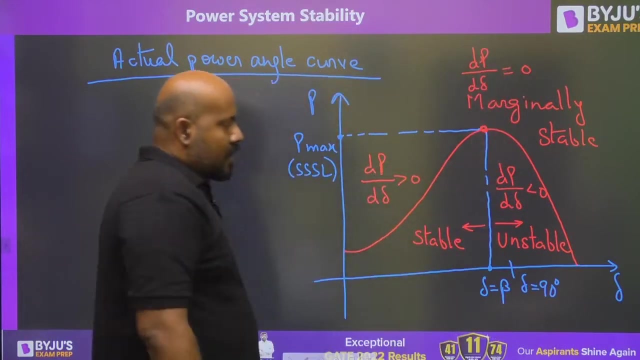 Why it is unstable region? Because dp by d del is greater than 0.. Why it is unstable region? Because dp by d del is less than 0. Why it is unstable region? Because dp by d del is less than 0. 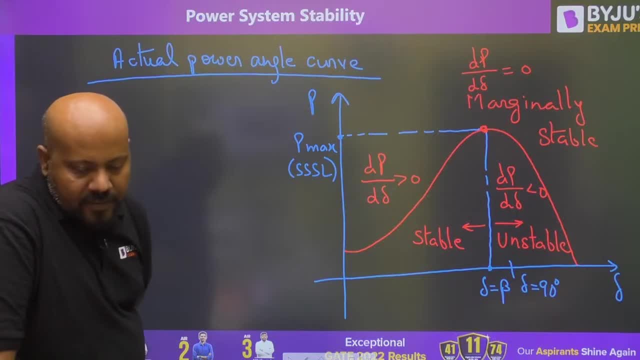 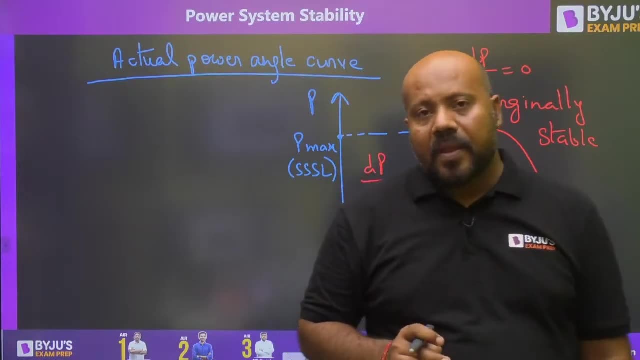 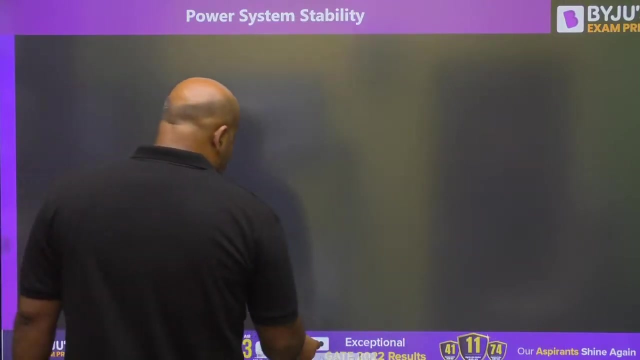 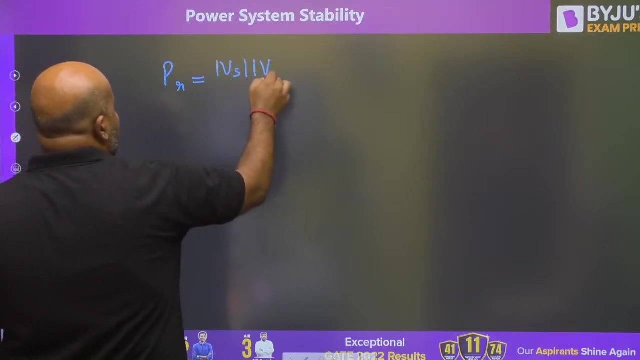 Why it is unstable region, Because dp by d del is greater than 0 And this point is marginally stable, Marginally stable Where? Let me just give you one more concept which can be asked in your examination: Suppose we are writing the power angle equation for PR as mod VS mod VR upon mod B and this: 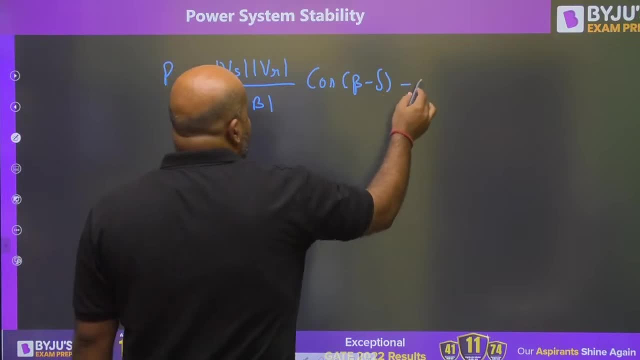 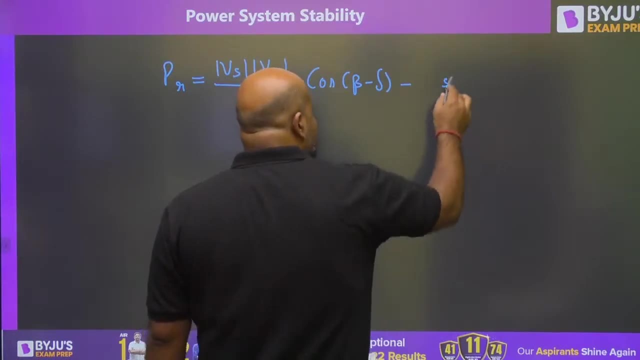 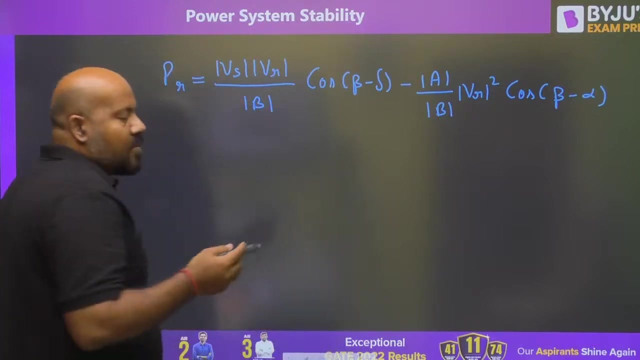 is cos beta minus del minus. and this is mod VS, sorry, mod A upon mod B, mod VR: square cos beta minus alpha. Now let us take some of the approximations. What are the approximations? We are taking? A, We are taking short transmission line approximation. 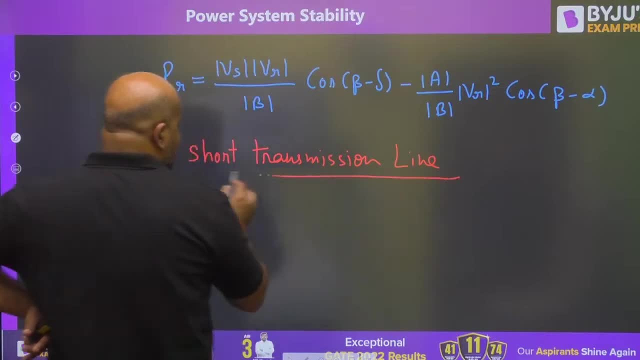 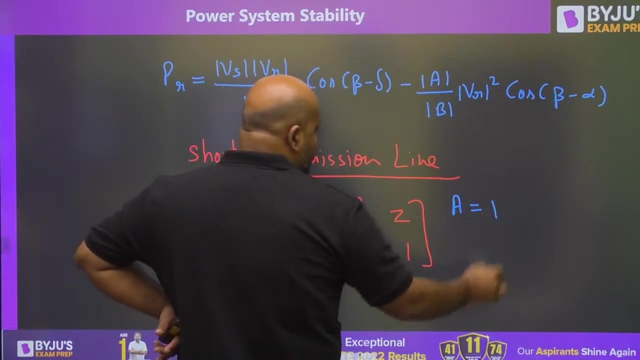 Now for the short transmission line. can you tell me what are the ABCD parameter? The ABCD parameters are going to be 1, Z, 0,, 1.. What is going to be A parameter value? A parameter is going to be 1.. 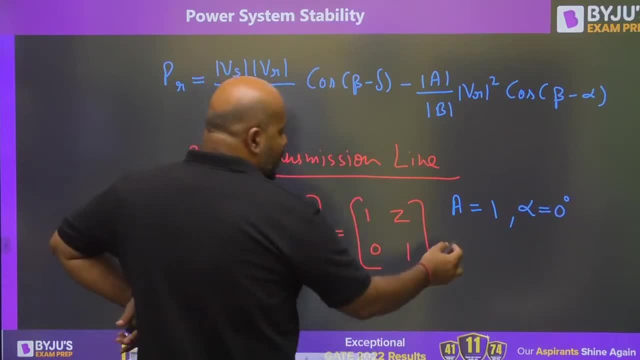 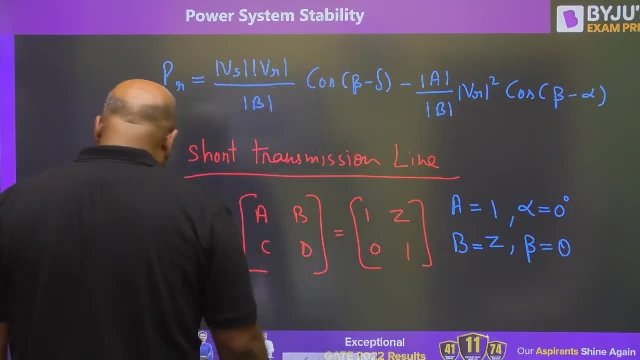 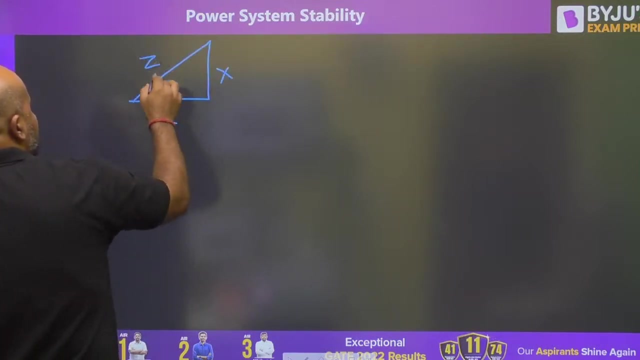 Angle of A is going to be 0., B is going to be what Z? And beta angle is going to be what? Theta Now? what is theta? What is theta? If this is R, this is X, this is Z. this is theta. 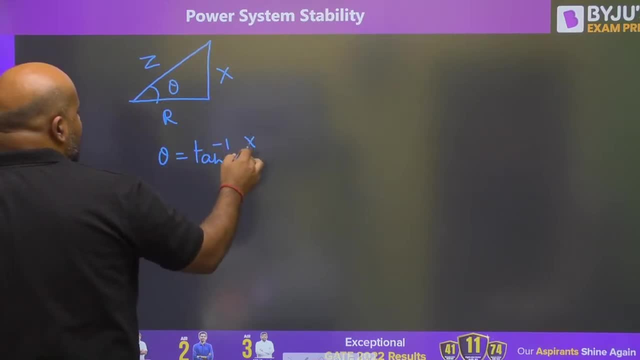 So how you are defining theta. Theta is tan inverse X by R, Is it clear everybody? Just tell me in the comment section: What is this R and X? This R and X are the. What is this R and X? What is this R and X? 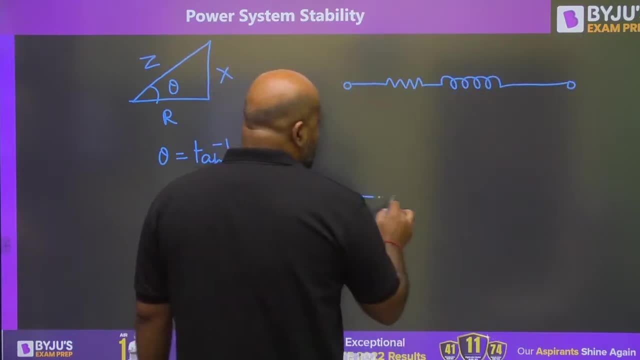 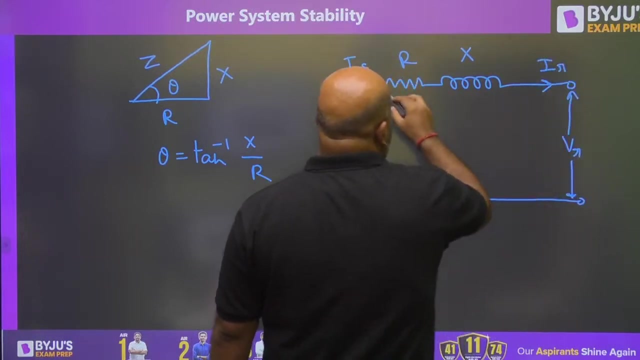 Is it Total series, lumped resistance and the inductive reactance of your short transmission line. This is your short transmission line approximation. I hope you understand it And this is what we are calling as Z. And this is what we are calling as Z. 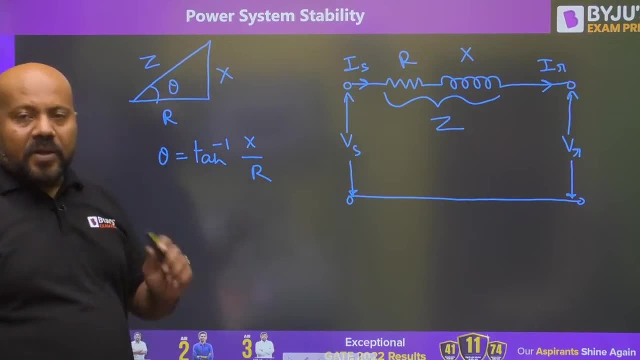 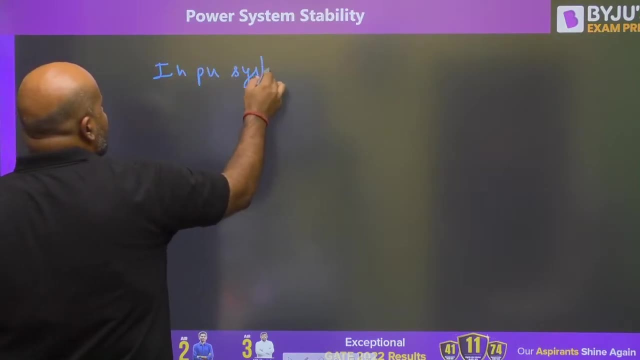 onset. This is S is equal to A. Now for the per unit system, or in general you can say in per unit system, or in general you can say: mod Vs and mod Vr are not going to be much different, They are going to be almost same. 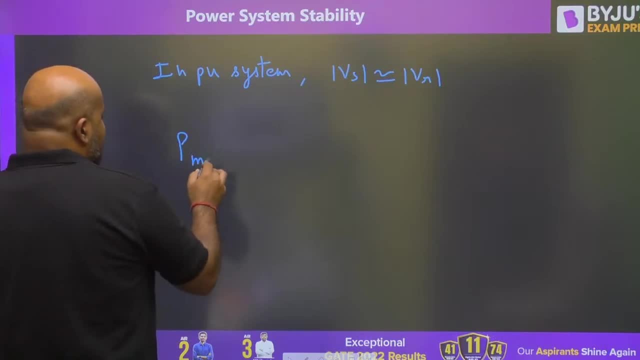 So if I write Pmax equation, what is going to be Pmax equation? Can you help me? So mod Vs, mod Vr, is going to be mod V, square Mod B I am going to write as mod Z, So this is simply going to be mod Z. 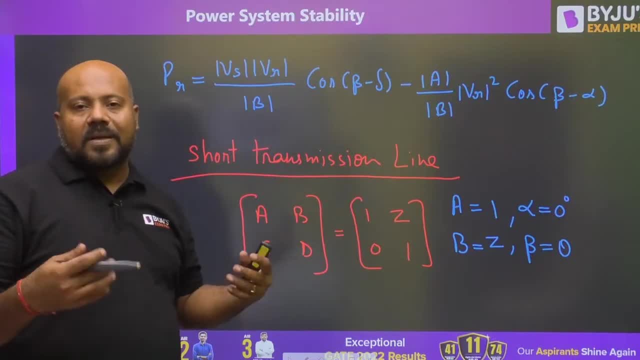 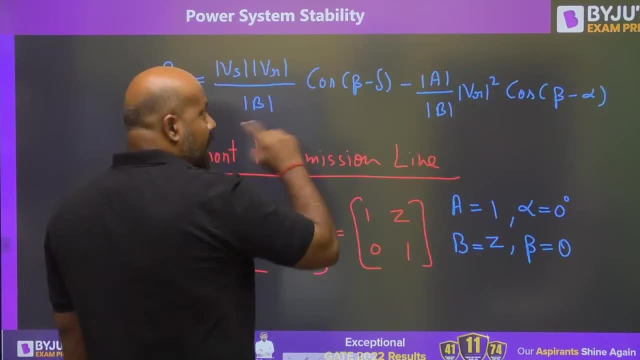 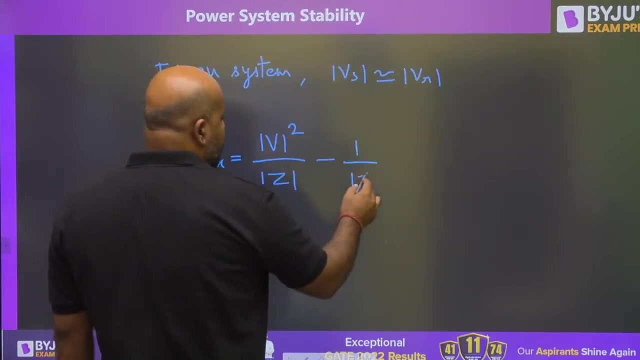 This cos beta minus del is going to be 1, because we are talking about the maximum real power received. So this is going to be 1 minus mod A is 1, mod A is 1.. Mod B Is mod Z And Vr square is simply V square. 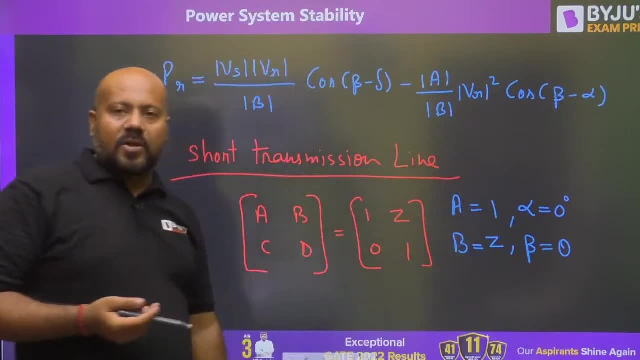 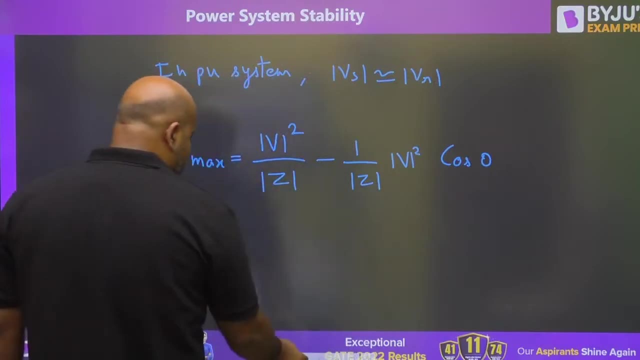 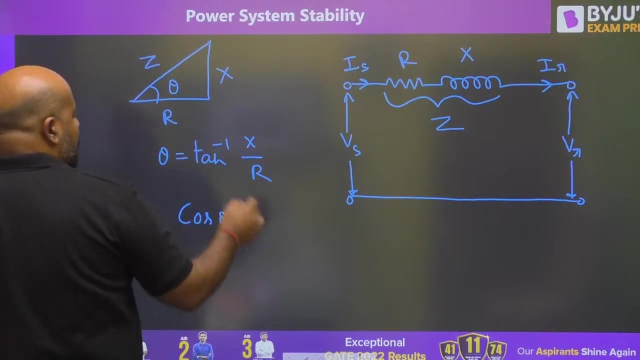 And then we have cos beta minus alpha. Now alpha is 0, and what is beta? Beta is theta. So we are writing cos theta, We are writing cos theta. Now, what is cos theta? Cos theta, you can write from here. Cos theta, you can write as R by Z. 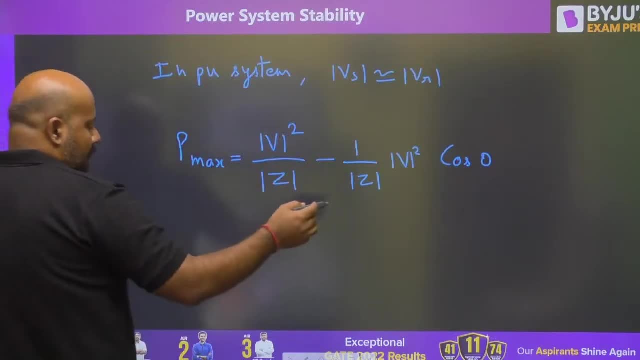 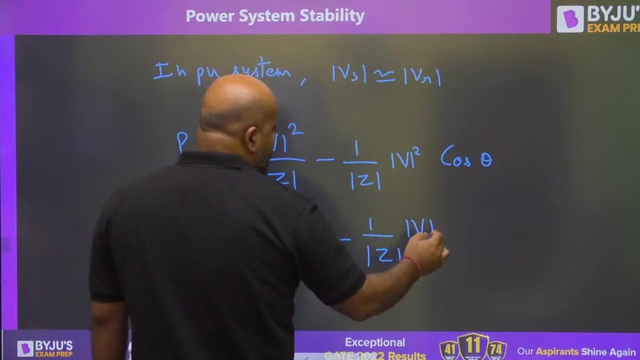 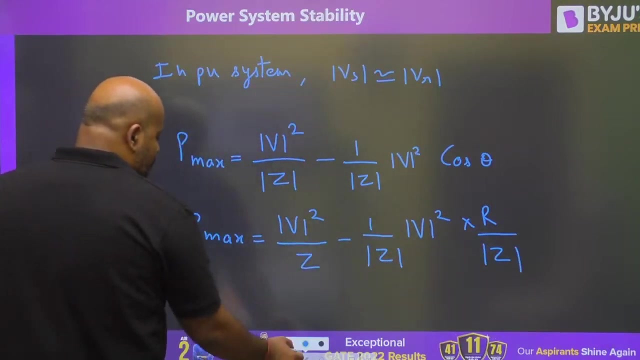 So you can write the value of theta here It is going to be: Pmax is equal to mod V square upon Z, minus 1 upon mod Z. mod V square and cos theta is R upon Z, That is mod Z. Now, if you see this equation, 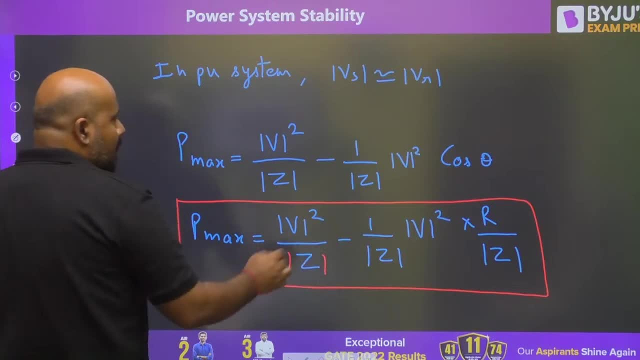 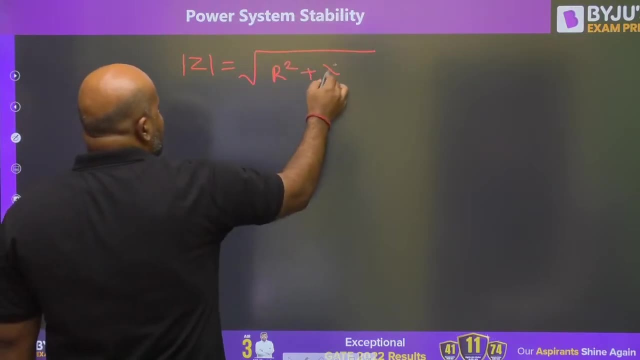 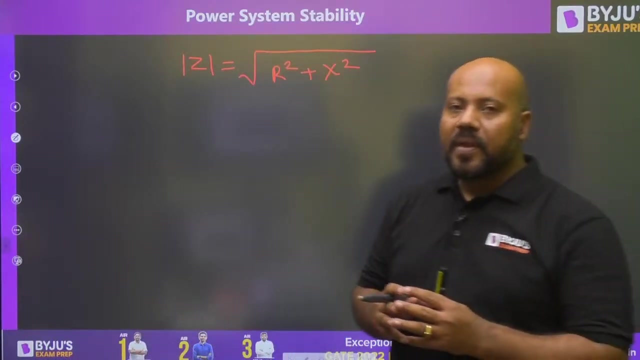 In this equation, This mod Z. how you can write mod Z. you can write as under root: R square plus X square, Yes or no. for the transmission line R and X, you can write mod Z as R square plus X square. Now, at the design level, when you are talking about the R and X, because R and X are the 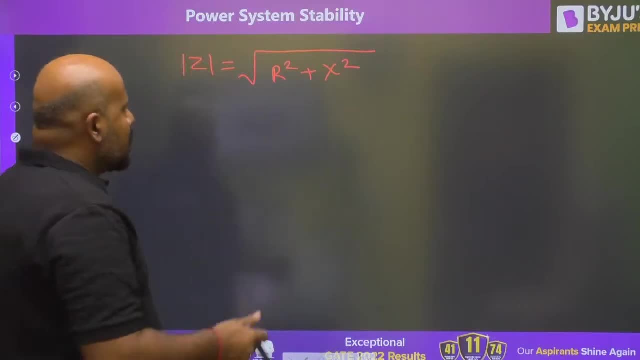 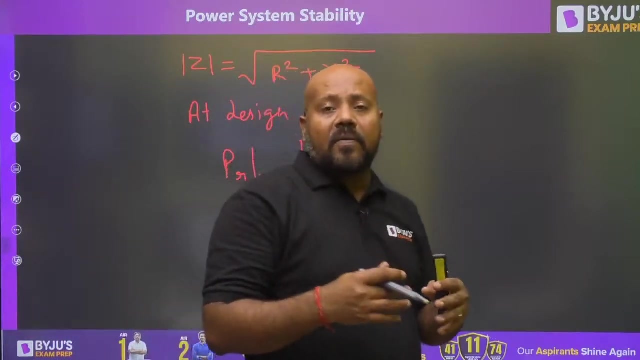 line parameters that you cannot change at the operating stage. So I want to know at the design stage, At the design stage I want to know the relation between R and X so that I can get P, R max maximum value, maximum value of the maximum real power received at the receiving end. 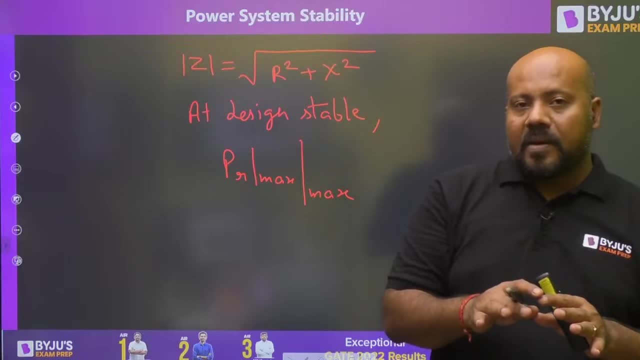 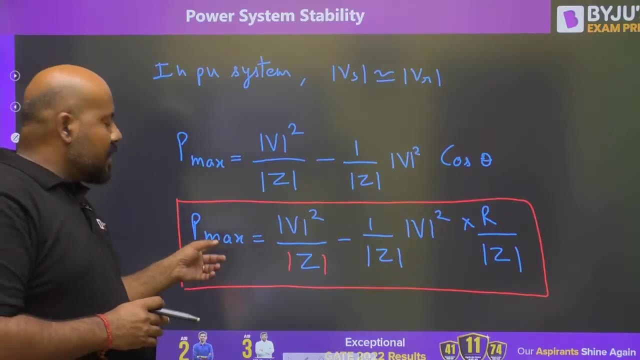 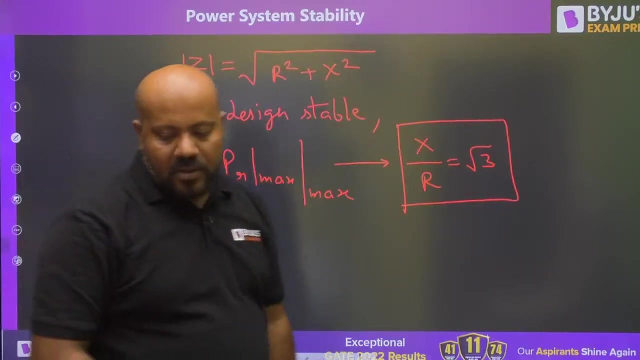 Again, I am trying to find the maximum value, of the maximum power by having some some condition at the design stage. So Now Differentiate this Pmax with respect to X, because we are making the variable X very popular question asked in various interviews. 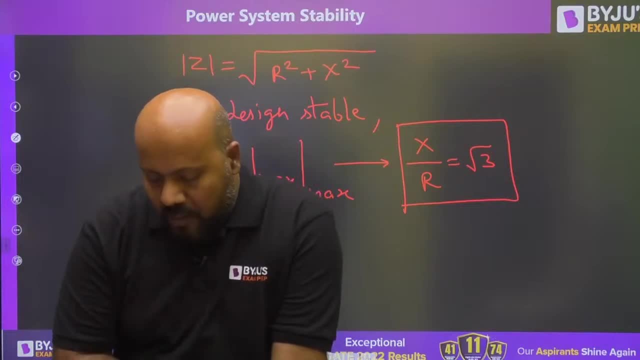 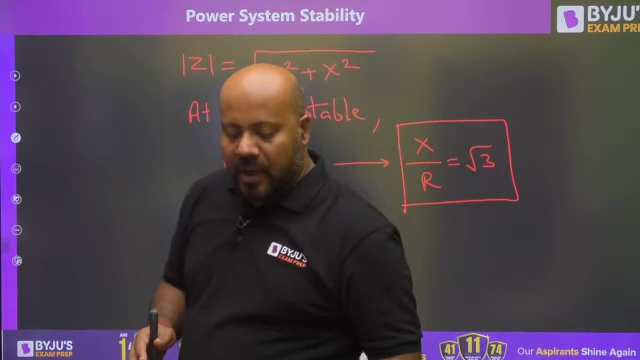 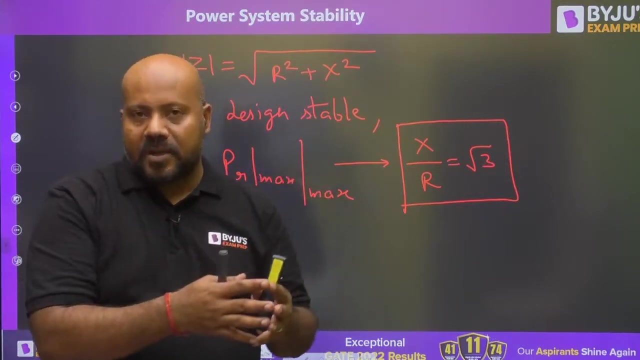 Everything is okay, my friend. Yes, very popular question asked in various interviews. What is the X by R ratio? the X by ratio? X by R ratio is generally taken as under root. 3. So That Pmax can be maximized. I hope you are getting this. 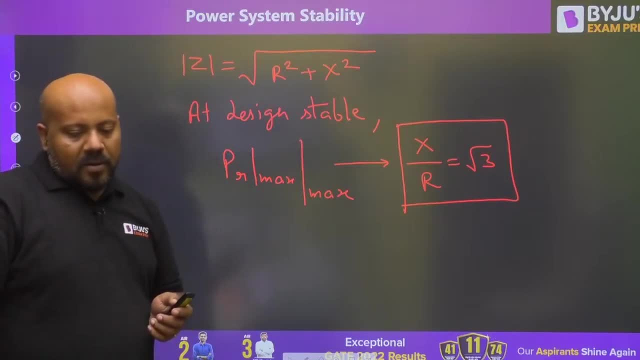 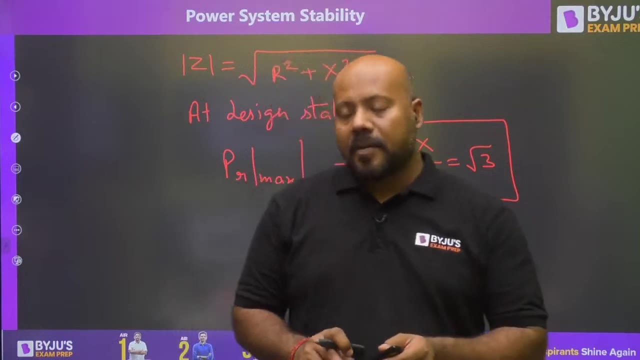 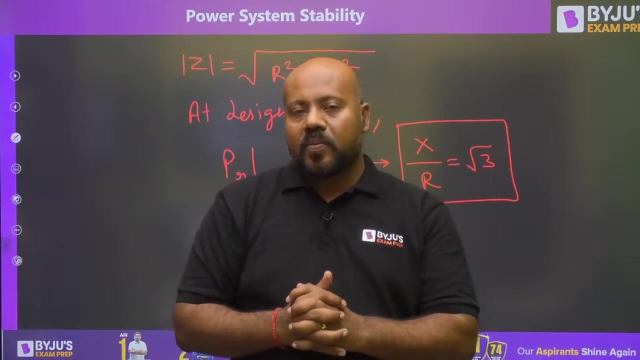 Is it clear? everybody, just tell me in the comment section. So let us stop here. This is what we have, what we wanted to discuss for the steady state stability. I also have to discuss transient stability, but in some other session, when I am going to practice some of the problems on stability, I will be giving you some brief idea with 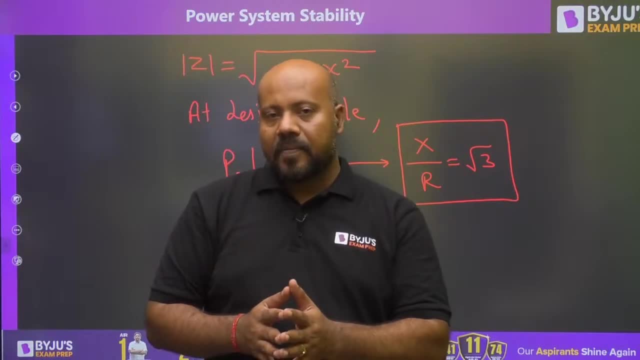 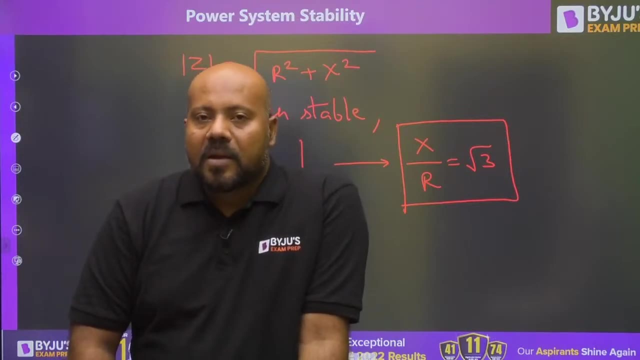 the help of the questions As far as transient stability is concerned. So thank you so much for joining me live in the discussion. It was a great time talking to you and I hope you are going to join me again in the next class tomorrow 8 pm in the evening, because tomorrow I am going to talk about some problem. 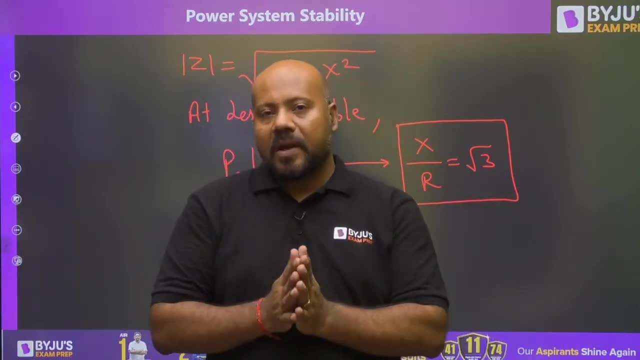 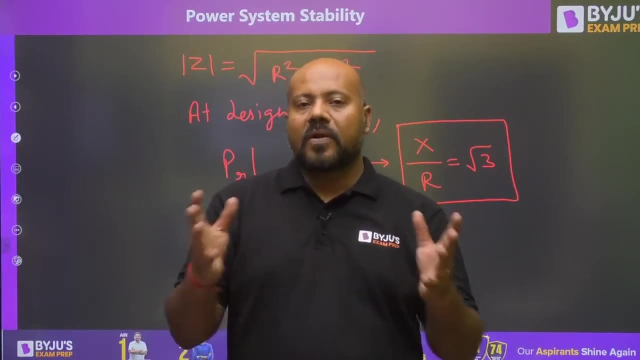 practices for the compensation compensation. some part we have discussed and some part we are going to discuss tomorrow, 8 pm in the evening on the same channel, Byju's exam prep. So do not forget to subscribe to Byju's exam prep. Stay connected.